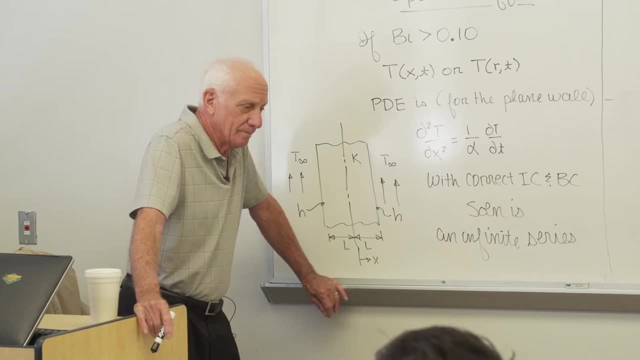 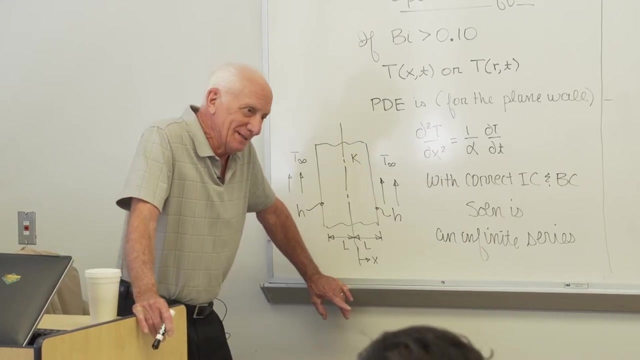 an object in conduction. heat transfer vary with time. There's only really two equations: One gives you the temperature as a function of time and the other one gives you the amount of energy transfer that occurred- capital Q. Now, the other side of the coin is: 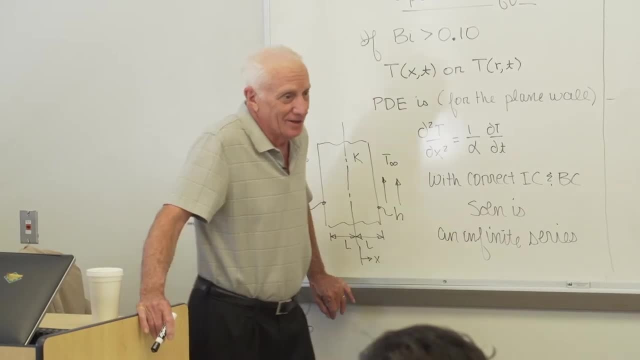 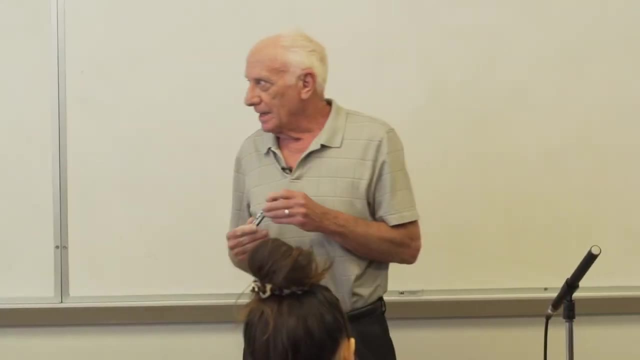 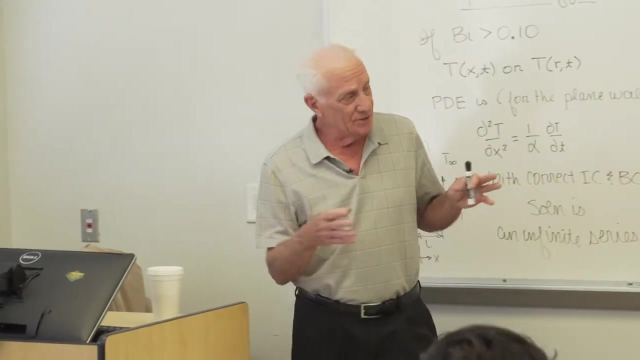 if the B-O number is greater than one-tenth, we no longer can use that very simple model which is called the lumped heat capacity model LHC. So that's today's topic, The first part: if the B-O number is less than one-tenth. 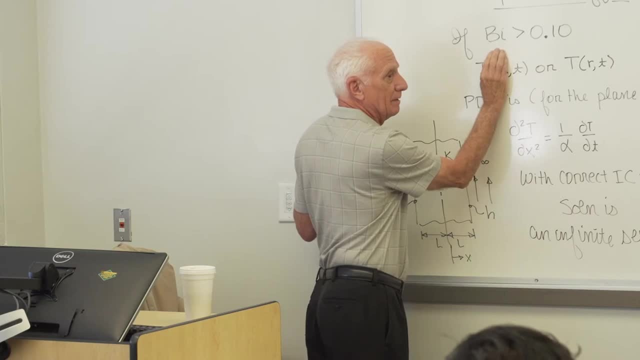 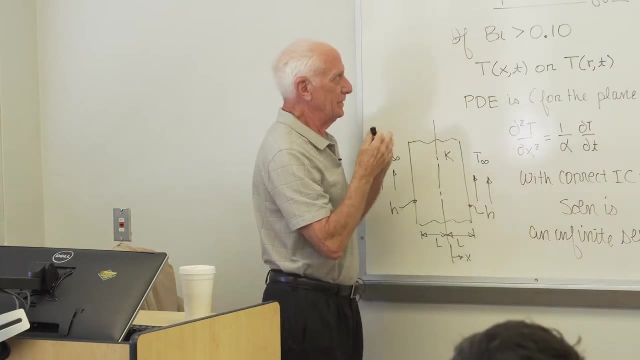 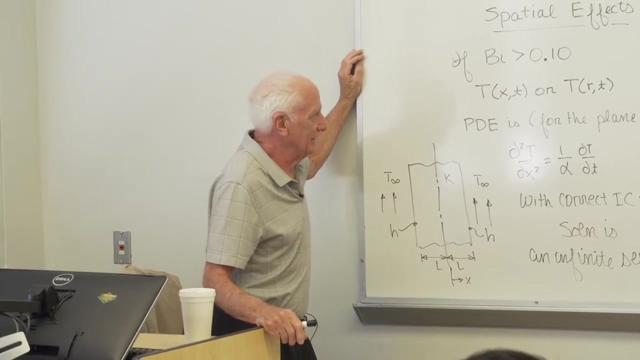 the temperature only depends on time, not of x. The temperature only depends on time, not of r. Now, B-O number greater than one-tenth. now it depends on two variables: x and t, or r and t, If we look only at a plane wall. 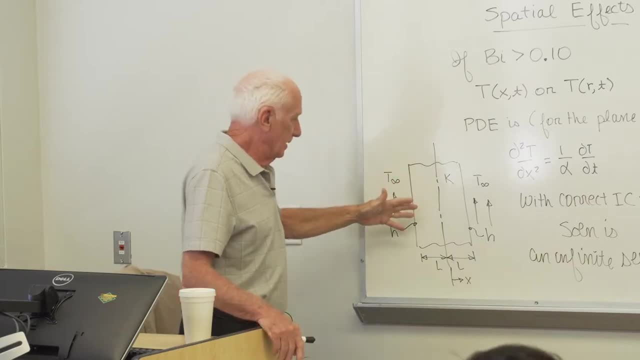 and we described the plane wall last time. here's the plane wall. its thickness is 2L. We measure x from the center line. x equals zero. The thickness is two times L. There's a fluid blowing over the left and right-hand sides at temperature t infinity. 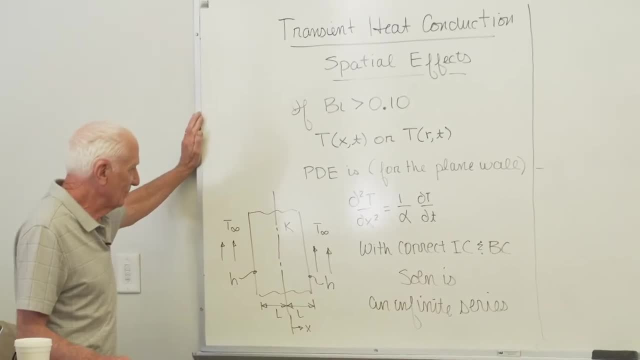 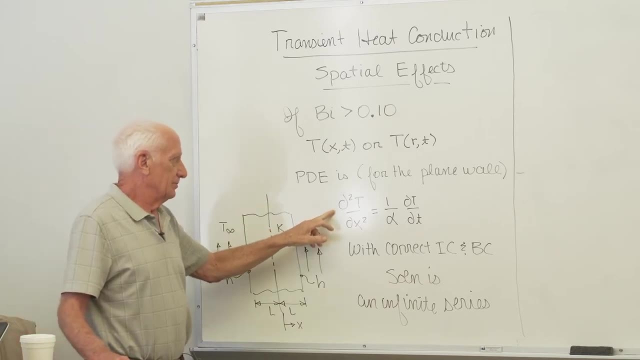 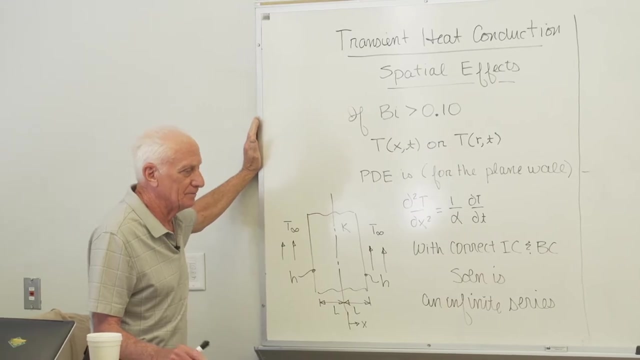 The convection coefficient on both sides is h and the correct partial differential equation for this problem would be: partial square t with respect to x, one over alpha, partial t with respect to time. With the correct initial and boundary conditions, the solution would be pretty long: an infinite series. 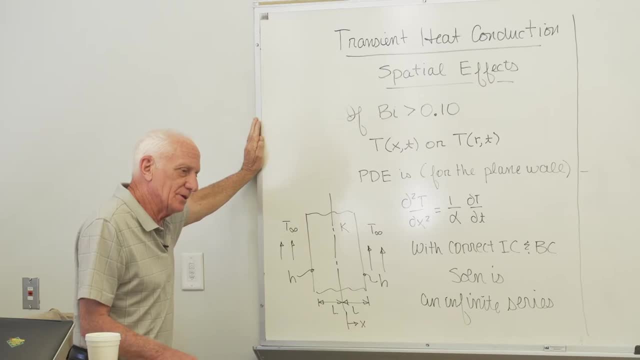 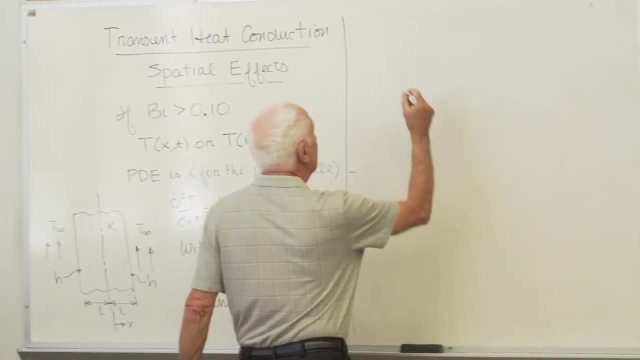 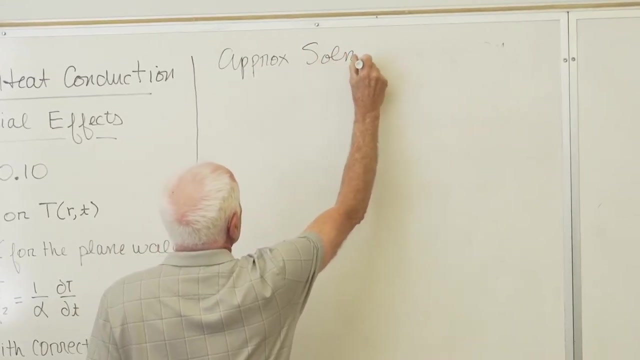 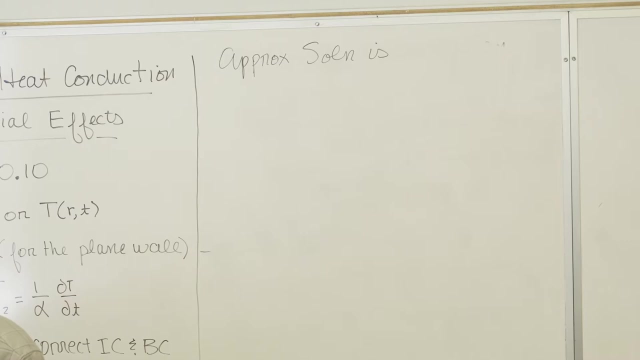 But we're going to look at only a one-term approximation to the infinite series. So because the infinite series is so long, we'll focus on a one-term approximation. So approximate solution is as follows: All right, So we take a look. first of all, 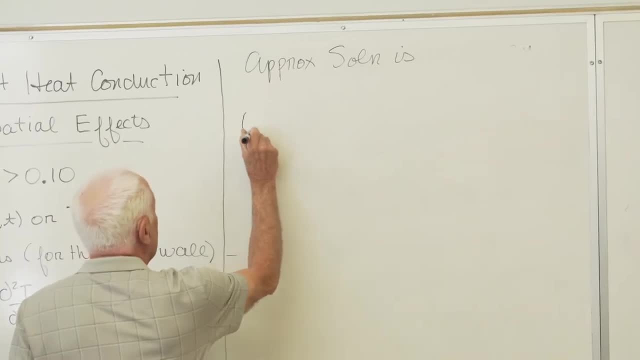 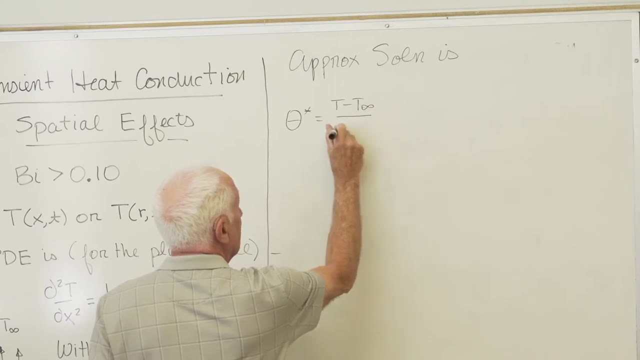 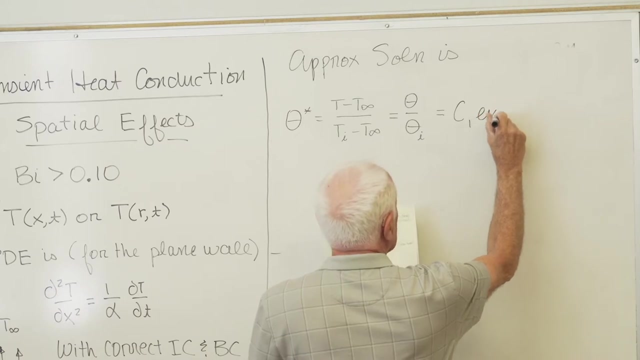 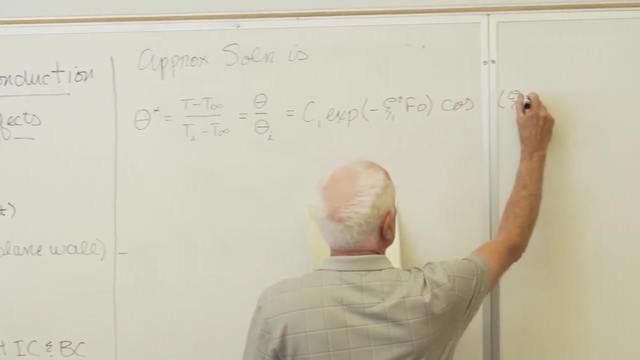 at something called Theta star and Theta star, t minus t infinity divided by t initial minus t infinity, That's really Theta over Theta i, Theta being t minus t infinity. C1 exp minus Zeta 1 squared. Fourier cosine of Zeta 1 x star. 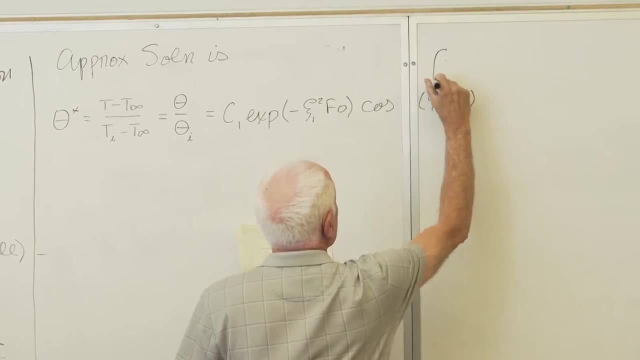 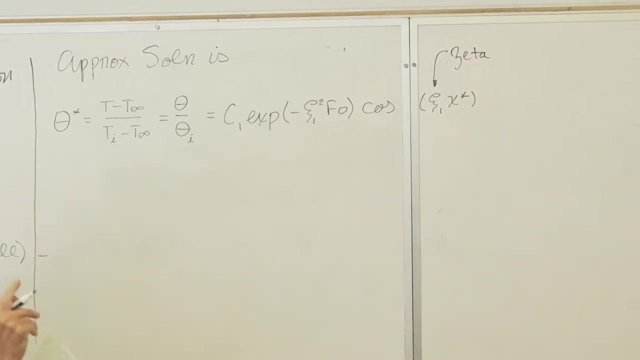 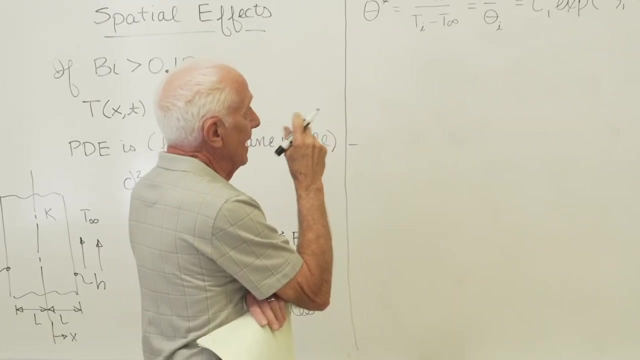 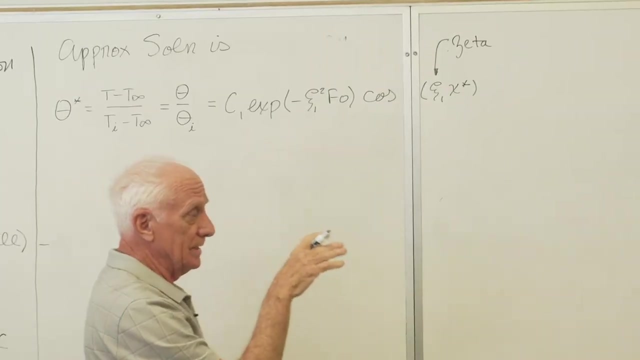 Zeta 1 x star. That's the one-term approximation of the infinite series, the first term approximation. Now there's two constants in there: There's C1 and there's Zeta 1.. We're going to mention how you get those. 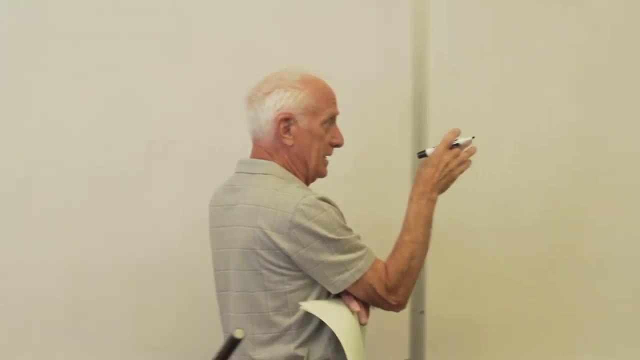 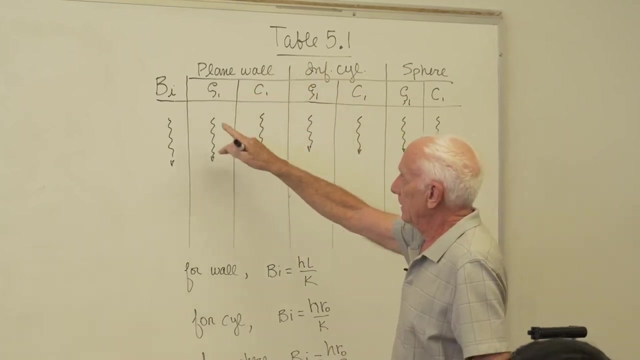 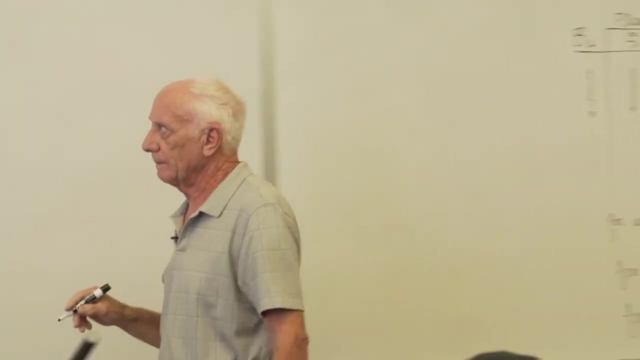 But just looking ahead a bit, we're getting those constants from table 5.1.. If it's a plane wall like over there, Bo number here, Zeta 1, C1. here That's how we get those constants. 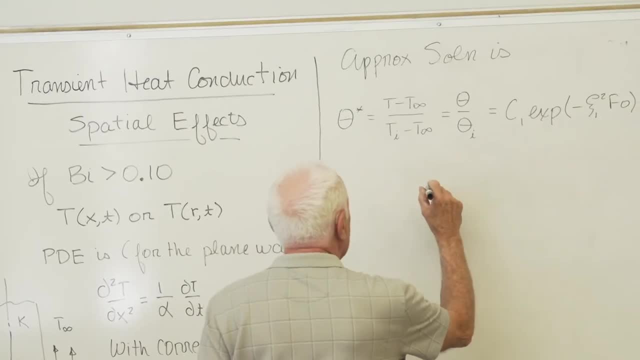 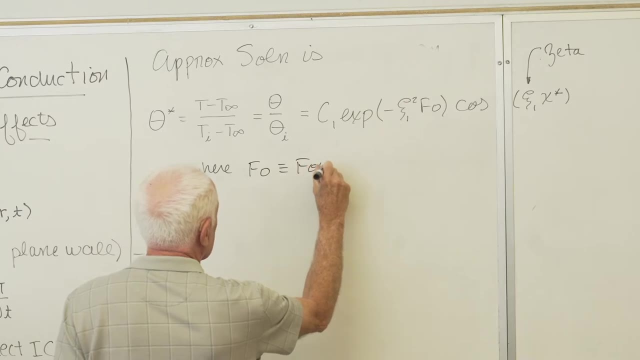 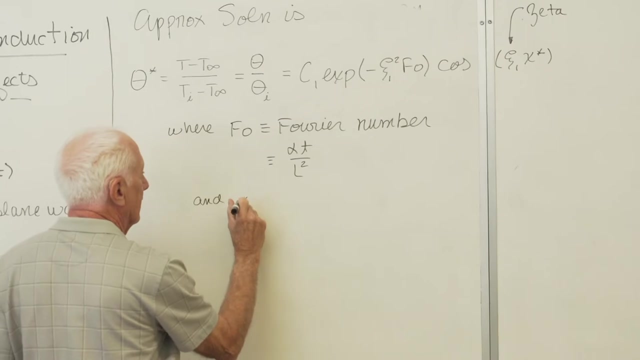 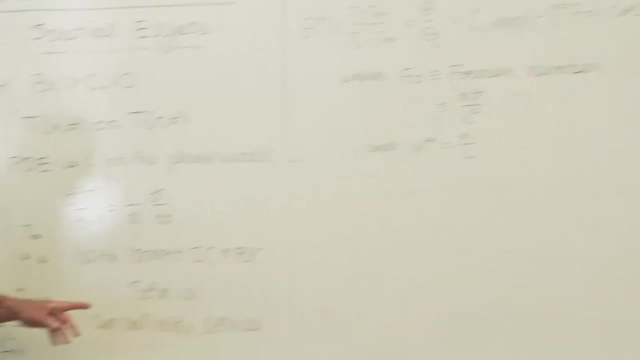 Now Fourier number: alpha t over L squared, What's L? again Half the wall thickness And x star equal x over L. So at the center line x is 0.. So x star is 0.. At the right-hand wall. 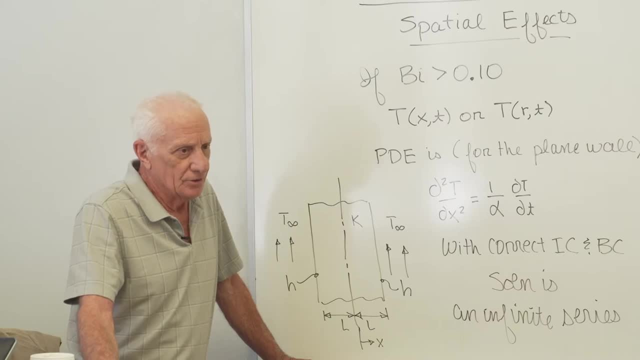 x is equal to L, So x star equal 1.. So x star varies from 0 at the center line to either plus or minus L, plus or minus 1,- pardon me, at the left or right-hand wall That equation is written. 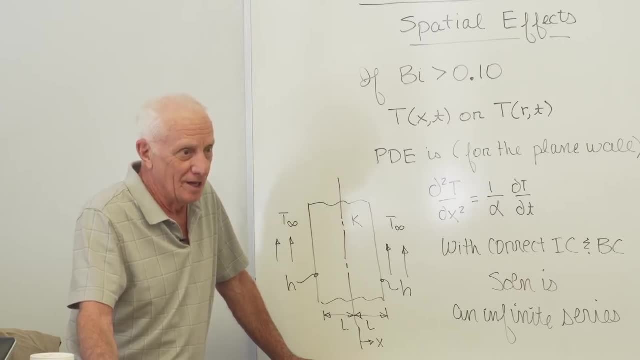 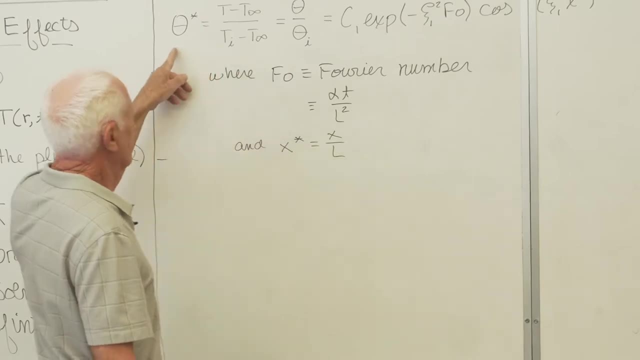 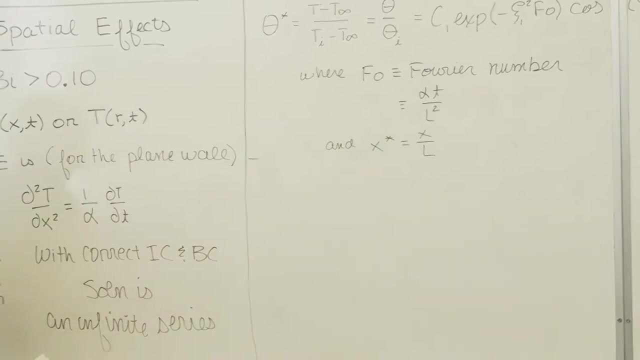 in a lot of dimensionless quantities. That's what we engineers love. That's why we do stuff like that. We love to make it dimensionless. Fourier is dimensionless. Theta star is dimensionless. X star is dimensionless, So 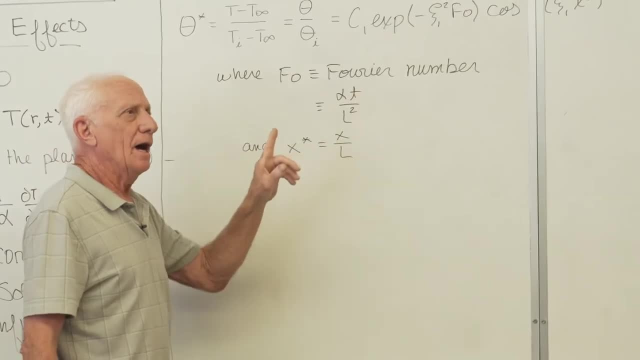 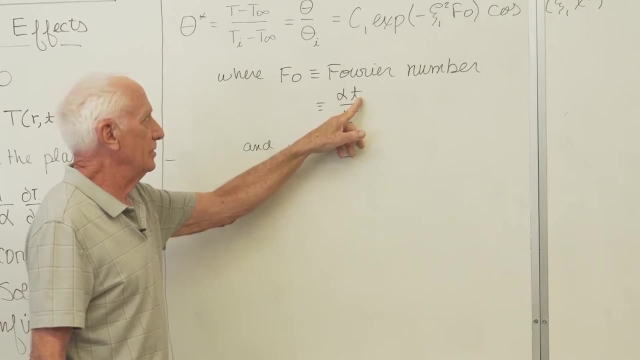 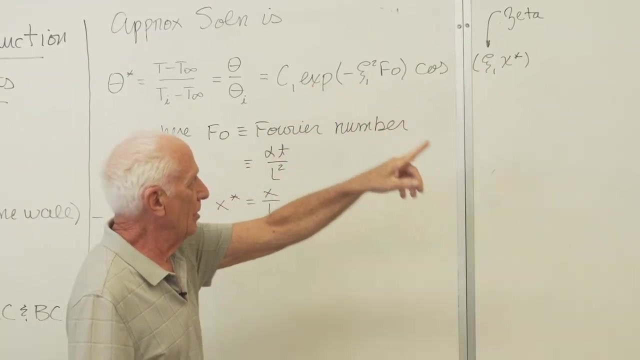 you give me a time. You say I want to know the temperature at a time of 1,000 seconds. Put it in here. get the Fourier number put it in here. get Zeta 1 and C1 from that table. 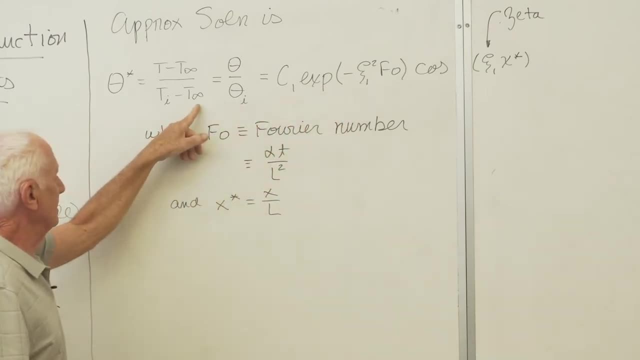 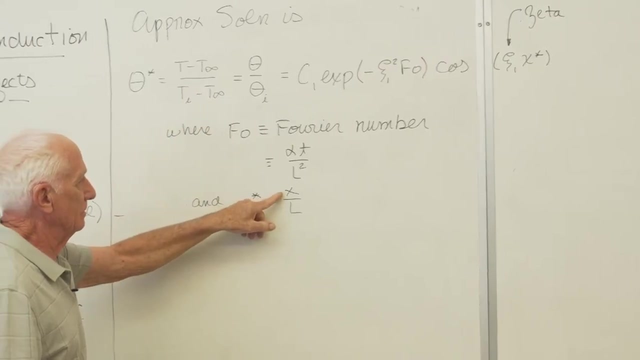 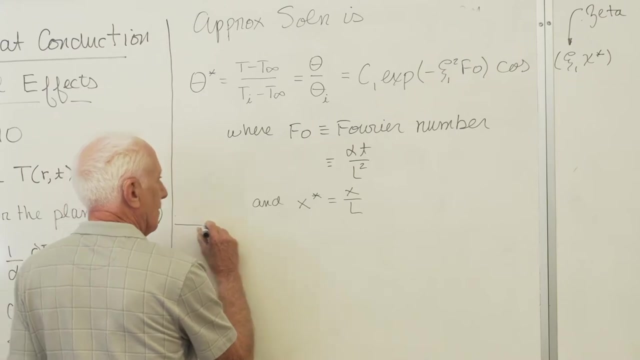 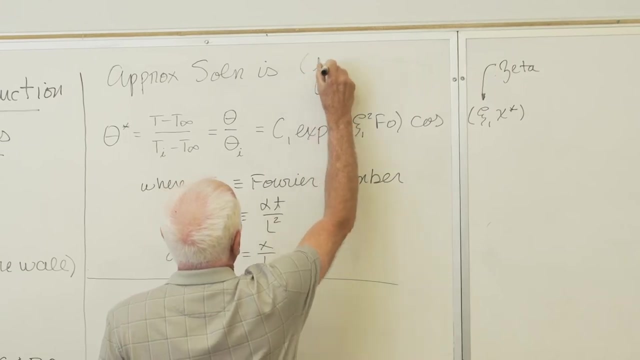 put them in here, do what it says. I know T infinity typically. I know T initial typically solve for the temperature Where At that x value and that time X and time there. So that's how we solve for the temperature, for T as a function of x and time. 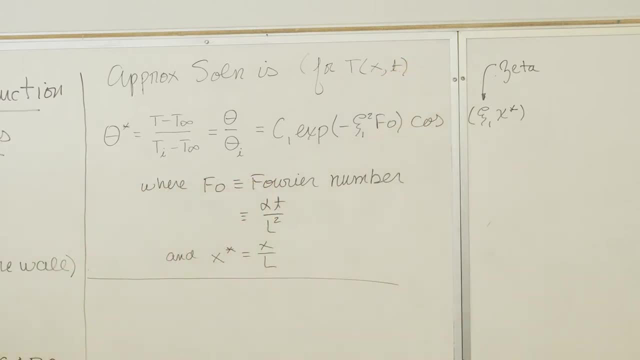 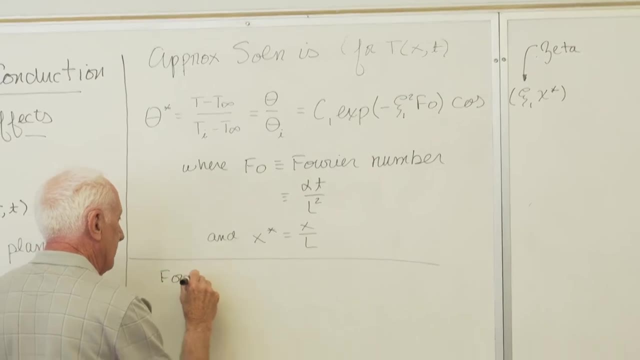 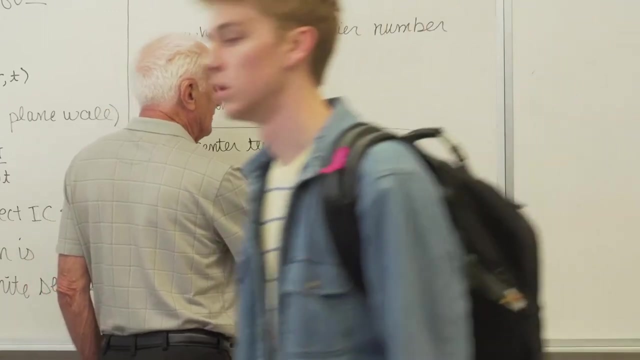 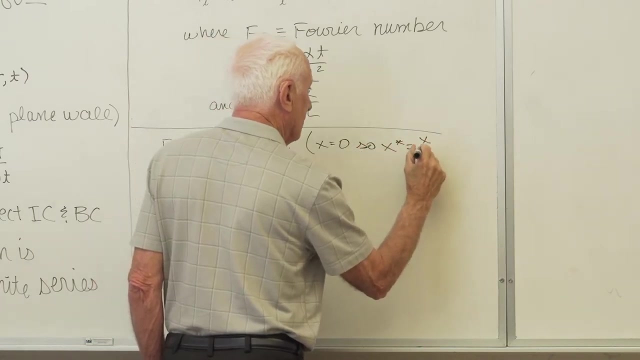 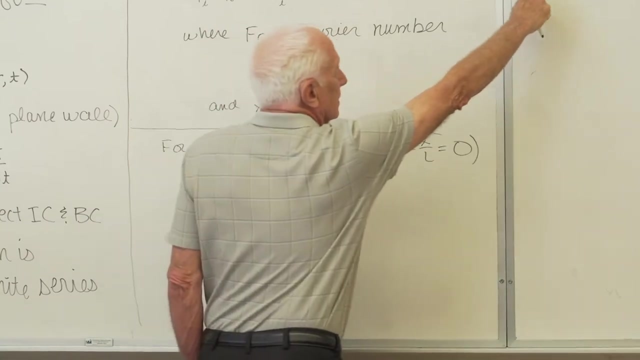 You give me x and time and I'll tell you a temperature. Now for center temperature at the center, x equals zero. So x star equal x over L equals zero. Cosine of zero is one. This cosine becomes one. 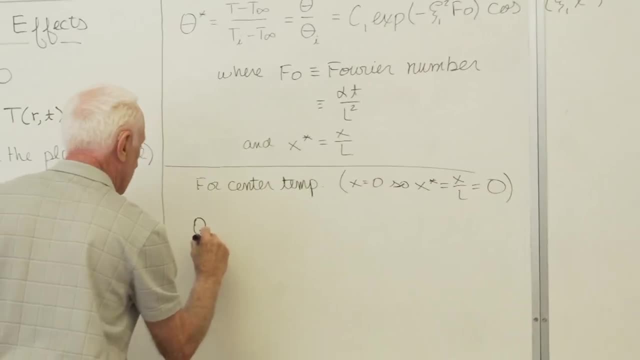 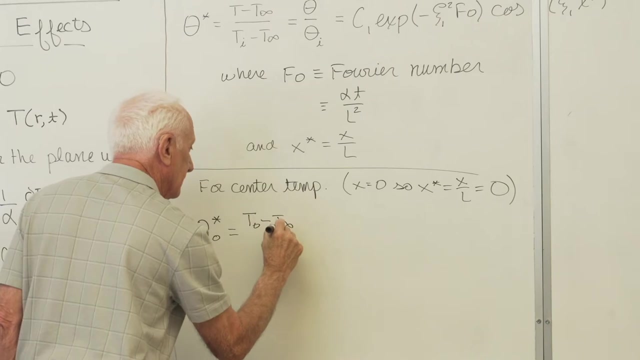 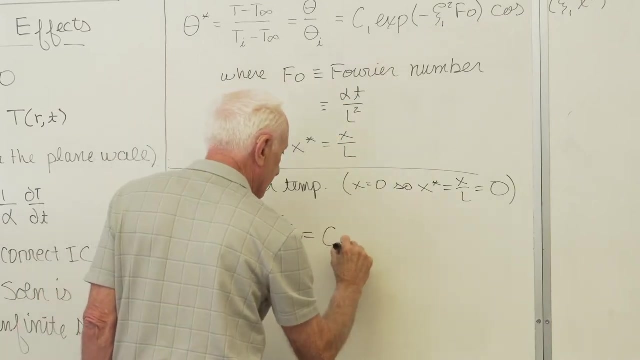 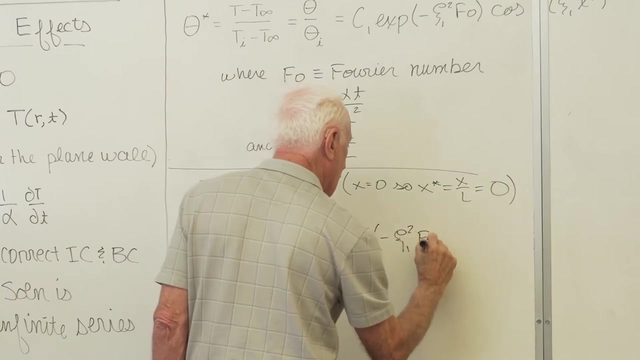 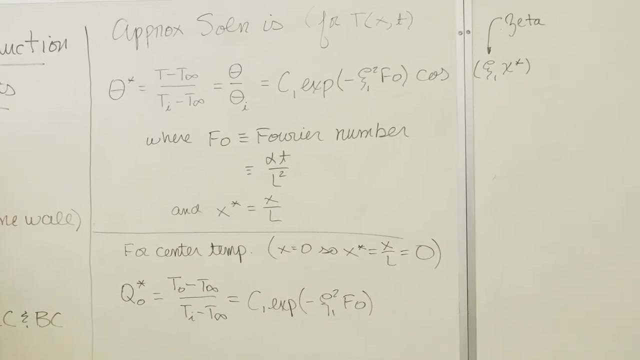 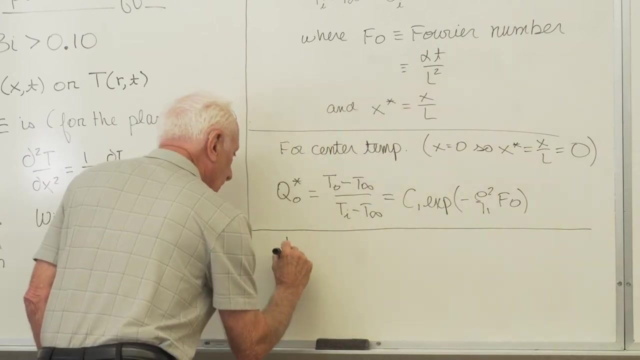 So Theta naught star equal T, center minus T, infinity T initial minus T, infinity C1 minus Zeta 1 Fourier, Zeta 1 squared Fourier. That's going to give me the center line temperature. Now for the amount of energy transferred: Q. 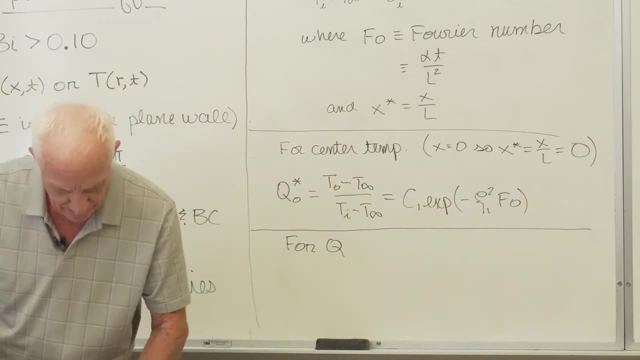 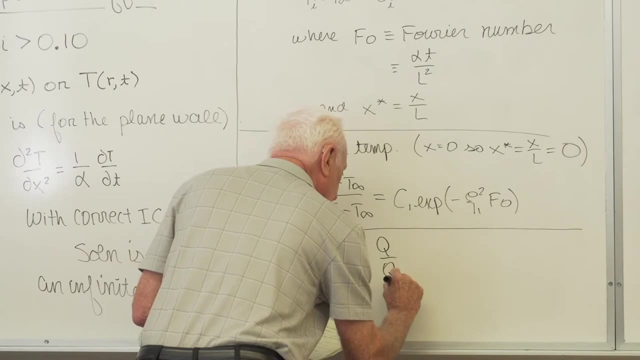 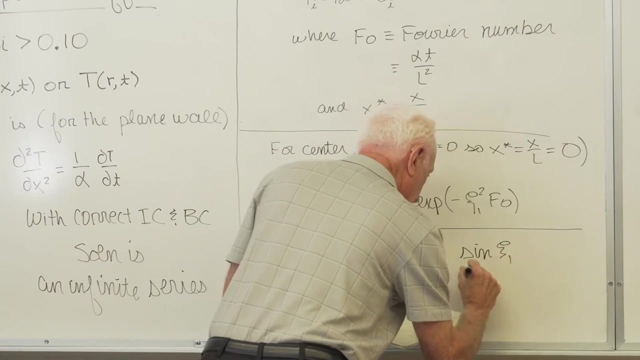 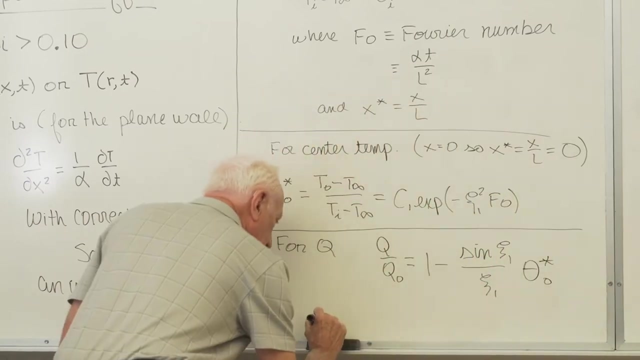 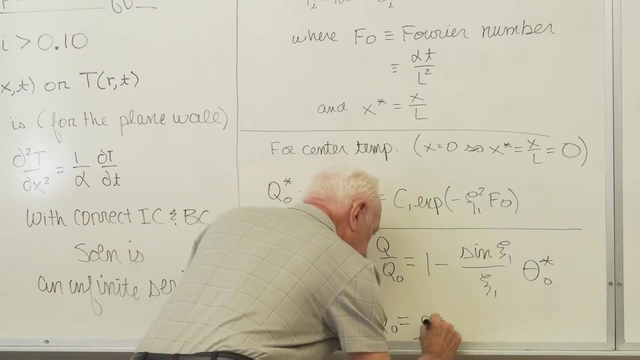 capital Q. let's see if I got that down. Oh yeah, For the center line temperature, Q over Q naught, and I'll mention Q naught in just a minute. Q naught is how much energy is stored initially in the object with respect to. 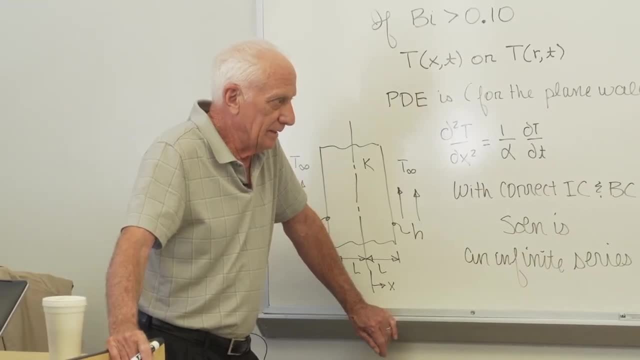 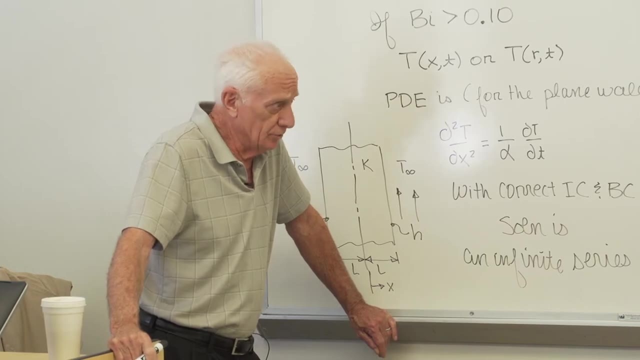 the surrounding fluid temperature: T infinity. T initial minus. It's the initial stored energy of the body. That's what Q naught is. Don't forget capital Q, T is in joules. Now the equation numbers, just so if you want to check those in the book. 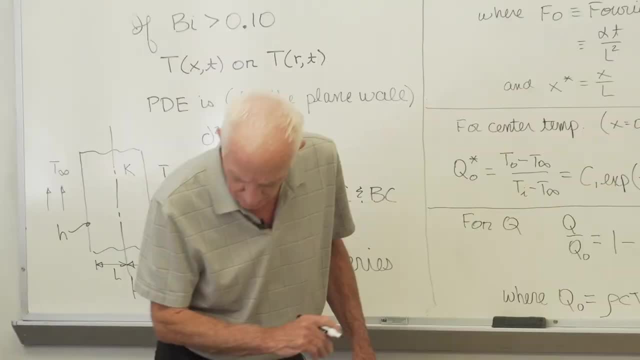 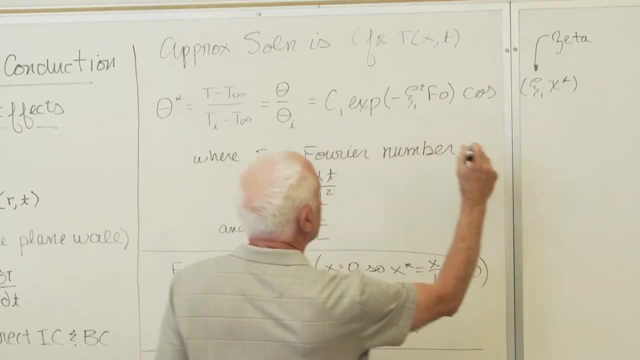 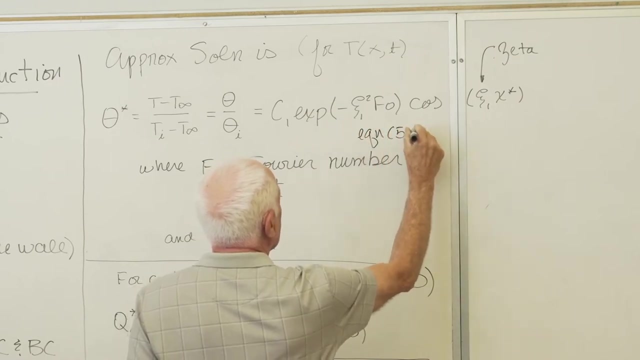 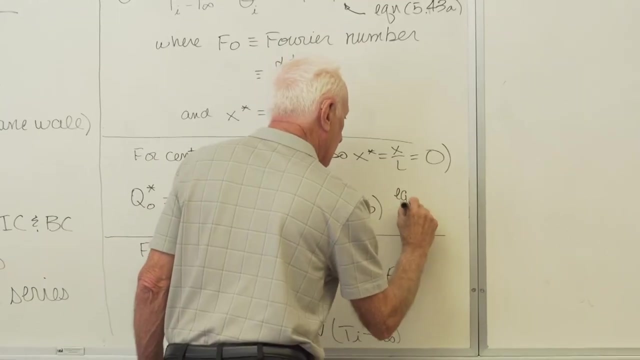 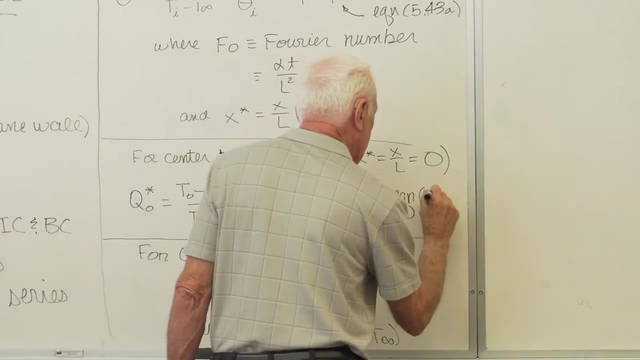 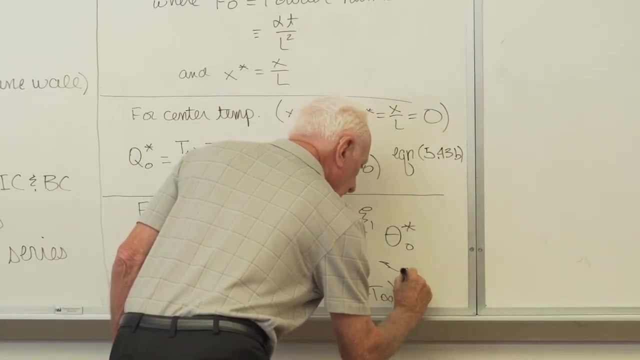 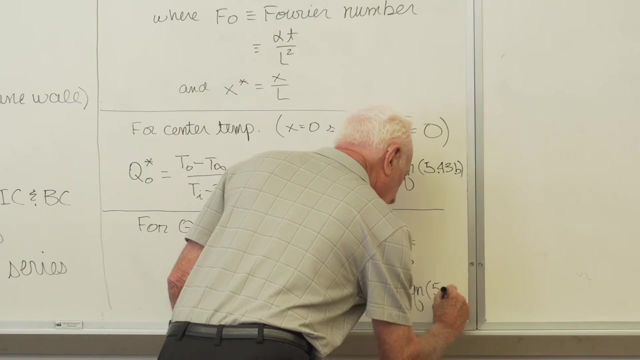 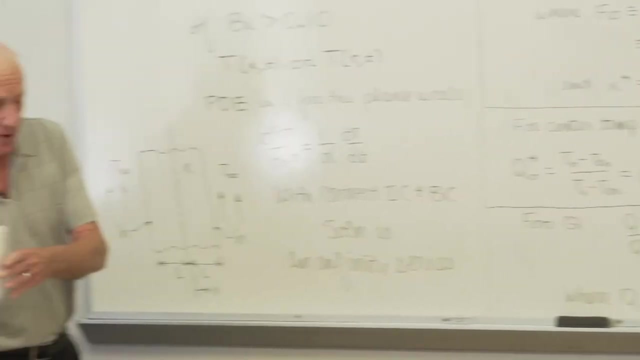 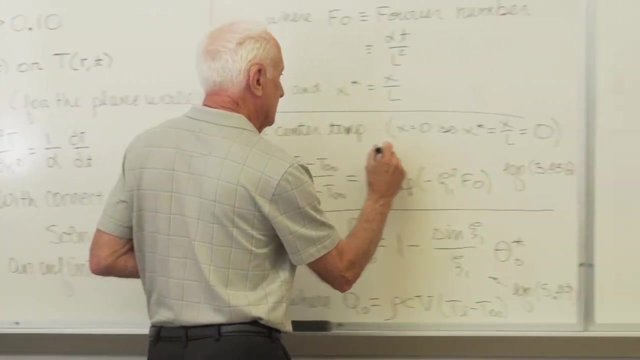 the first one is equation 543a. I'll put it here. This one is equation 543b. This one is equation 549.. So you've got three equations. One gives you the temperature. I'll put this down For the center temperature. 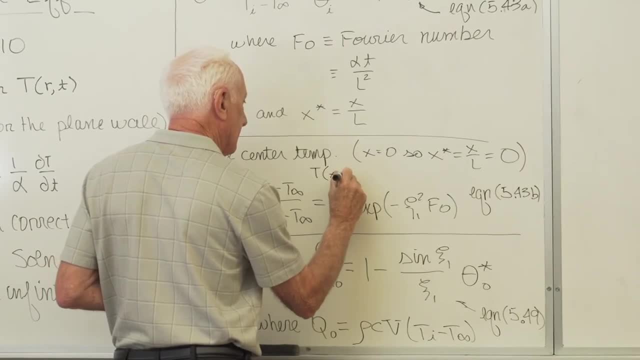 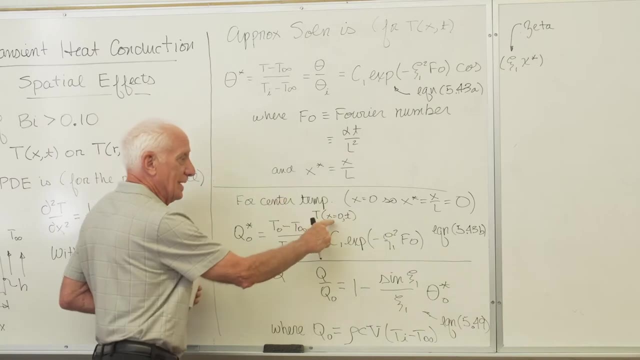 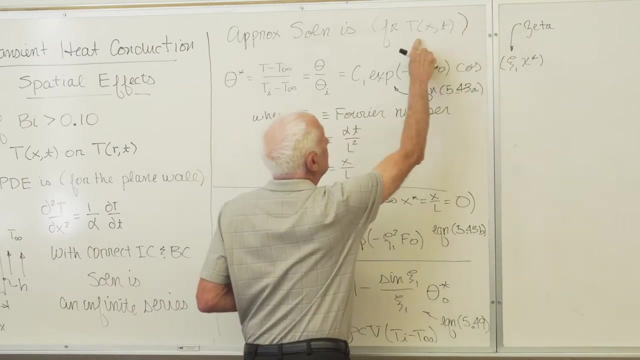 T, where at x equals zero for any time T. that's what that gives you. So you can find the temperature at the center line, equation 543B. You can find the temperature at any x value, equation 543A. or you. 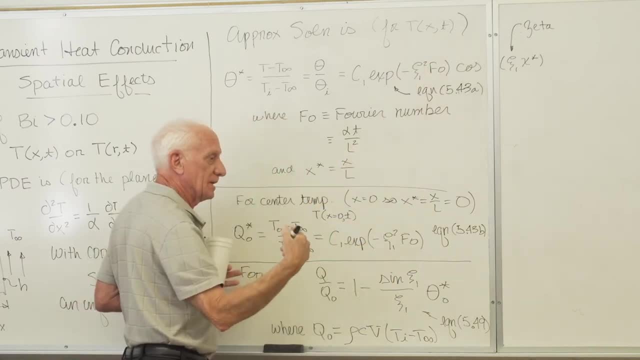 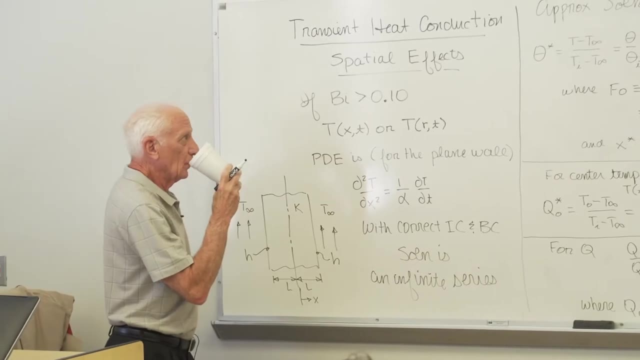 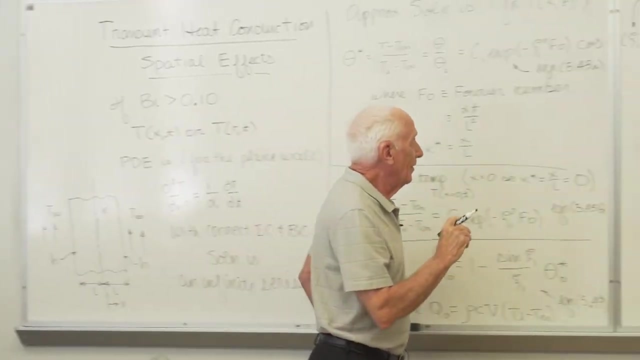 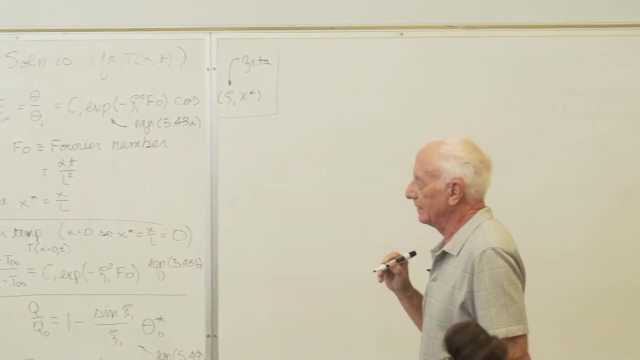 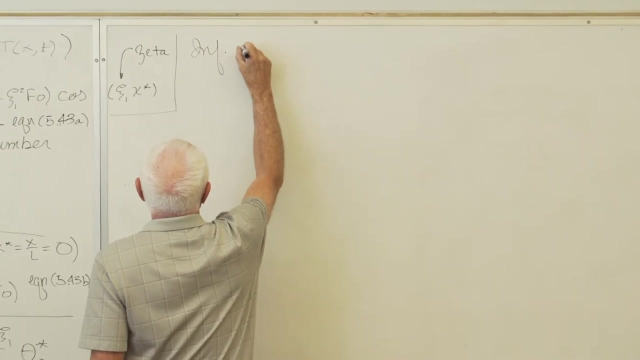 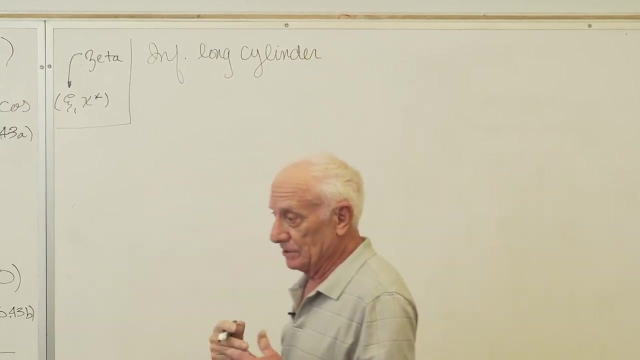 can find how much energy has been transferred from time zero to whatever time T by equation 554.. For what kind of geometry? A plane, wall, Three equations. Now let's take a look at an infinitely long cylinder. By that we mean, if its length 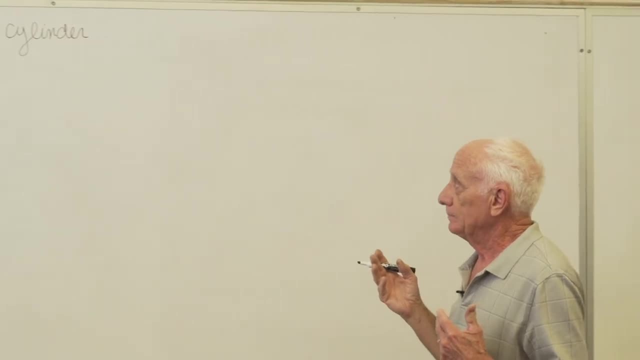 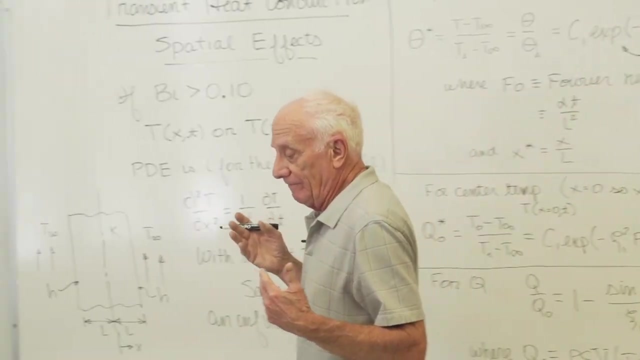 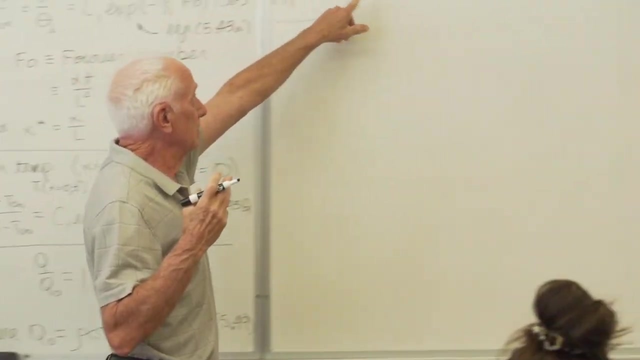 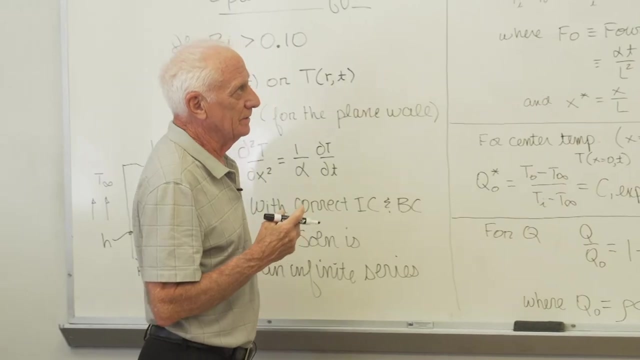 is a lot greater than its diameter. If you see a problem in homework or exam, it says: consider a very long copper wire. That tells me I'm going to assume it's infinitely long. One-eighth inch wire diameter, three feet long. Oh yeah, that satisfies it. 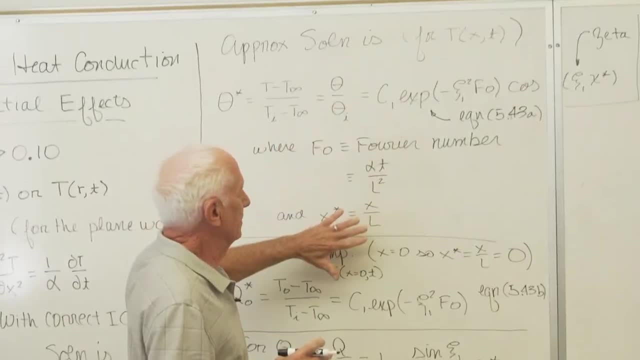 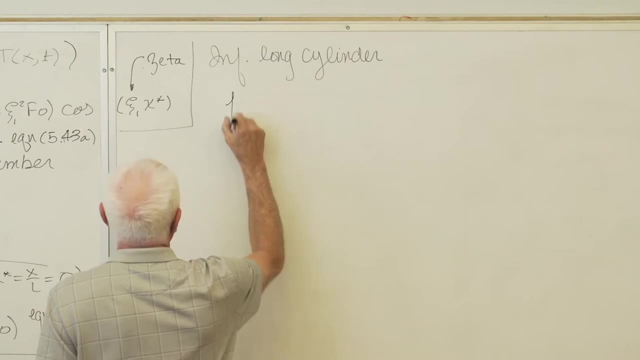 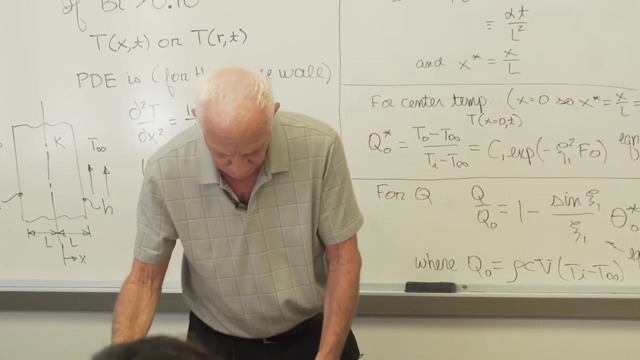 Okay, here we go again. three equations: The general equation, the temperature for any radius at any time, T. the outside radiuses are not. I'm not going to write the equations down, but I'm going to tell you what numbers they are. 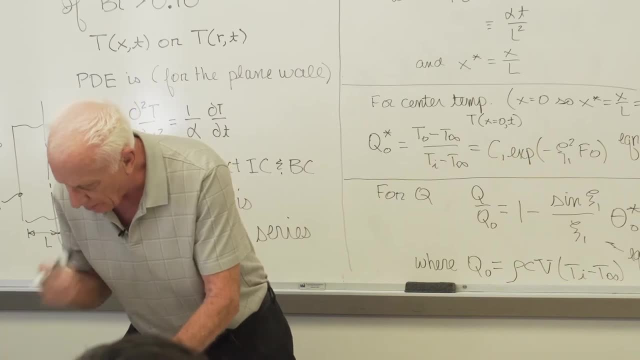 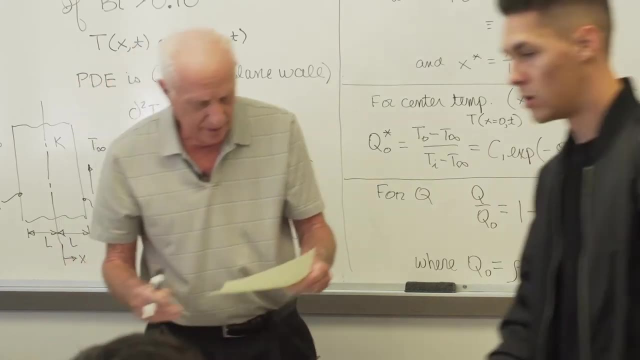 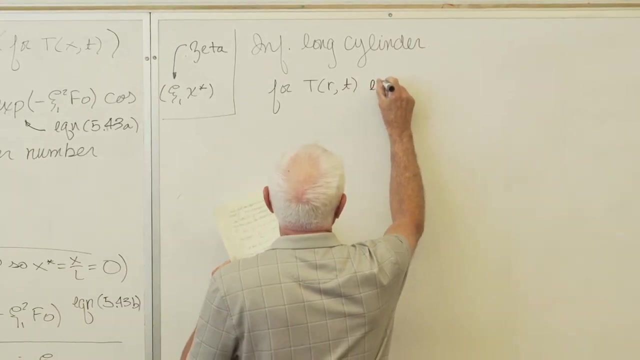 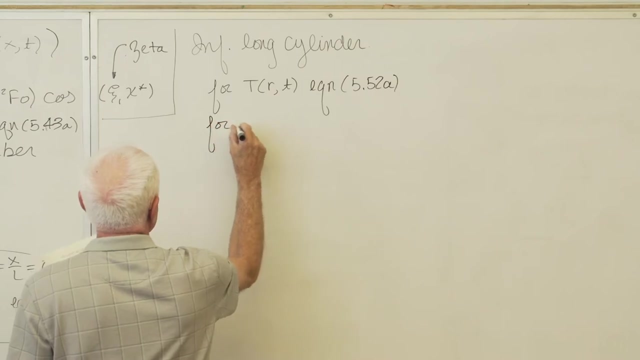 So for that one, let's see if I've got that written down here somewhere. Okay, that one. Yeah, here we go For T as a function of any radius in time. equation 552A For T at the center line. 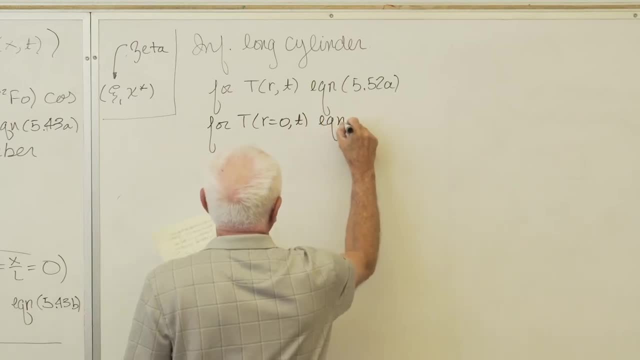 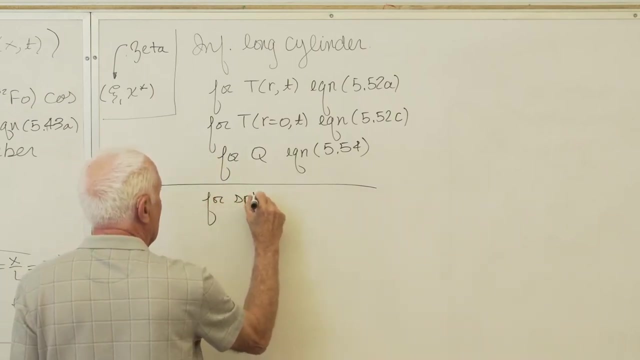 any time: T: 552C, Let's see 552C. yeah, For the amount of energy transferred in a certain time interval: 554.. Yeah, Yeah, Now the last of this. I'm going to describe three different geometries. 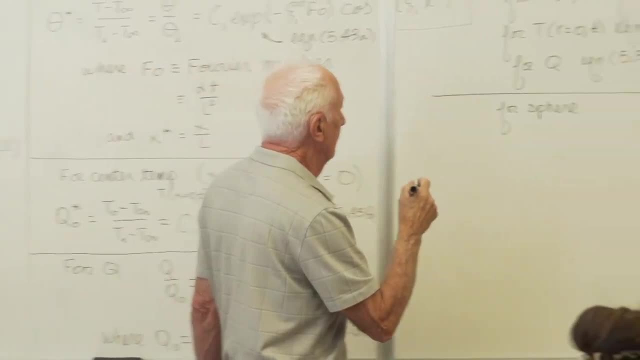 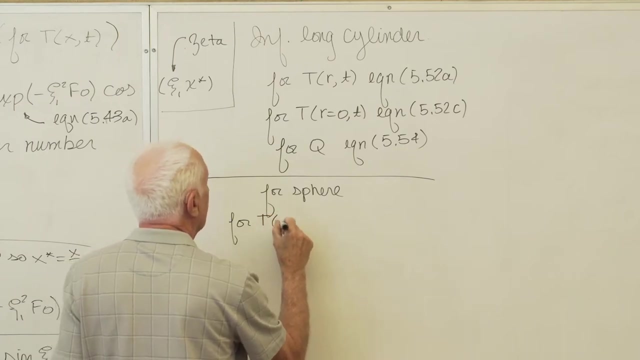 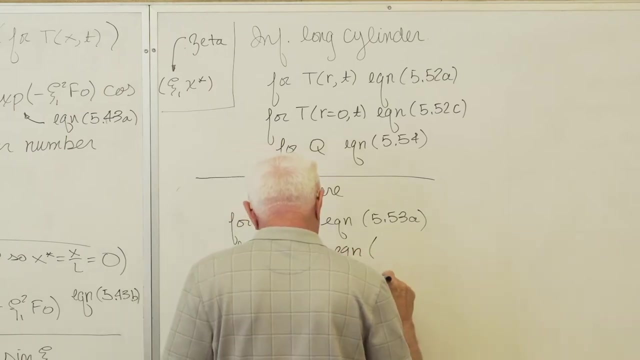 a plane wall, a long cylinder and a sphere. For the sphere for the temperature as a function of radius and time, equation 553A For the center of the sphere. 553C- either textbook For Q, either textbook. 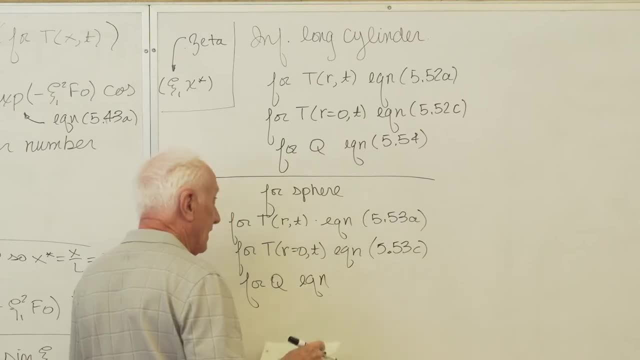 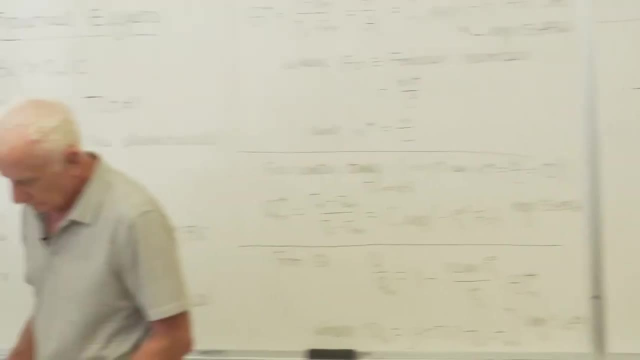 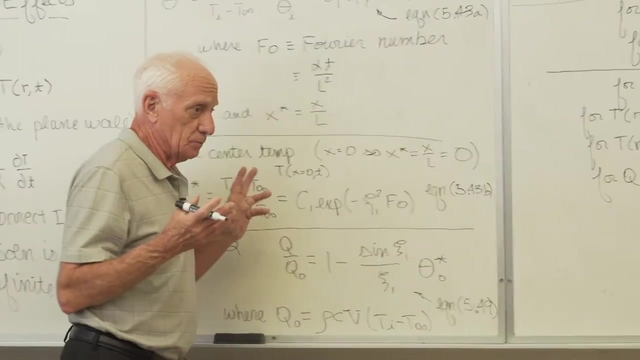 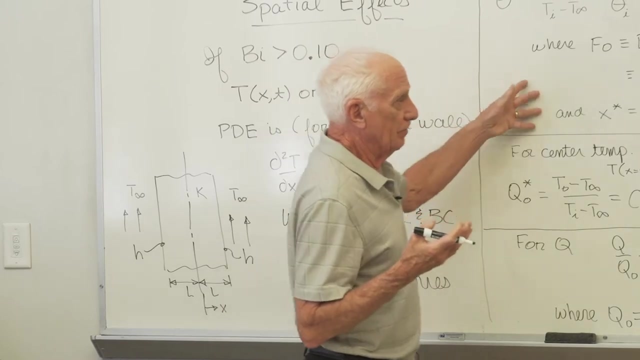 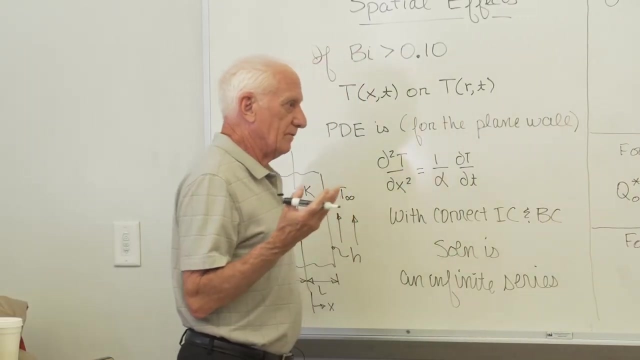 Q, equation 555.. So these are the three geometries our textbook focuses on. How many total equations are available to solve these guys? Three for plane walls, three for cylinders, three for spheres. nine, What's that for If the B0 number is greater than one-tenth? 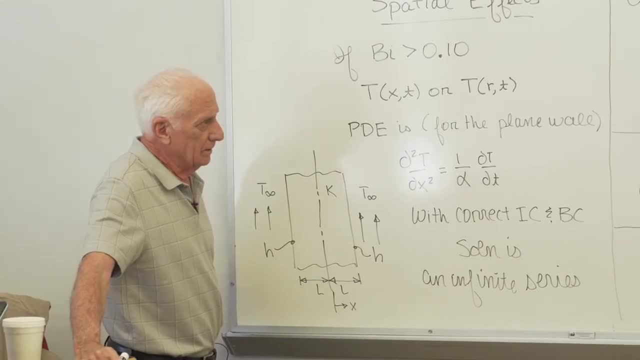 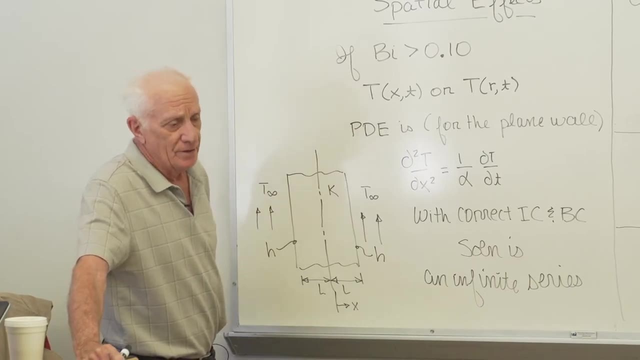 and you don't want to use lumped heat capacity, then you've got those nine choices. What if the B0 number is less than one-tenth? Oh, life is easier. B0 number less than one-tenth. there's only two equations. 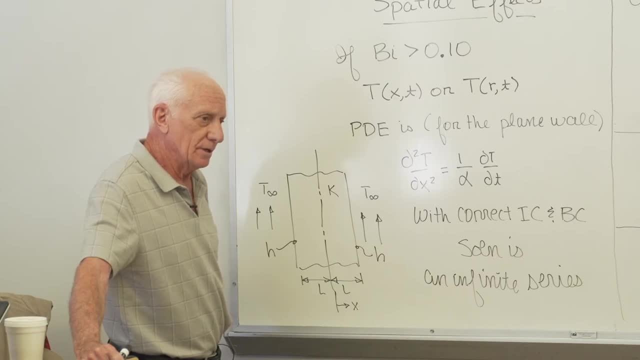 One gives you the temperature as a function of time. the other one gives you Q as a function of time. You don't see X in those equations, you don't see R in those equations. life is easy. But now, when the B0 number exceeds this? 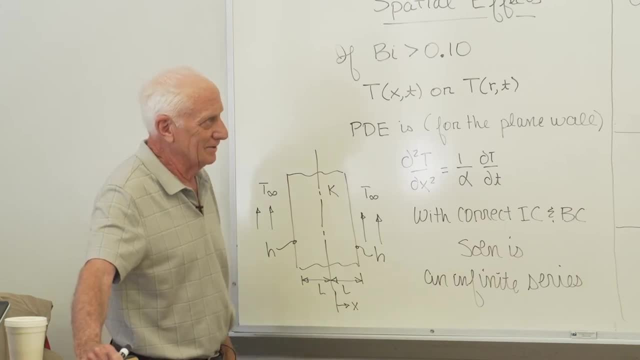 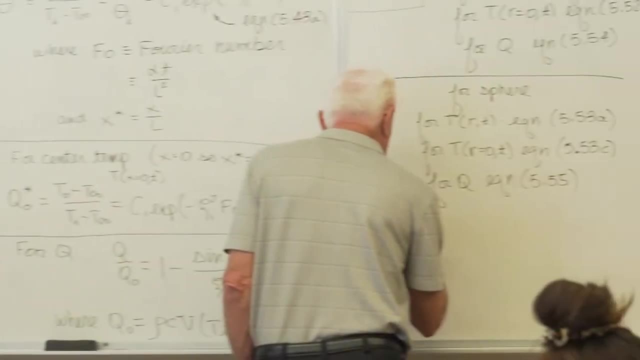 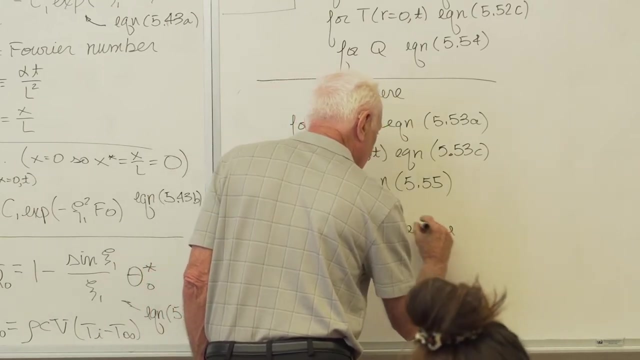 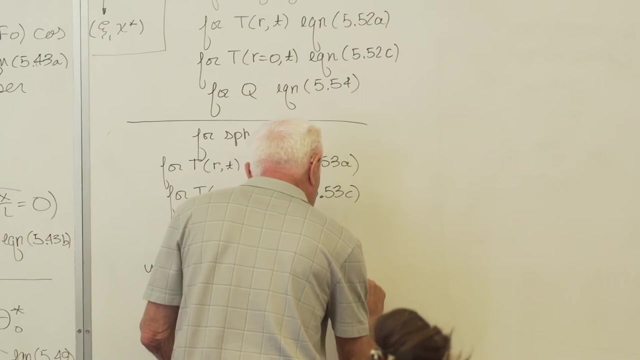 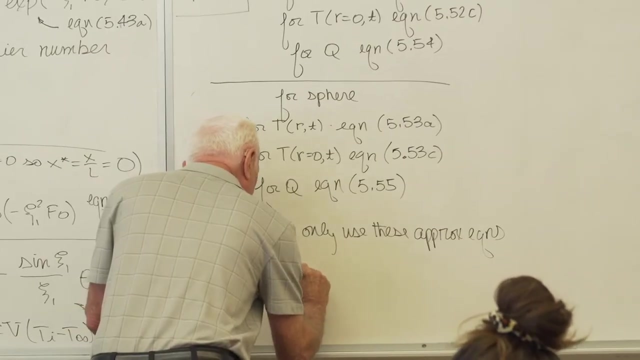 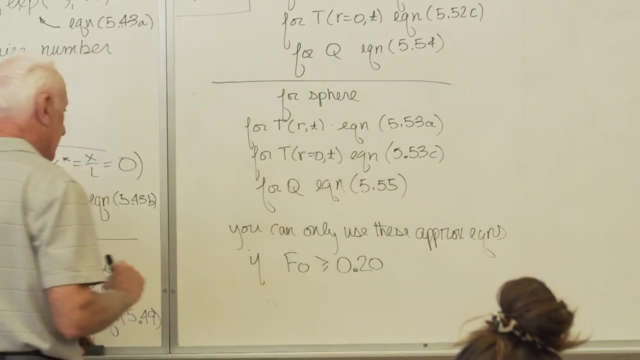 now you've got to go through much more complicated analysis. These are the first term approximations. You can only use these equations- approximate equations- If the Fourier number greater than or equal to 0.2.. Here's a Fourier number right here. 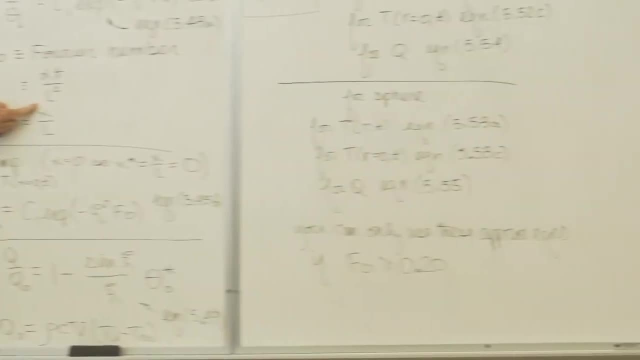 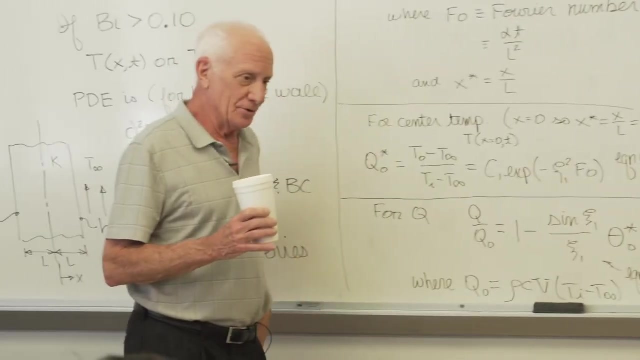 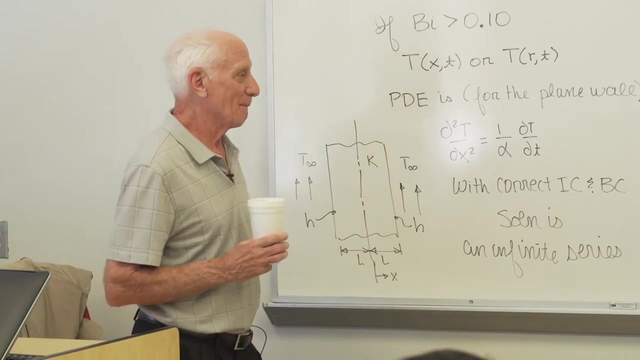 Fourier number? What if it's not? You can't use the one-term approximation. You got to go back and throw in more terms in the infinite series. The one-term approximation, the approximation won't give you an accurate answer, or an approximate answer even. 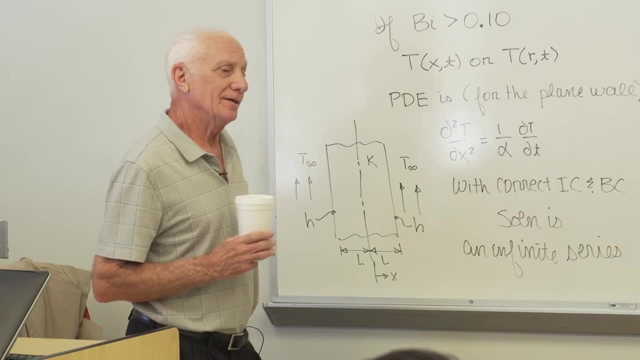 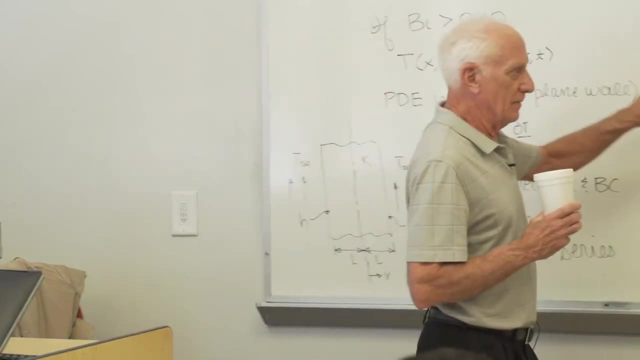 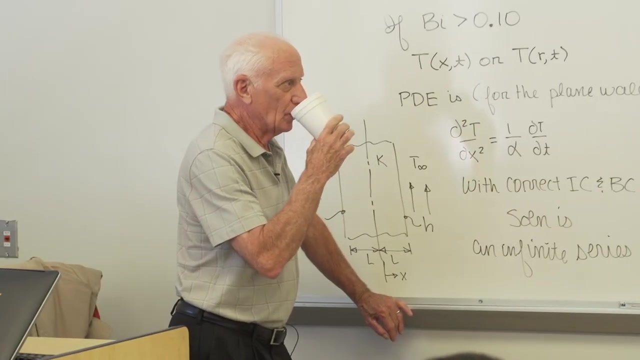 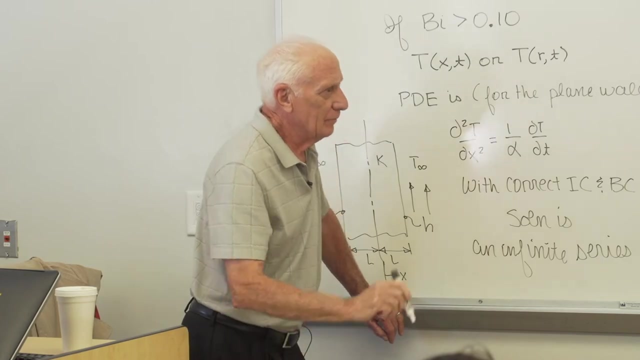 So you can see, in problems like this you might have to check two-dimensional parameters, the B0 number and the Fourier number. So that's two possibilities there. What does that physically mean when we have this guy right here? Well, as an example, 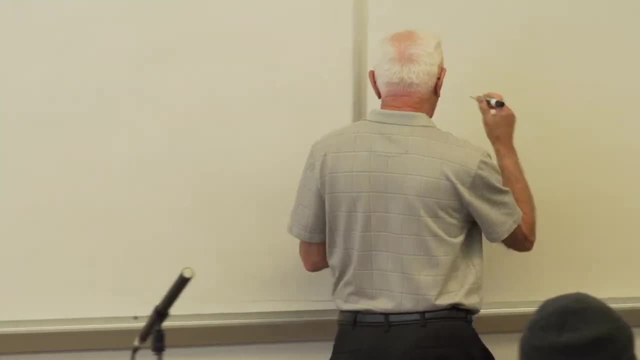 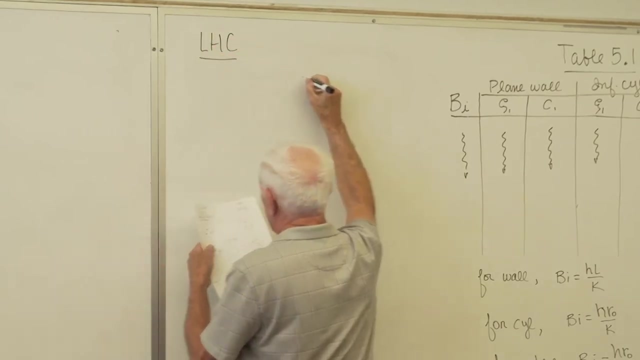 let me just sketch something that might help you visualize what's going on. We're going to cool a sphere With the lumped heat capacity model. what that gives us and the approximate solution are the actual, we'll say using the approximate solution. 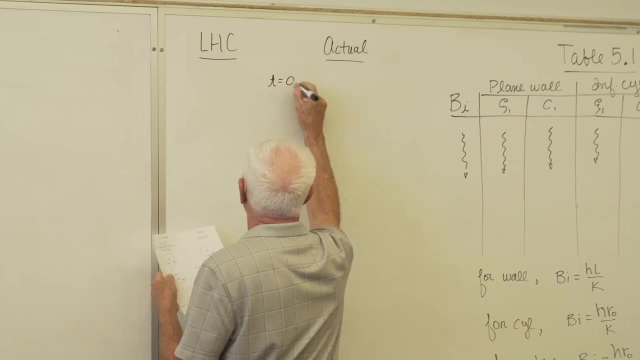 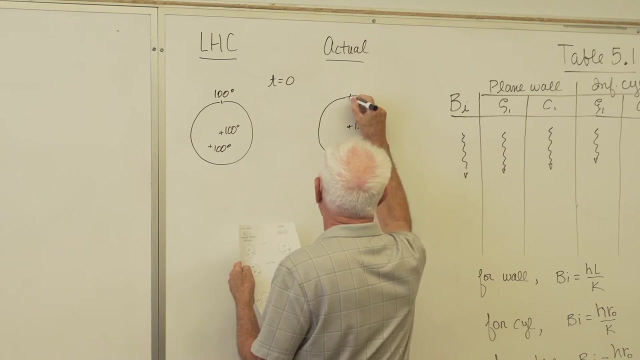 We'll start out at time equals 0.. We've got the sphere initially at a temperature of 100 degrees everywhere, A 100 degrees for both cases. Then we're going to just say, let's just say 60 seconds. 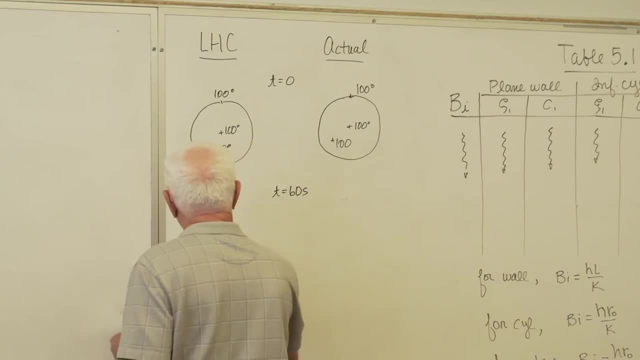 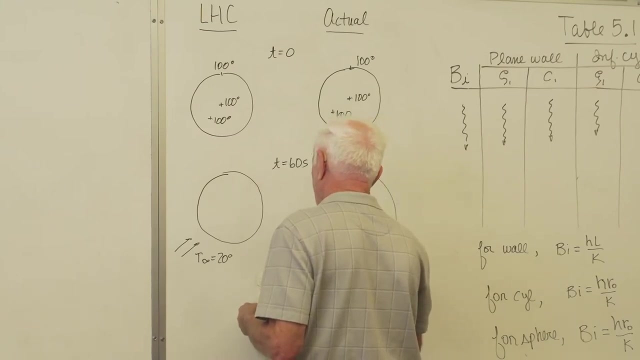 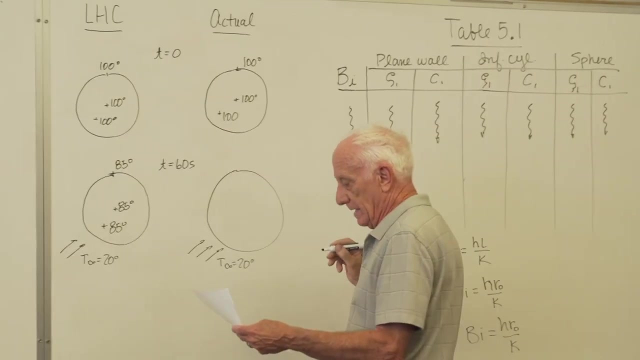 just make something up. Now I'm going to blow air over this. at a temperature of 20 degrees, This sphere might have cooled down now to 85 degrees. With the lump heat capacity model, it's 85 degrees everywhere. Actually, it might not be that way. 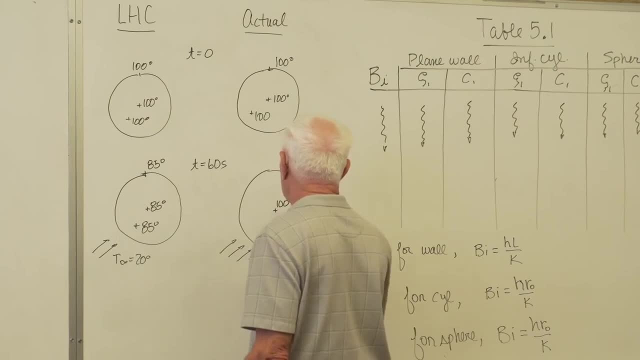 The center might not have started to cool at all yet. It might still be at 100.. This surface temperature might have cooled by a lot. It's down to 78.. Inside somewhere it might be 87.. Now we go to 120 seconds. 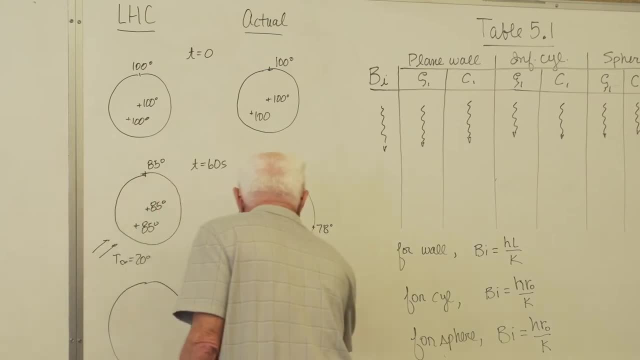 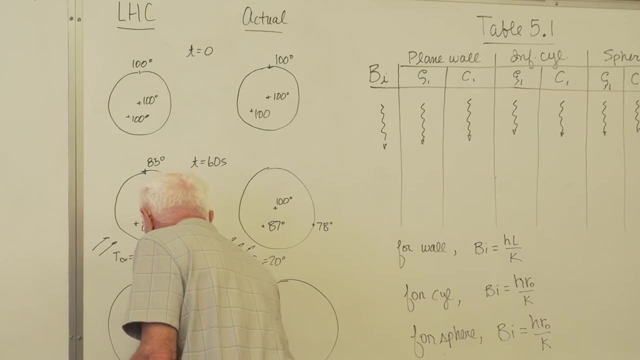 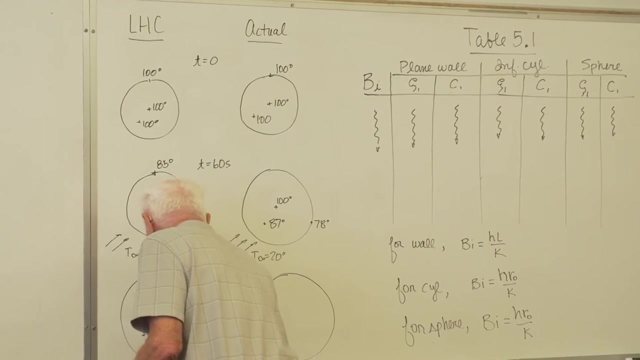 Lump heat capacity model. oh, it's cooled down now. It's down to 60 degrees, Where, Everywhere. It's not a function of radius, It's only a function of time. The real-world situation: Oh yeah, the outside is now cooled down to 50.. 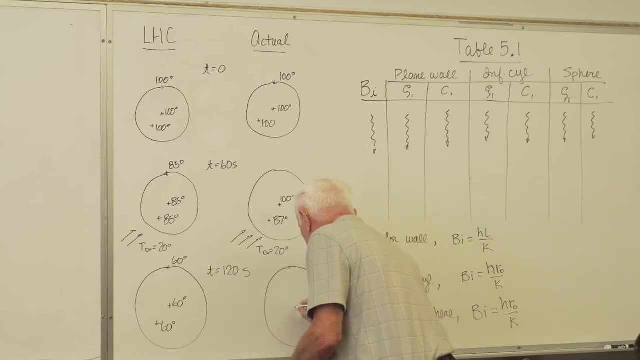 The center finally started to cool down. It's down to 90.. Somewhere else the temperature might be 70.. Lump heat capacity. Temperature is only a function of time. I don't care what the radius is. Actual VO number greater than 0.2.. 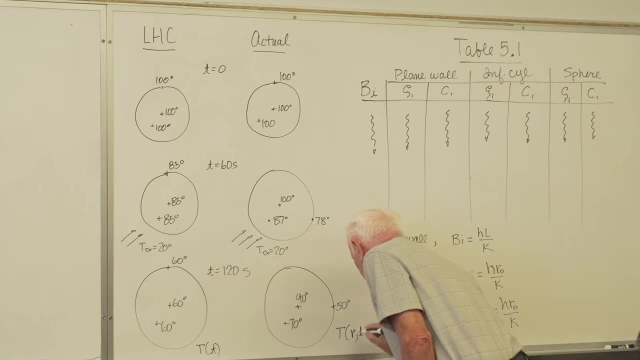 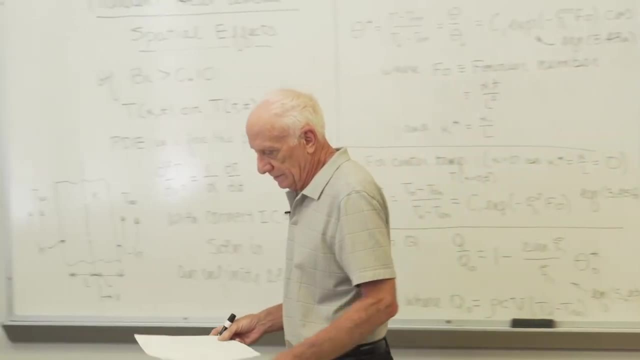 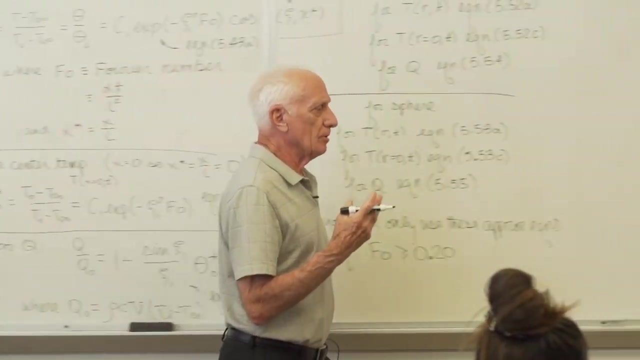 Temperature now is a function of the radius and of time, So that is a little physical feeling. for what does that mean when the VO number is less than or greater than 0.1.. The VO number is also a ratio of two resistances. 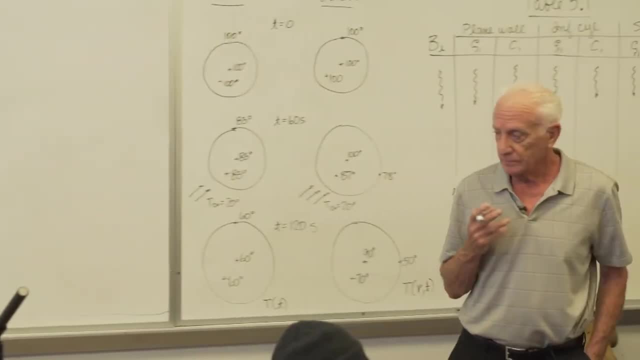 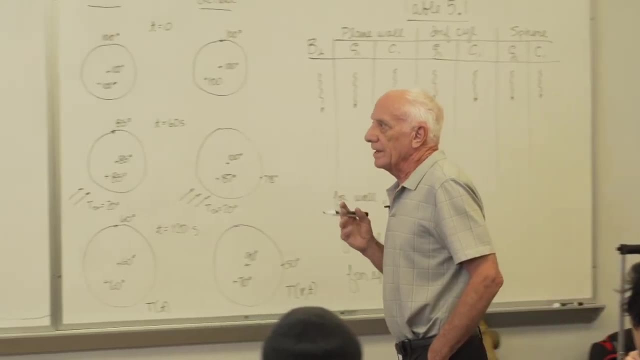 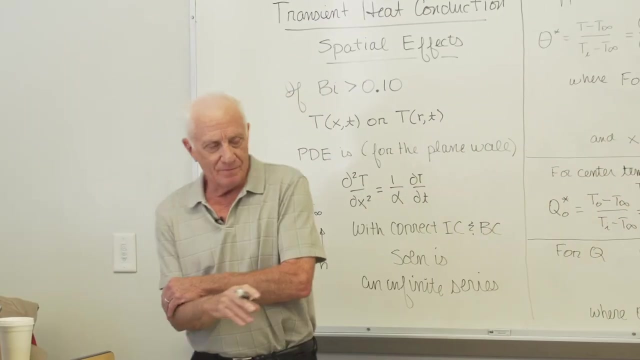 the conduction resistance and the convection resistance. So it's a measure of two resistances: conduction and the convection. So back to here. Yeah, life is more complicated when the VO number is greater than 0.1. In this textbook, you don't have to ever. 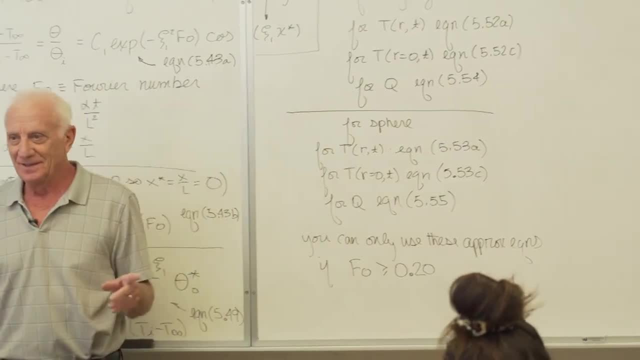 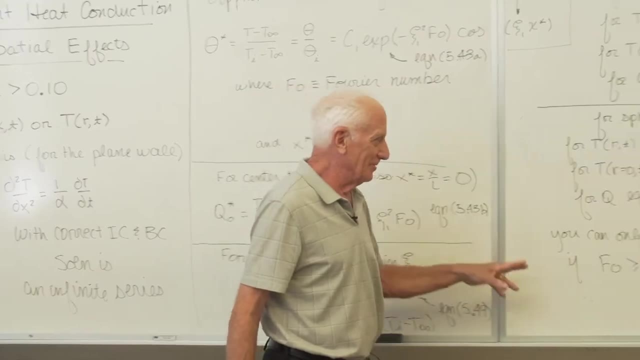 worry about this because he's not going to make you, at end of chapter problems, make you do an infinite series, So don't worry about that, Although you should always check that, just to make sure you're okay. I don't care if it's homework or an exam. 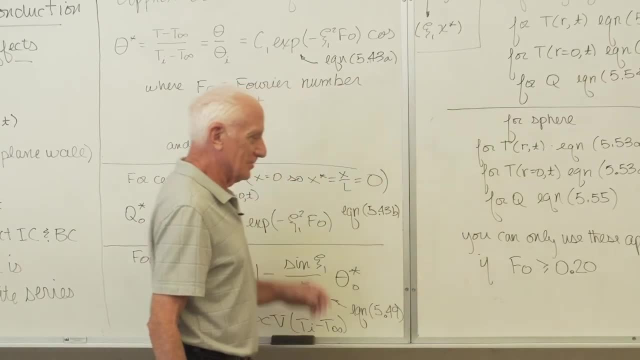 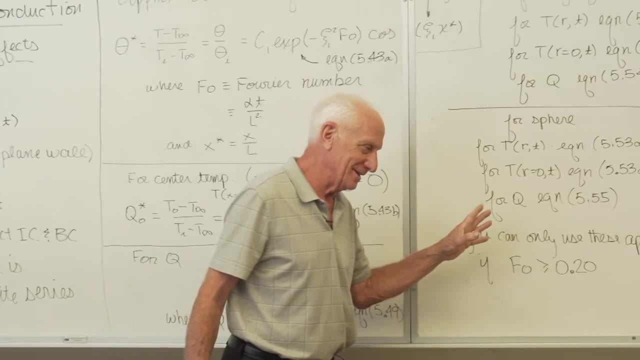 When you're done, check that guy and see if that's true, But here, regardless in this case, if it's not true, you probably made a mistake, because mostly all these problems are in here. Satisfy that. But just to check it. so you know you've checked it. 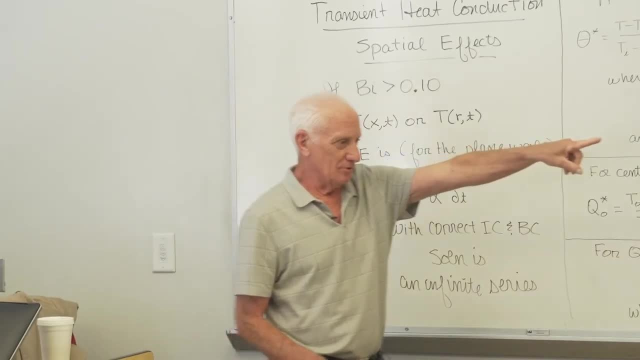 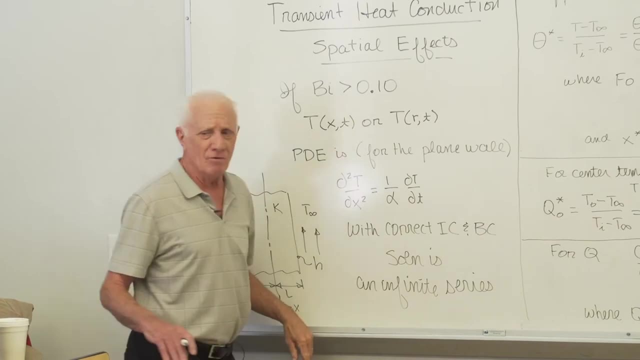 Okay, Nine equations, one table solving if the VO number greater than one-tenth. By the way, can you use this stuff if the VO is less than one-tenth? Of course you can. It's the actual solution to the PDE. 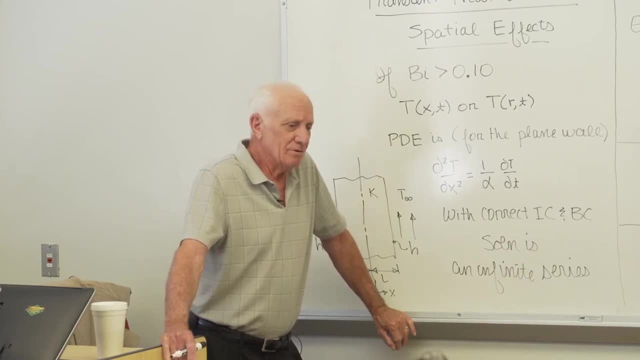 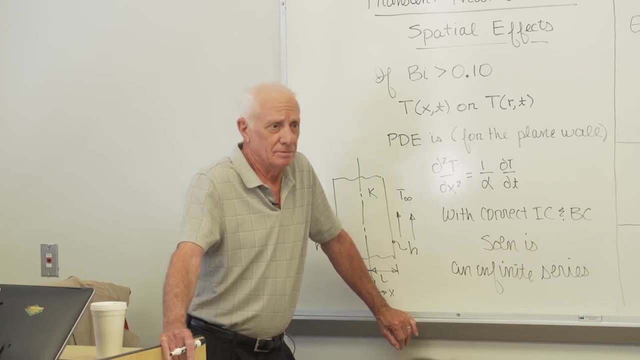 one term approximation? Sure you can, But why would you want to If the VO number is less than one-tenth? take the easy way out. How many equations are there? Two? You want to solve two equations, or maybe nine equations? 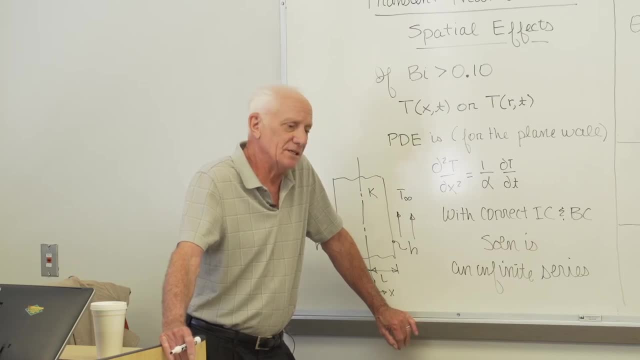 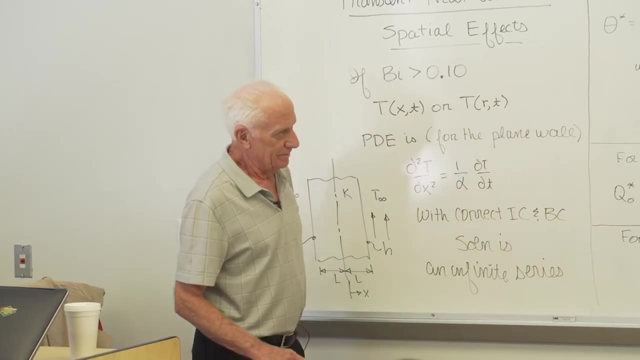 No, do the two. If the VO number is less than one-tenth, take the easy way out lumped heat capacity. Although the approximate solution works for any VO number, Lump heat capacity only works if the VO is less than one-tenth. 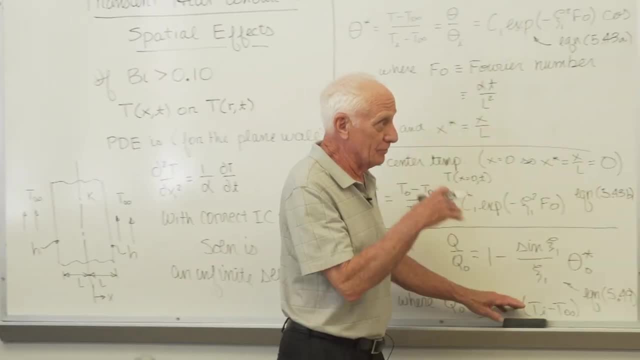 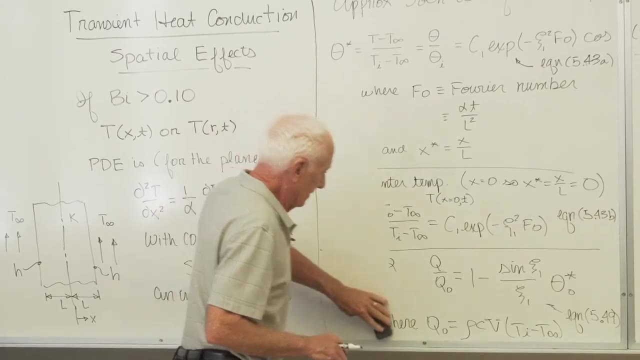 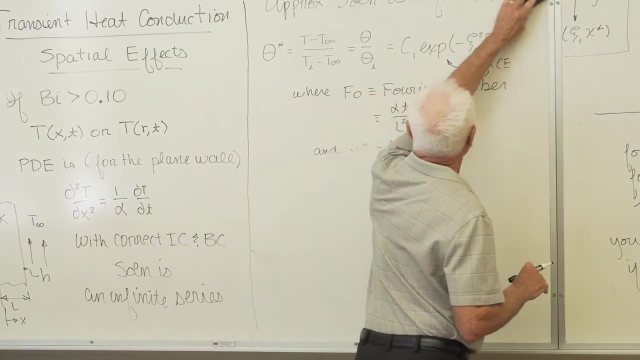 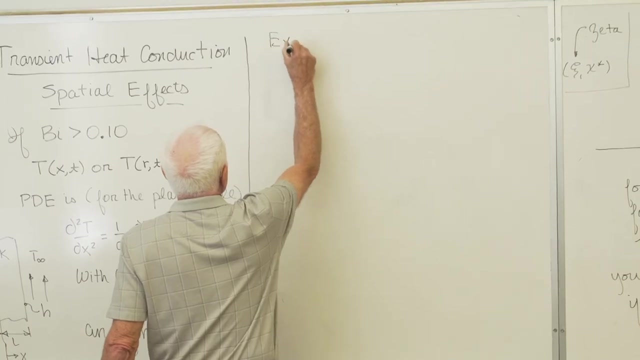 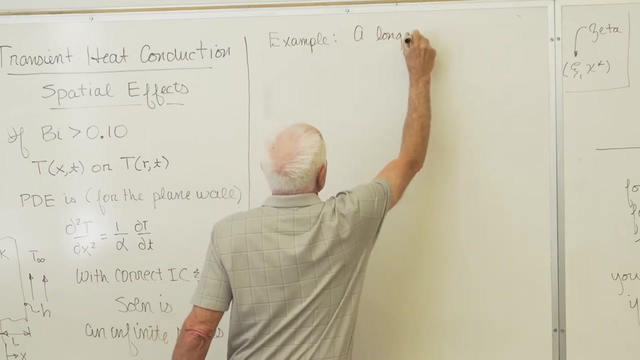 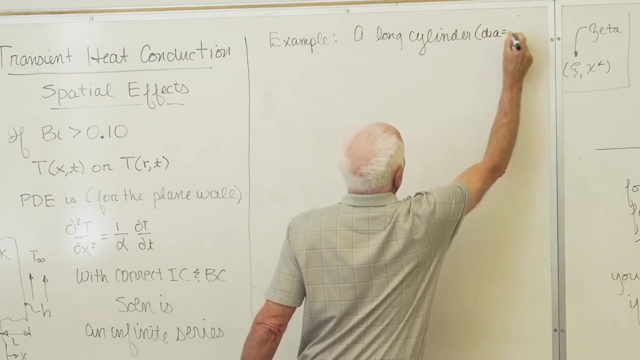 So let's take an example problem and go through all this. We're going to take a long cylinder, All right, So let's erase this. Any questions on this? before I erase some stuff? Okay, Diameter equal 20 centimeters. 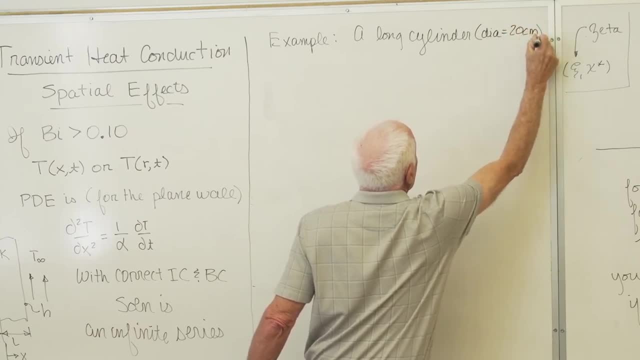 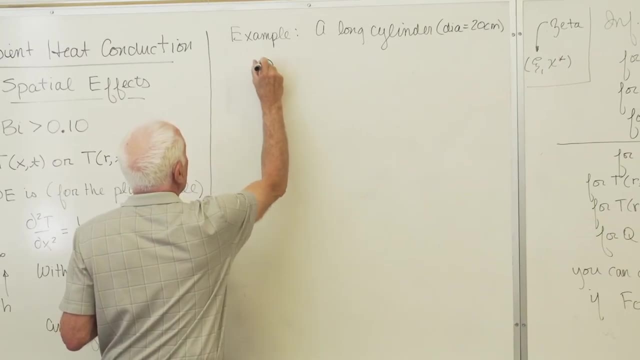 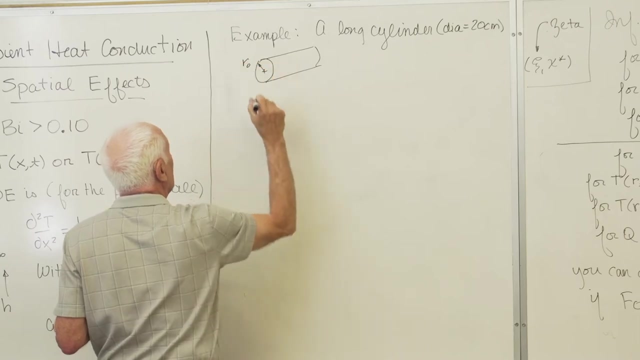 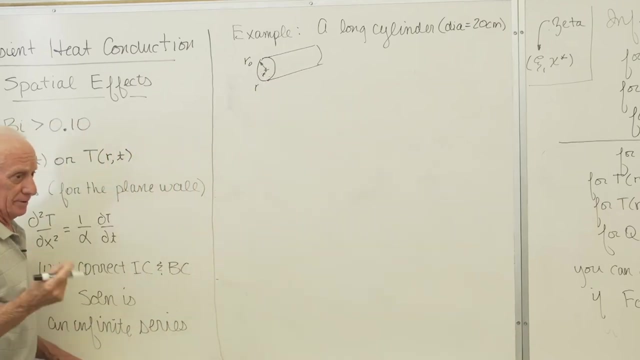 Diameter equal 20 centimeters. Diameter equal 20 centimeters. Okay, So obviously it looks like this: R is the general radius, anywhere from zero to R naught. R- naught is the outside radius. Oh, by the way, the material. 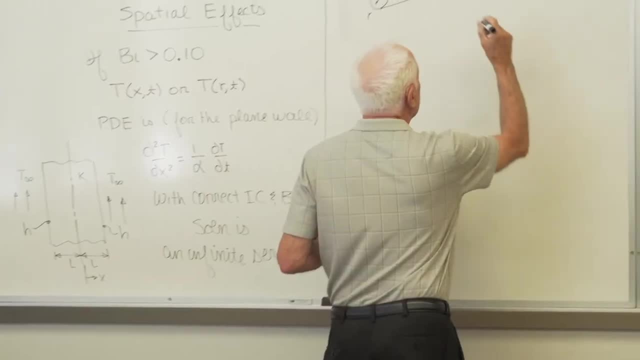 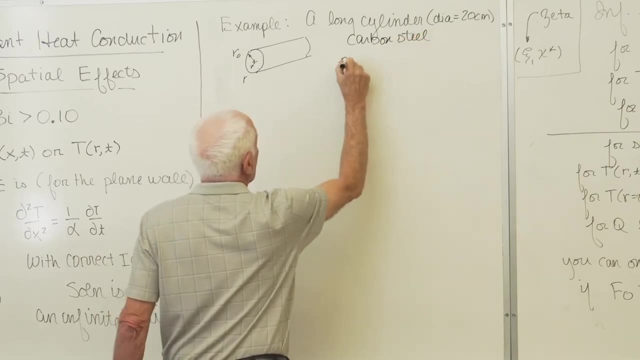 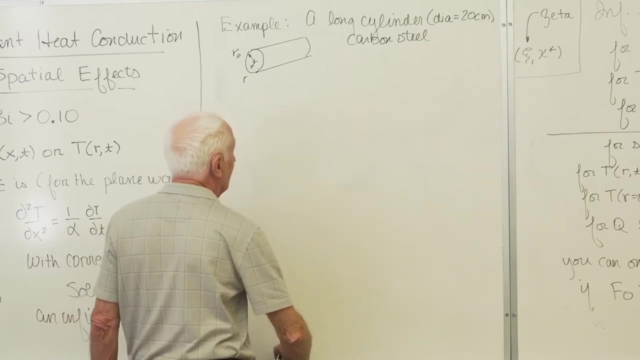 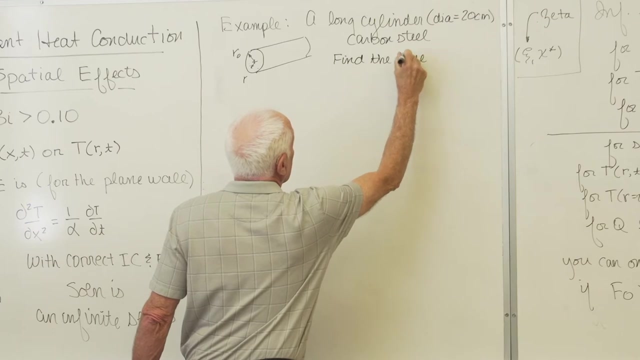 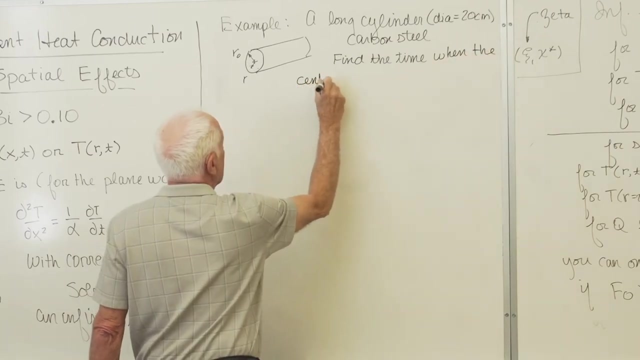 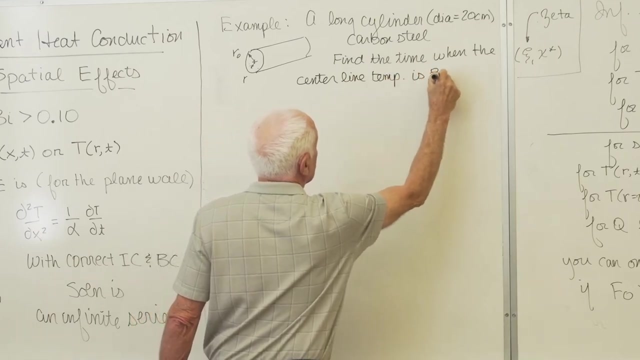 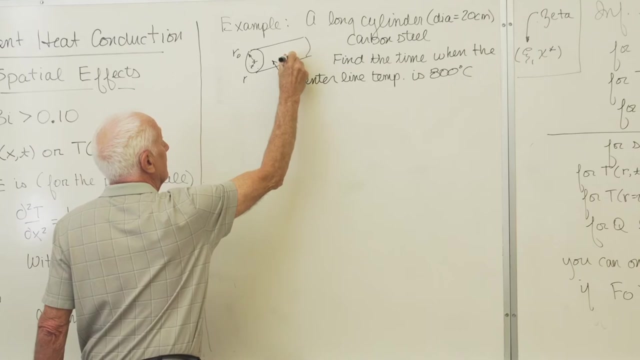 this guy is carbon-steel Properties at. okay, Let me tell you what we're supposed to find. first, Find the time when the center-aligned temperature, let's see, is 800 degrees C. This is 800 degrees. There is air blowing over this at temperature T, infinity. 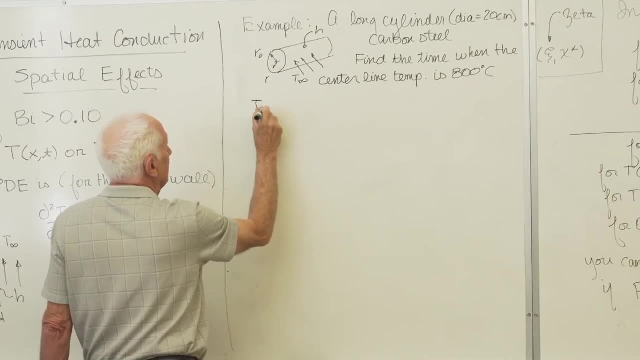 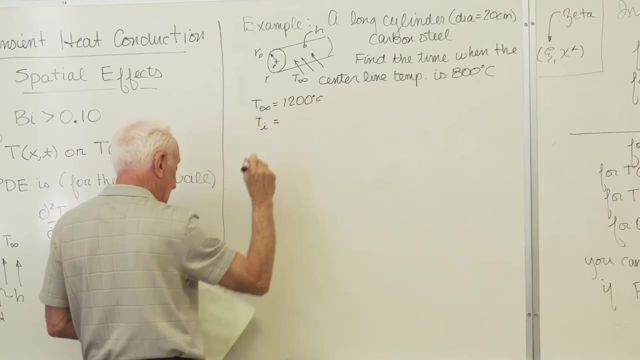 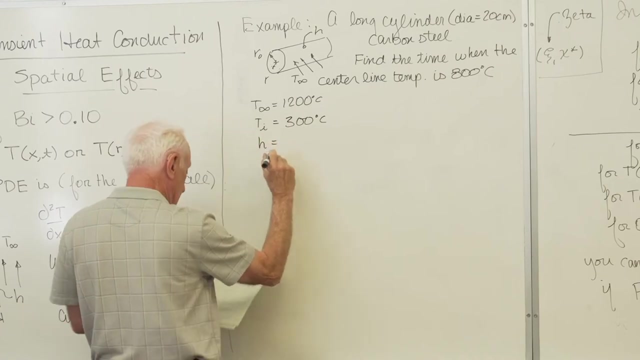 There is a convection coefficient H on the outside surface. T infinity is a hot gas. temperature: 1200 degrees C. We start out with a temperature T. It goes up. Okay, the long cylinder at initial temperature, TI of 300. Convection coefficient is 100. 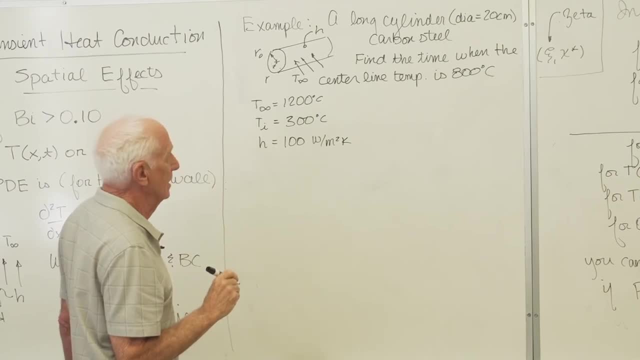 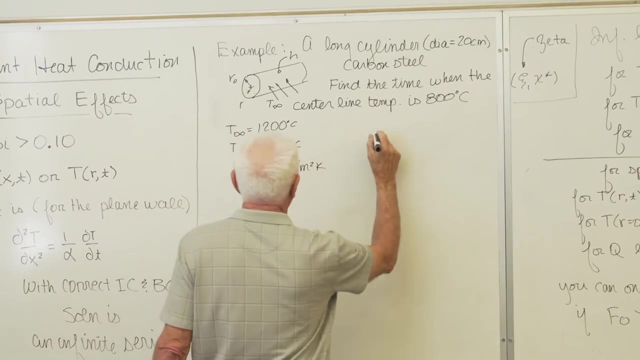 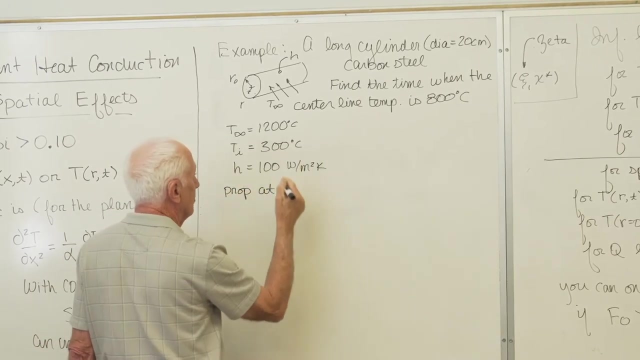 At what time does a centerline temperature get to 800? it started out at 300 in the middle everywhere. Okay, Properties at 300, I'm going to take. it starts out at 300 and the centerline gets to 800, so I'll take that average. 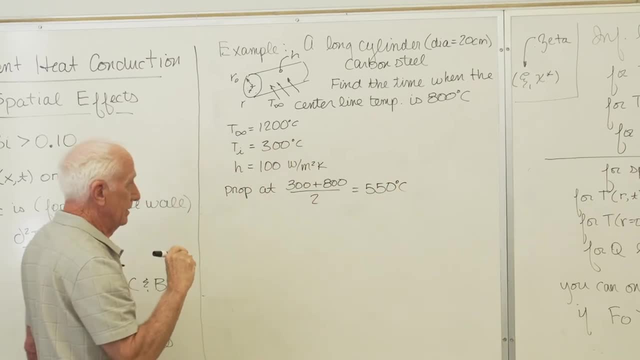 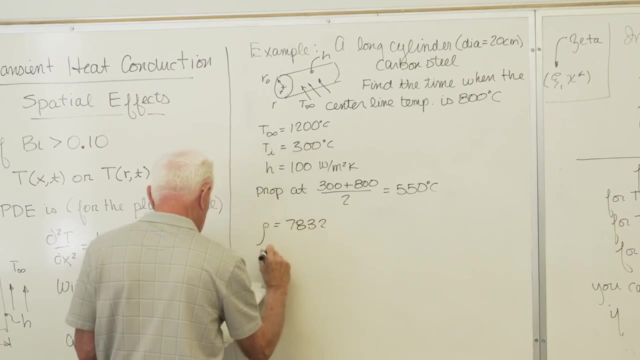 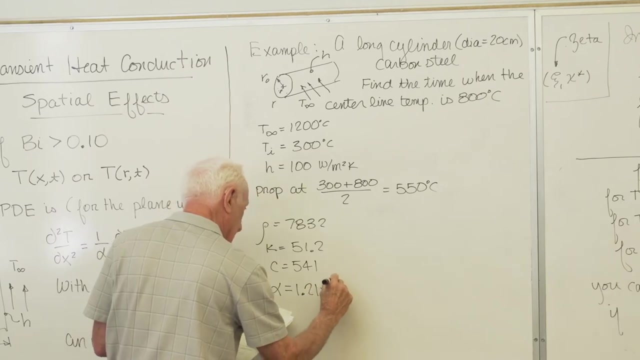 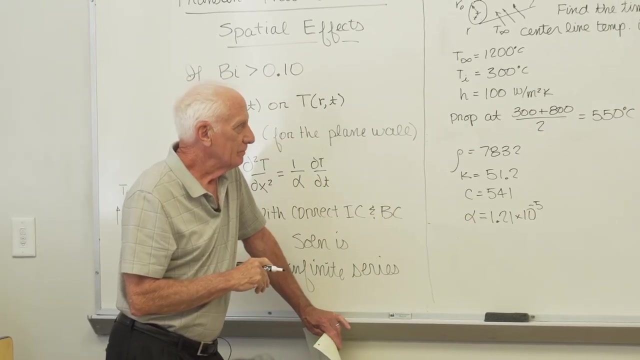 550 degrees C. go to the back of the book. the table fine carbon steel got it. get the density, Thermoconductivity, Specific heat and thermal diffusivity, The properties you know from before. so there are the properties. of course they're correct. Okay, so the Bo number. 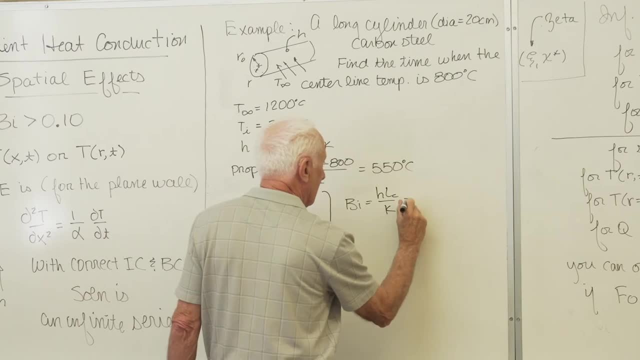 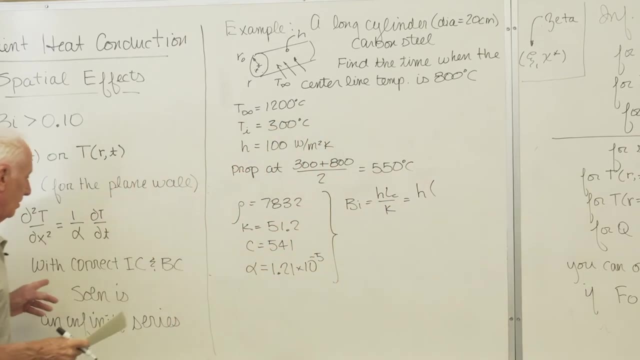 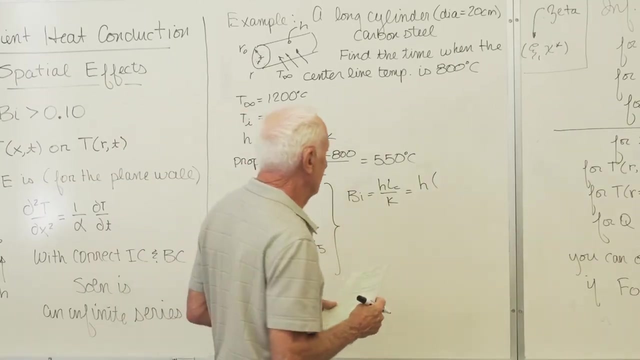 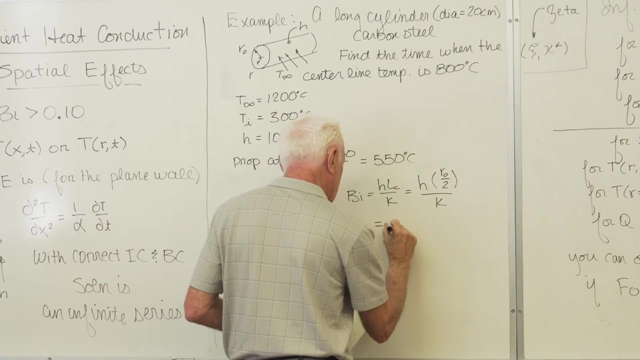 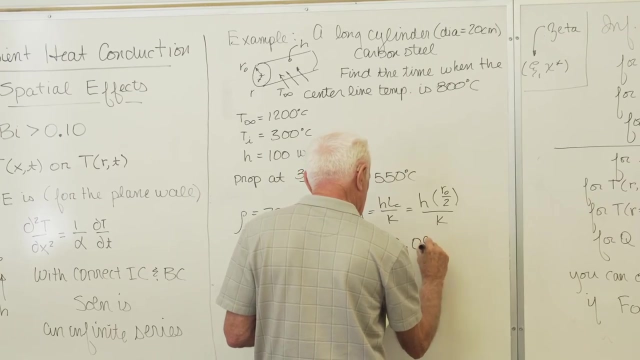 HLC over K For LC. LC for a plane wall is L. L sub C for a sphere are not over 3. L sub C for a long cylinder are not over 2. The Bo number comes out to be Zero point zero. nine seven, six. It's really close to zero, point one. 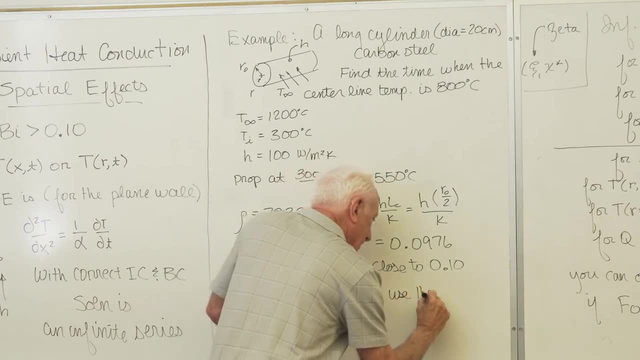 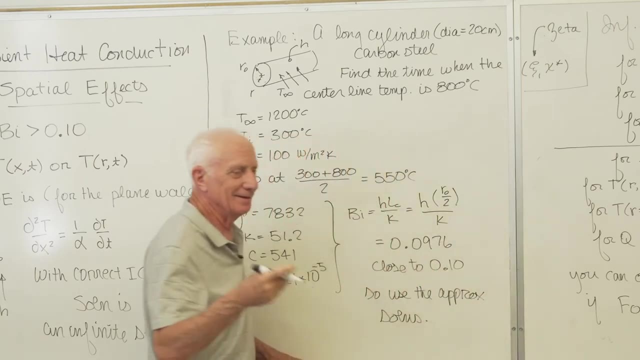 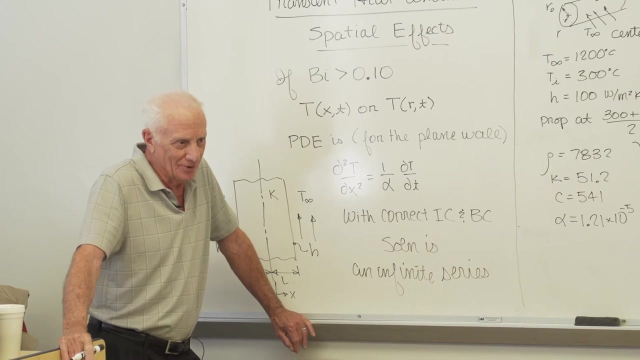 So I'm going to use the approximate solution Now legally. legally I could say: okay, it's less than one tenth, so I can use lump T capacity. I know that's. that's the rule for homework and exams. no matter what, if it's less than 110, go ahead and use lumpy capacity. 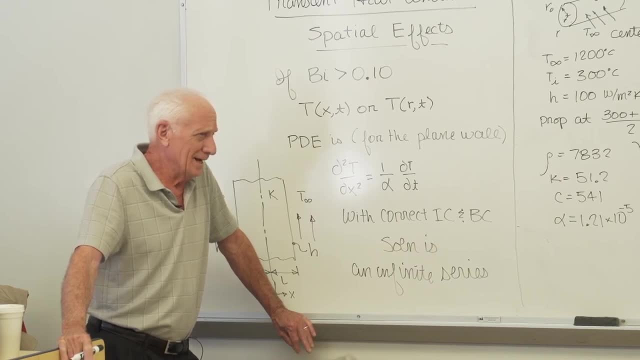 But the closer you get to one tenth, the more inaccurate that model becomes. so I'm just going to say, Okay, we're really close to 0.1.. So I'm going to go ahead and try to use the approximate solutions. Okay, All right now. 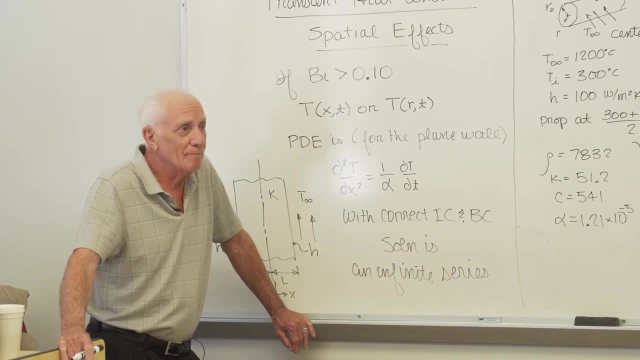 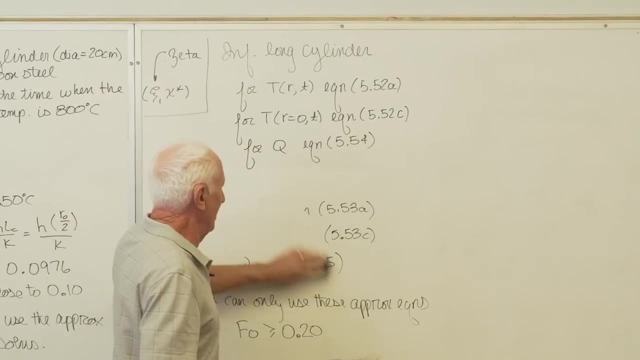 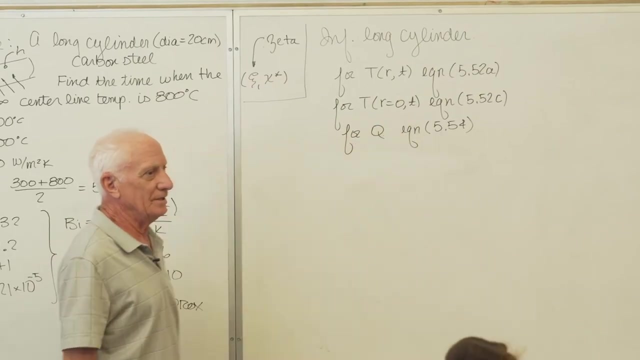 What am I given? I'm given the centerline temperature. Okay, I have three equations. Which equation is for the centerline temperature? okay, Not a problem, I just set it right here. Equation 552 C. so guess what I do? I say: you know what I'm going to use? equation 552 C: okay, 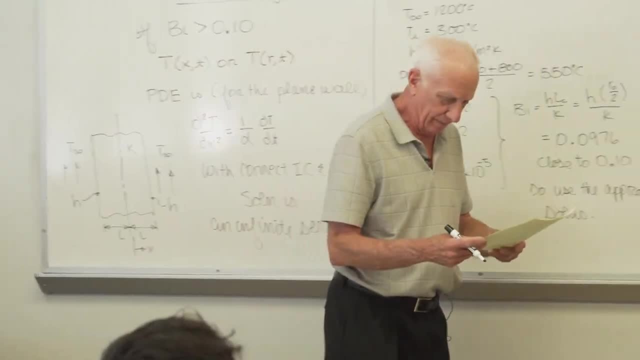 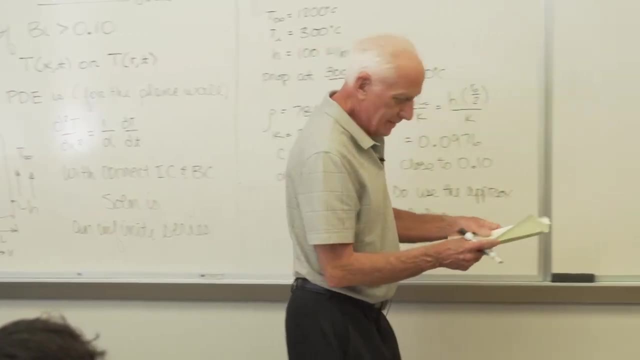 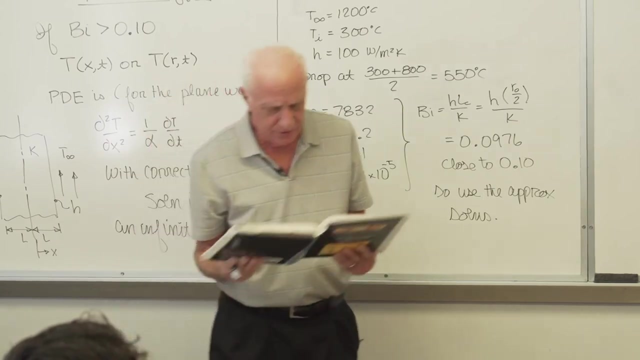 so here's equation 552 C. Okay, let's see where we have that guy here. no, here we are, and I didn't write it down, so I'll write it down on the board for you. Here we are. infinite cylinder. 552 C: Theta naught star. 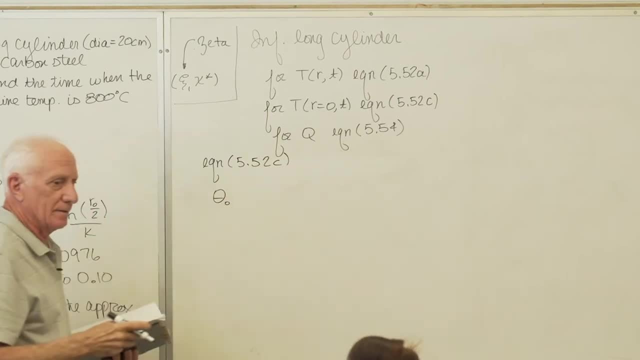 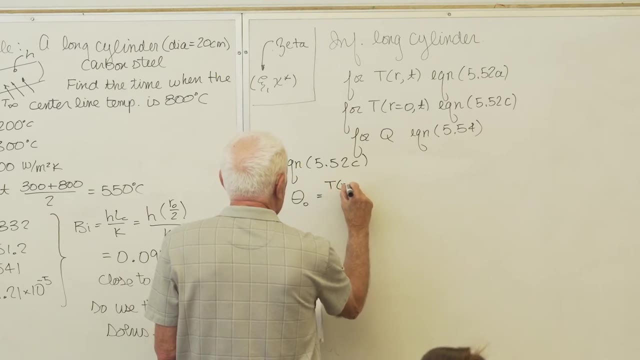 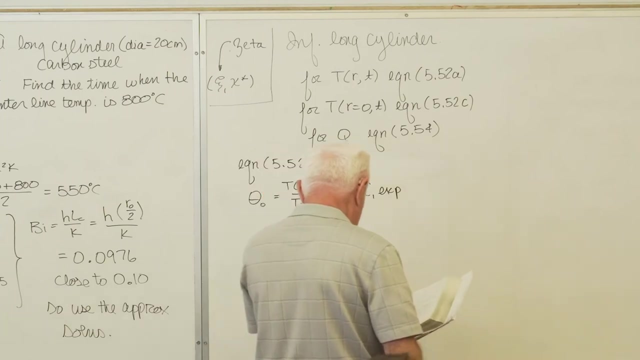 Theta naught. what does the naught mean? Theta naught? centerline temperature: r equals zero T at. r equals zero minus T. infinity divided by T initial minus T, infinity equals 552 C, C1, exp minus Theta 1 squared 4EA. 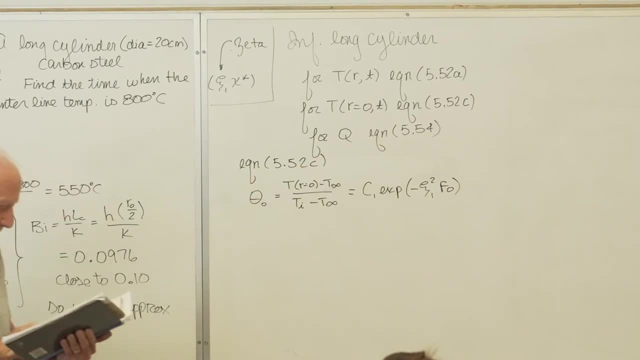 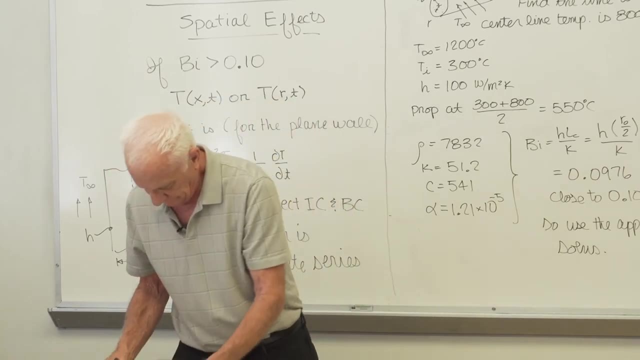 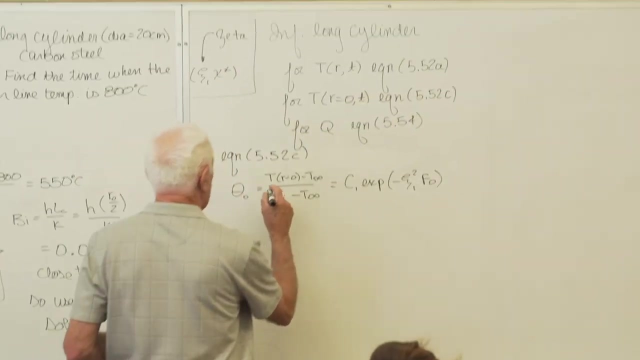 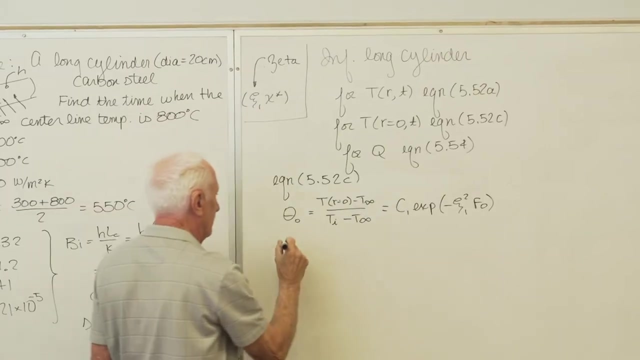 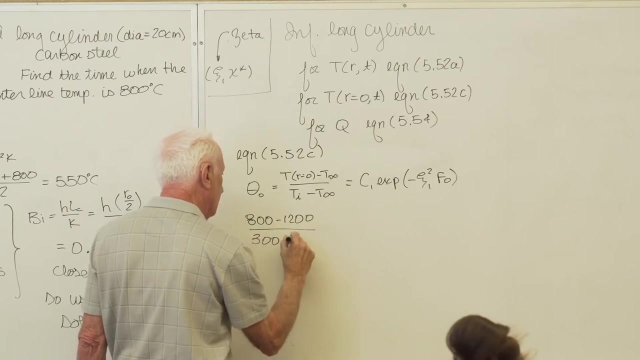 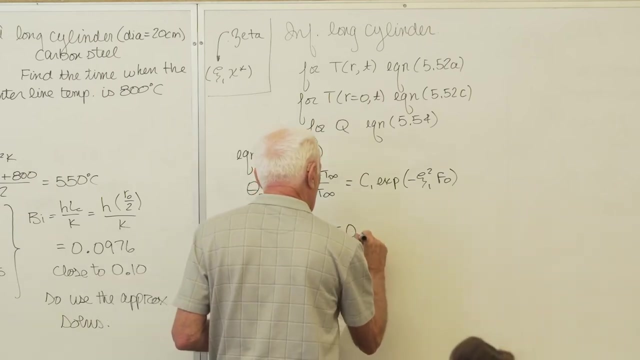 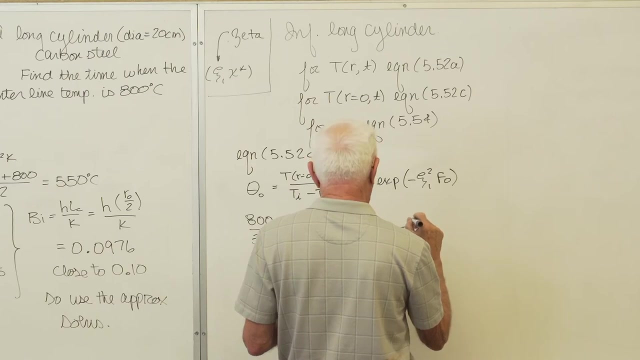 There it is. So let's see what that gives us here then. T at r equals zero. centerline temperature: 800.. T infinity, 1200.. T- initial, 300.. T infinity, 1200.. Zero, 0.444, equal C1.. 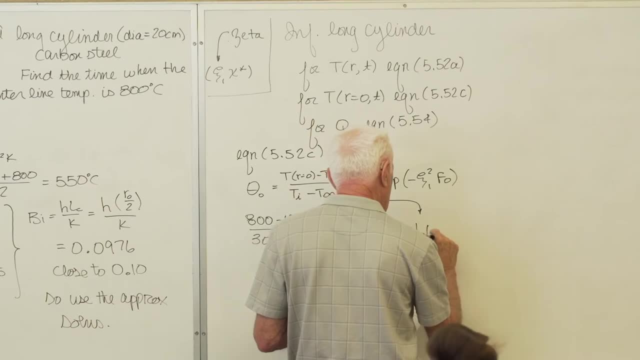 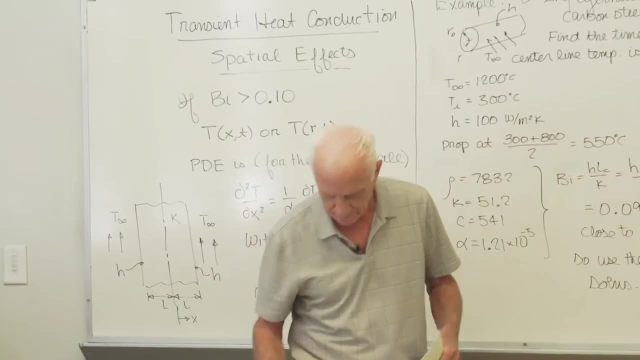 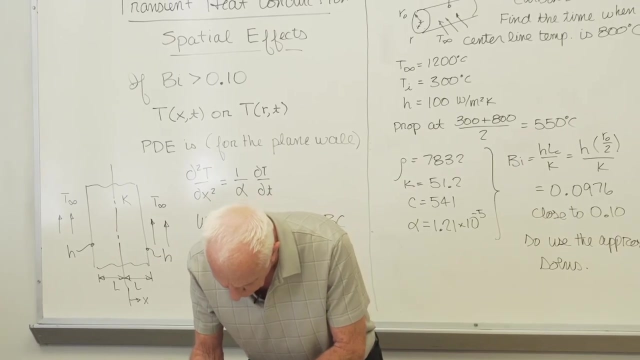 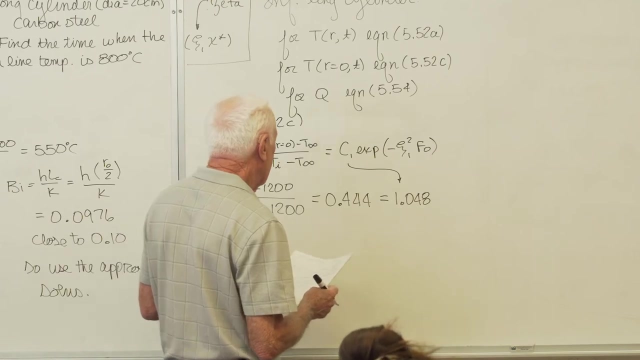 I'm going to put it right here: C1, 1.048, and that's at what was our B0 number 0.1.. Mm-hmm, Yeah, Okay. Times exp minus Zeta 1,. 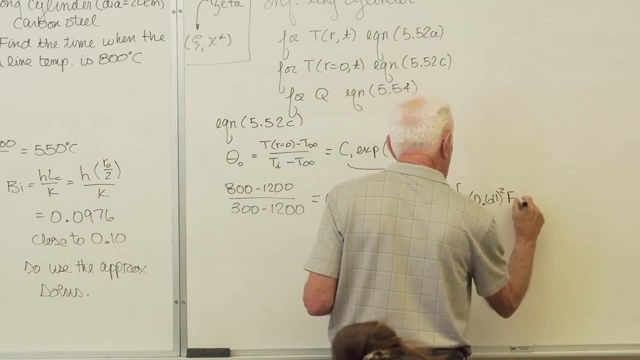 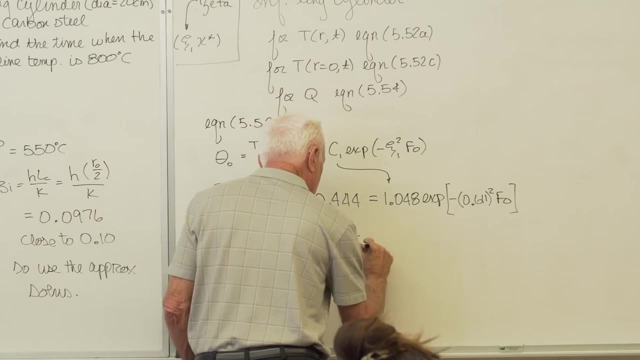 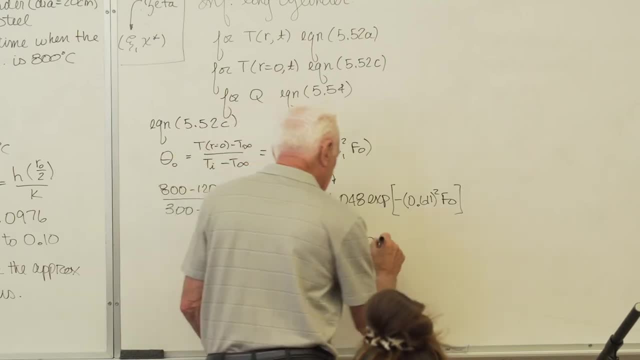 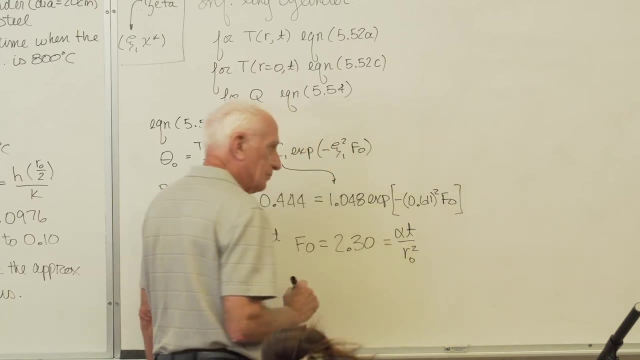 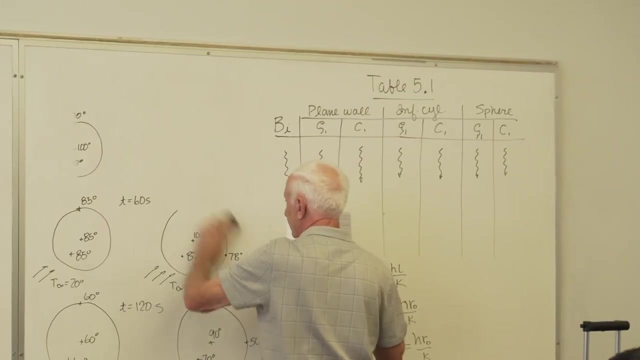 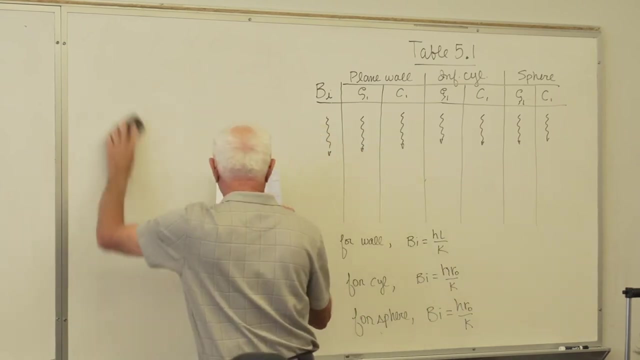 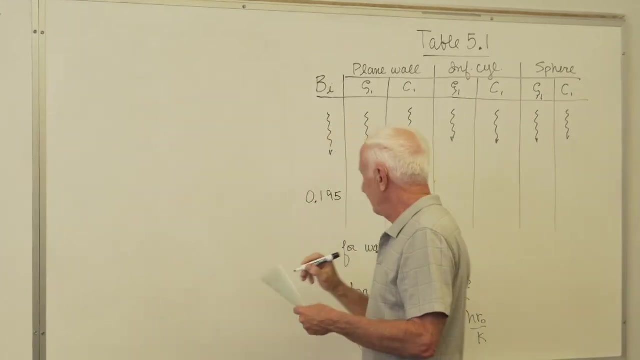 But the 4EA is Alpha T over R, naught squared. All right. so let's see what we have here. Go down here to VO 0.195.. It's really close to 0.2.. Go to the infinite cylinder. 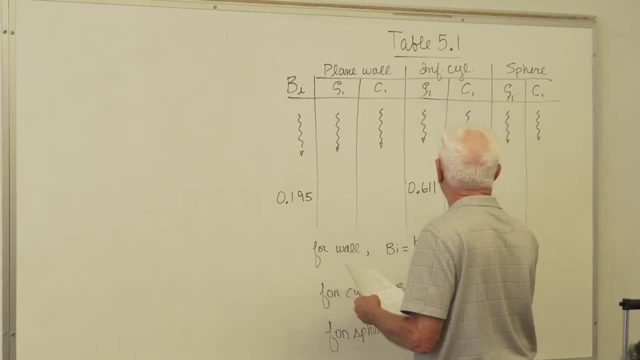 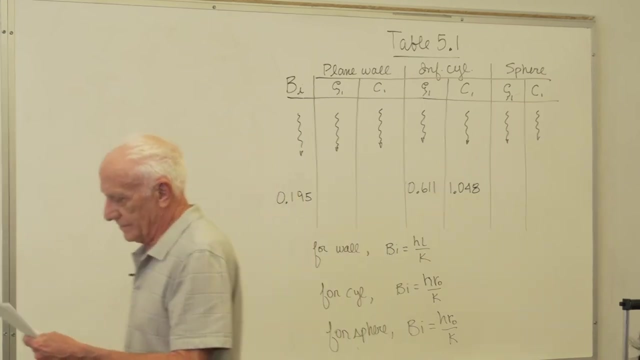 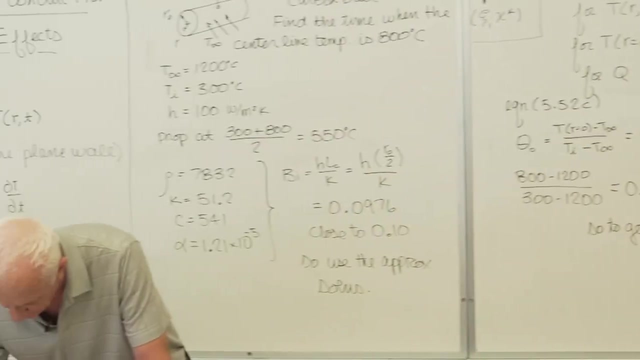 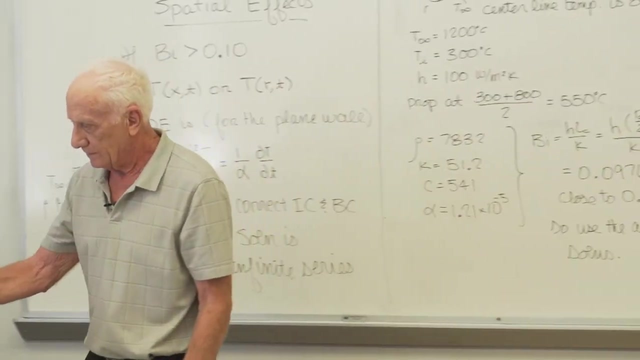 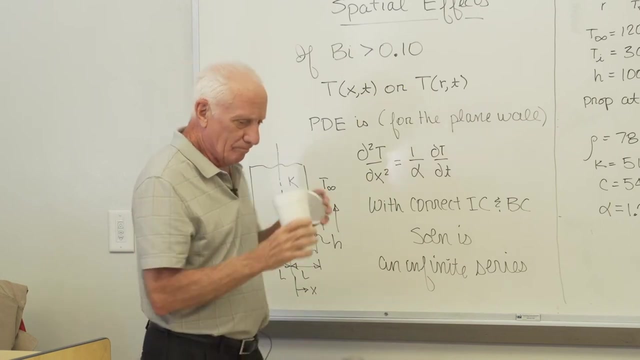 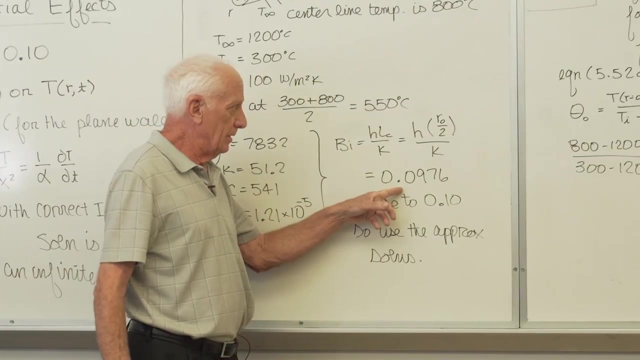 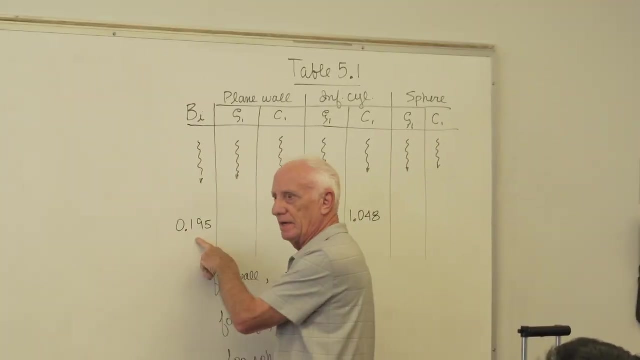 Zeta 1, 0.611, 1.048.. Double-check it, make sure it's okay. Yeah, it's okay. What's the VO number? VO number 0.0976.. What's the VO number 0.195.. 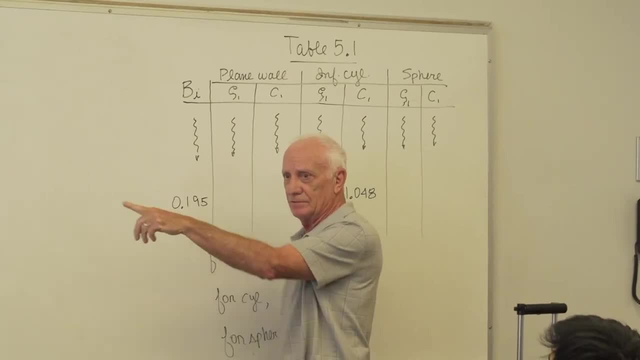 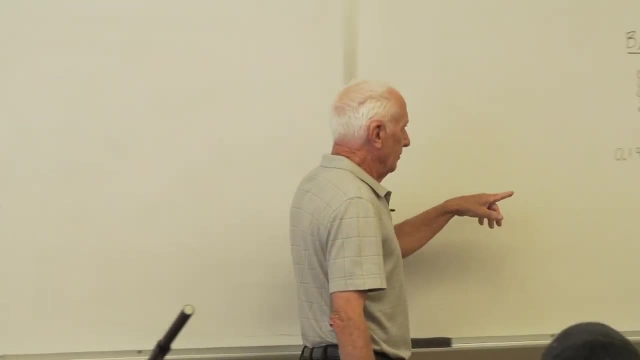 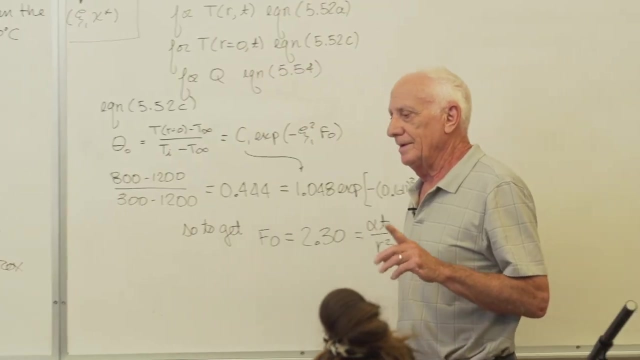 Whoa, wait a minute now. There's two values. What's going on here? Why did I go to the table 0.195, where the VO number should be 0.098?? Well, you got to read the fine print in the contract. 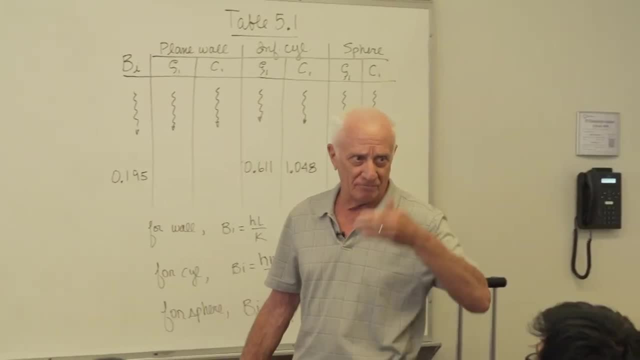 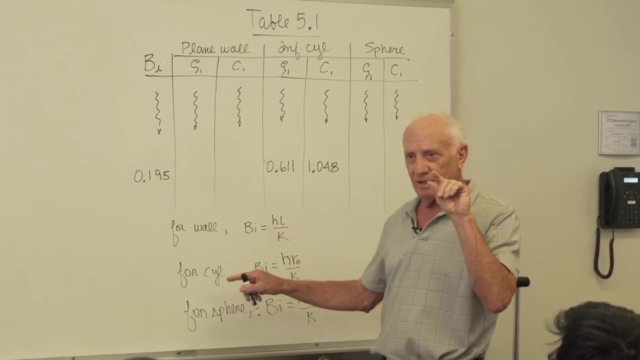 The fine print in the contract is usually at the end of all the fun stuff up front of the contract. Here's all the fun stuff At the bottom of the page in fine print. you got to read a fine print. It says, by the way: 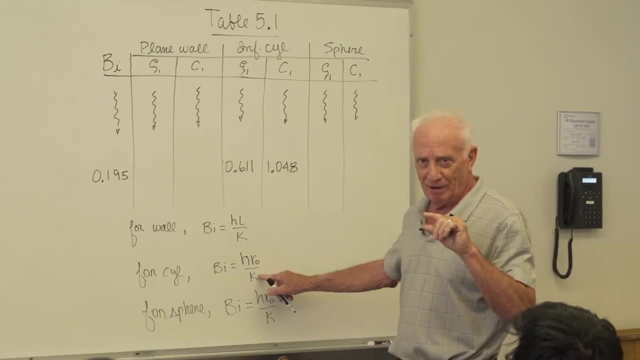 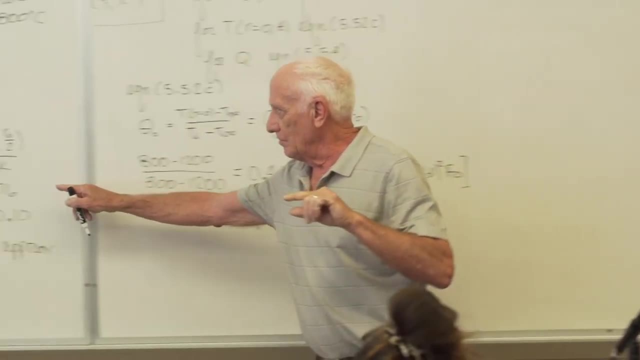 when you're using the cylinder, don't use R naught over 2 for VO number. Use R naught, which means you double it. You double 0.0976 and you get 0.195.. Boy, you better be careful. 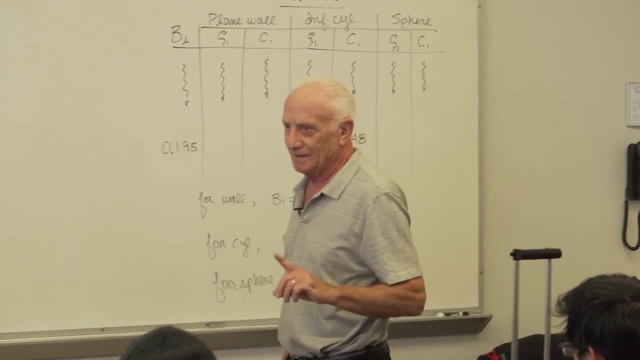 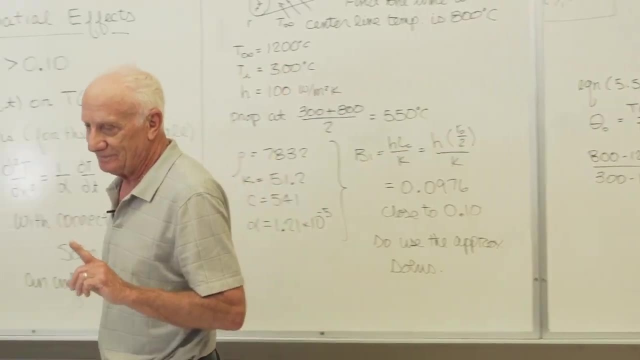 On homework or exams. it's easy to make that mistake. I guarantee it. I've seen it on exams. People in a rush will make that mistake. You got a big yellow highlighter. highlight it. Does it make any difference for the plane wall? 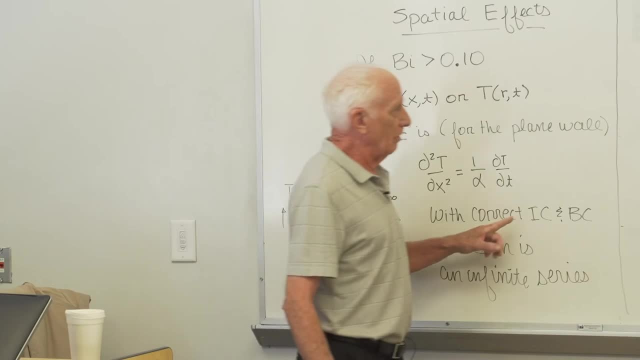 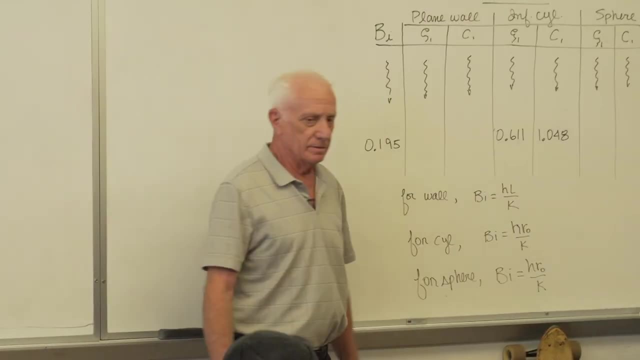 No, it doesn't make any difference. The VO number for a plane wall is HL over K. The VO number over here for a plane wall is HL over K. What's the VO number over here to check? one-tenth for a sphere. 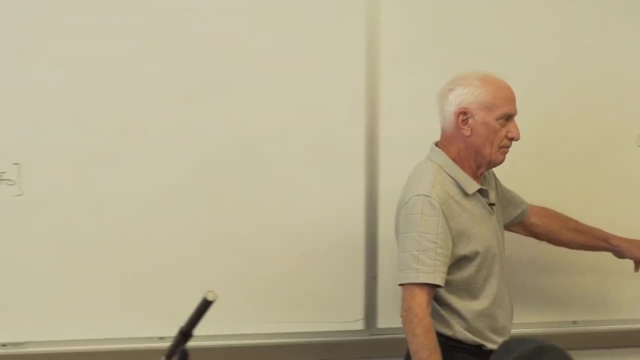 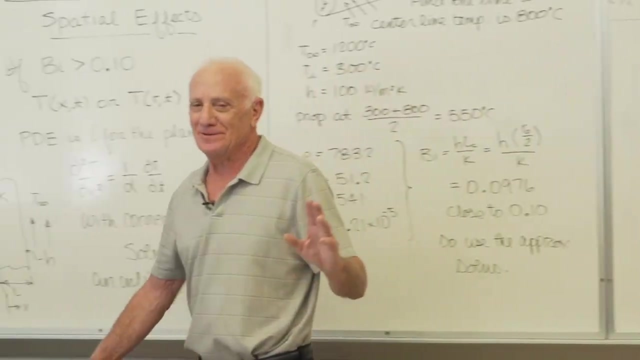 R naught over 3 over here for a sphere. Don't put the 3 in there. it's just R naught, So be careful. There's reasons for that, but I'm not going to go through all those great reasons. 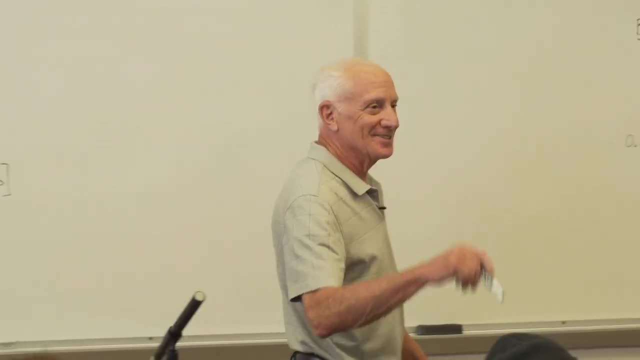 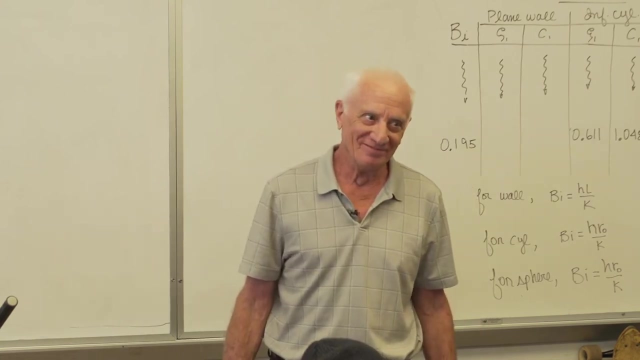 It takes about 10 minutes to describe it. Why did I do that? Yes, sir, So the VO number we used to check would be the actual one. Yes, that's right. What's the actual one? Over 2 and over 3.. 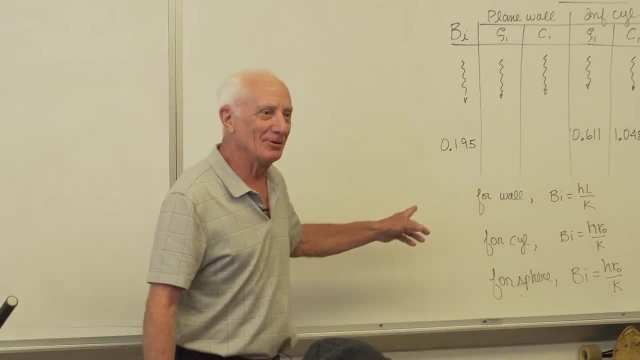 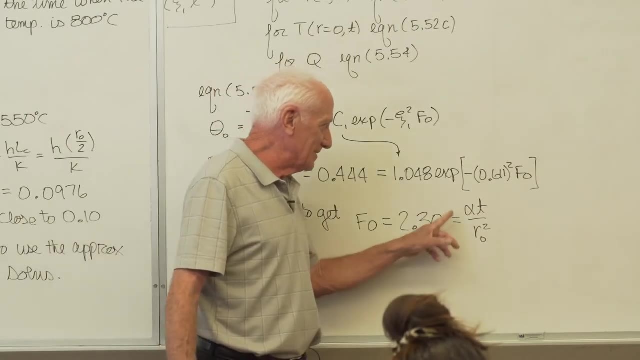 The R naught over 2 and R naught over 3.. Yes, exactly, Only when you use that table there. Now here's another thing, since you mentioned that too. The book says: Fourier is alpha t over L squared. That's for a plane wall. 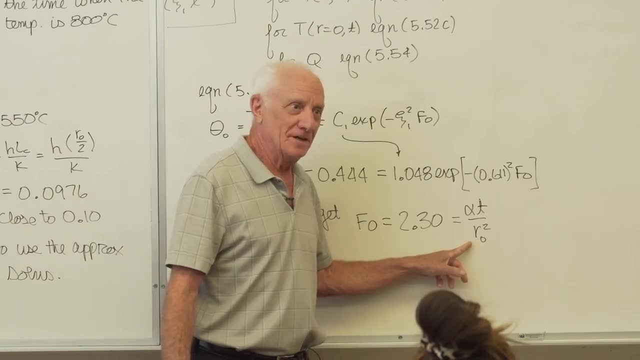 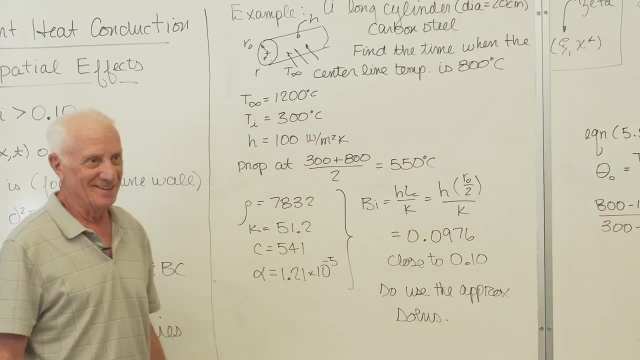 For a long cylinder, it's R. naught. For a sphere, it's R naught. The only time you put that R naught over 2 and R naught over 3 is when you check the VO number there. That's it, Just a big red flag. 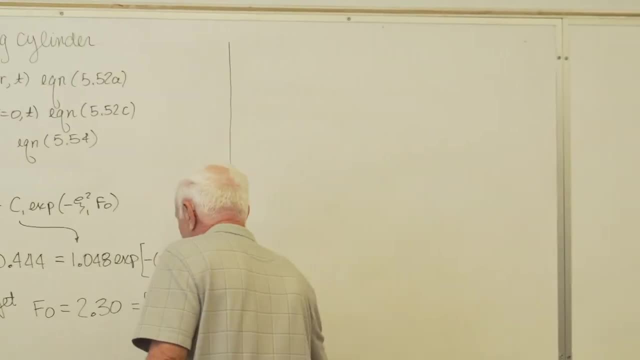 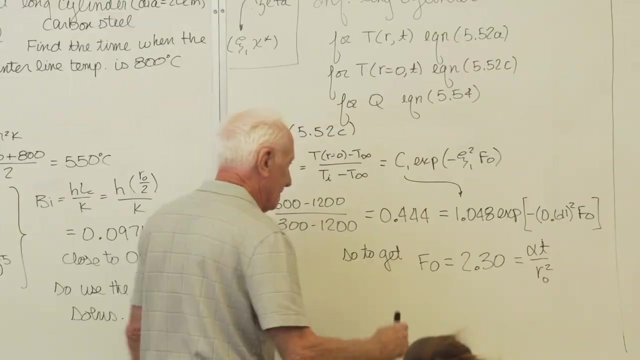 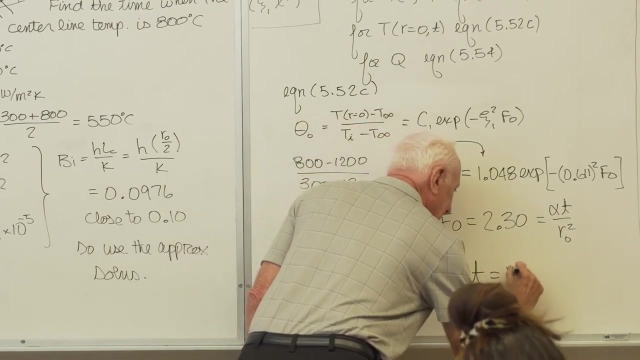 be careful. that's all Now. solve for t. I know alpha, alpha. Yeah, there's alpha, I know alpha. I know R naught Solve for t. t equal 1,900 seconds. So after 1,900 seconds. 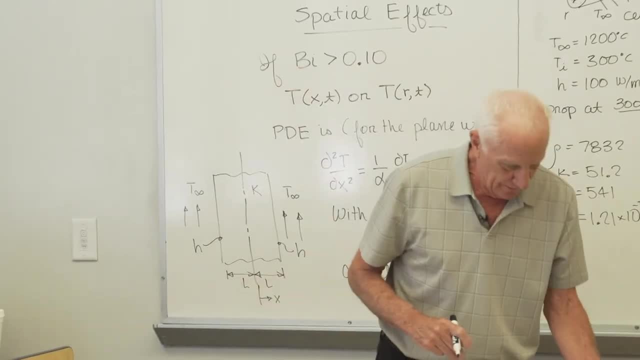 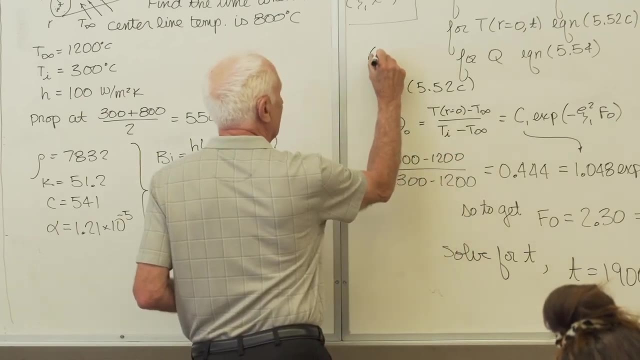 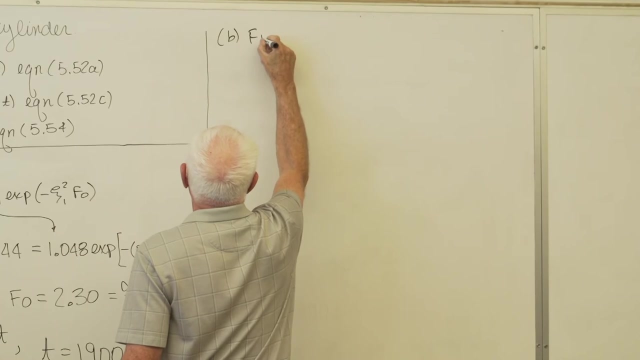 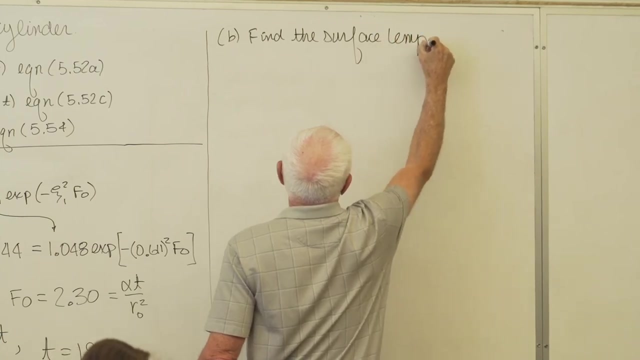 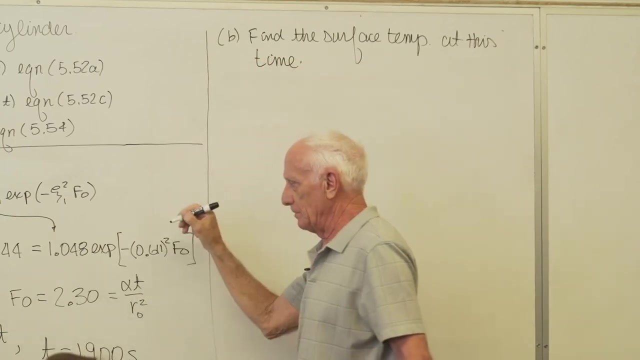 the center line temperature is 800.. Now, that's Part A. Did I put Part A down? I didn't put Part A down. It's okay. Part A. Part B: Find the surface temperature at this time. What's the surface temperature now after 1,900 seconds? 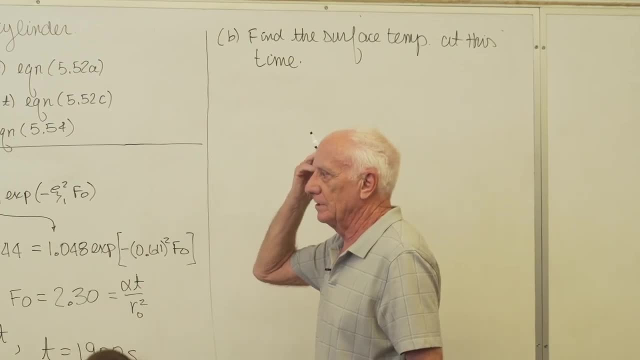 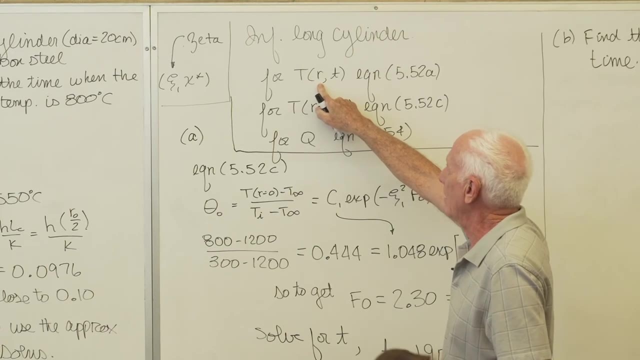 Here's your decision. What do I want? Surface temperature: Where's that? R equal R naught Here. R equal R naught. I got to put R naught in there. What equation do I use? Not a problem. 552A. 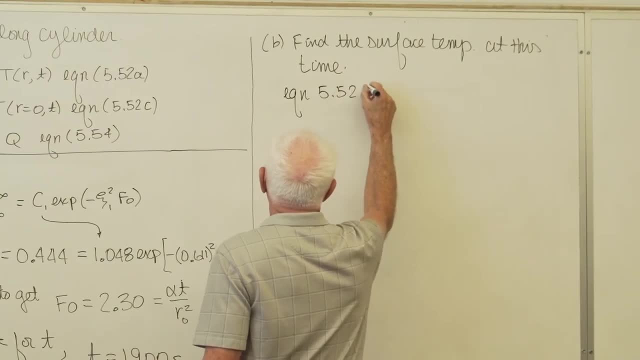 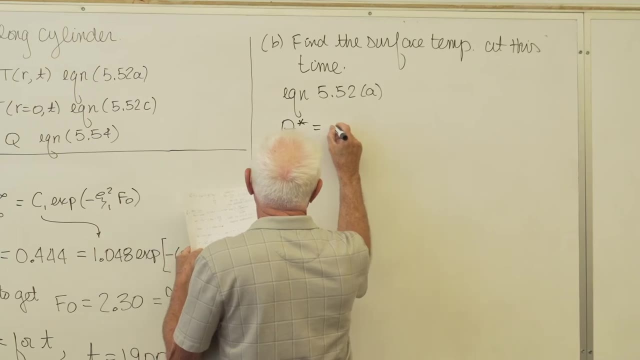 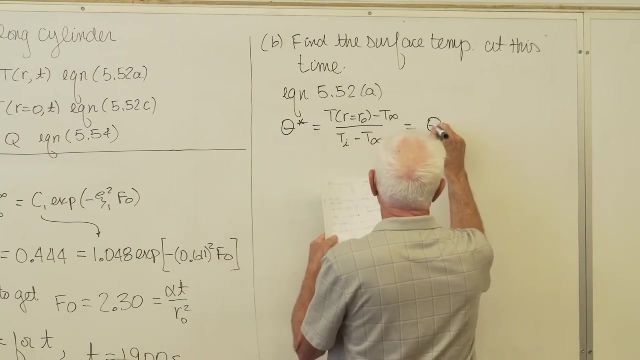 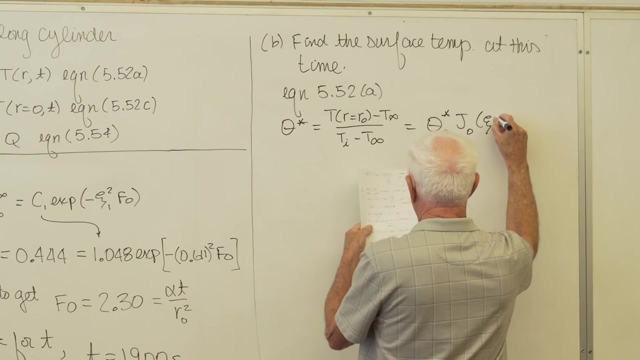 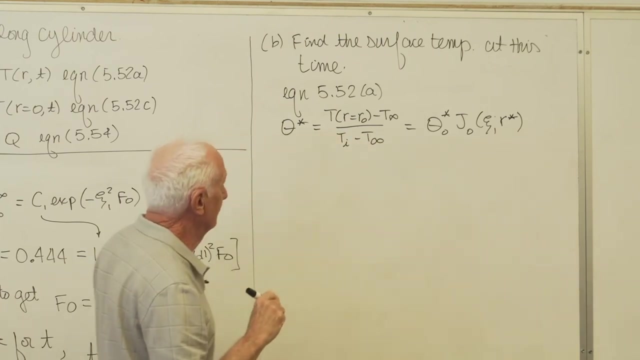 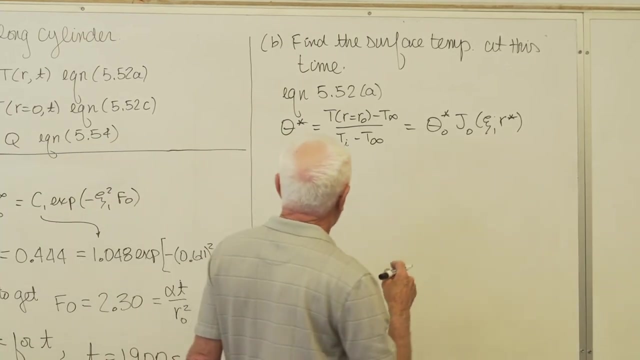 Okay, Here's 552A Bessel function, Bessel function. Okay, Bessel function. Bessel function, Number 1.. Well, I want to solve for that guy. Temperature R equal R, naught. What's this guy right here? 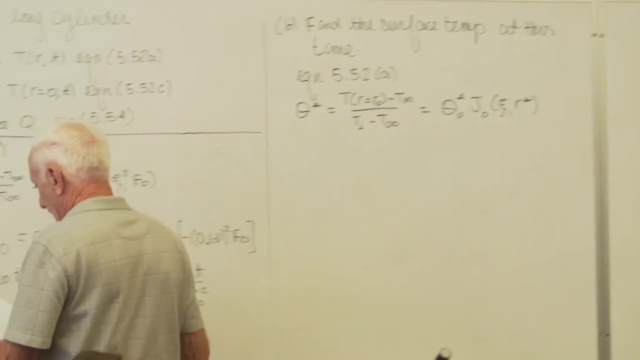 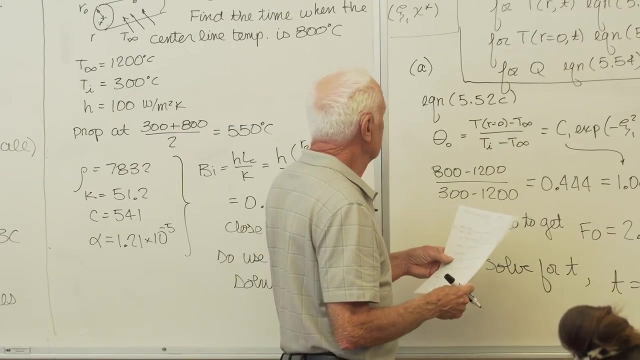 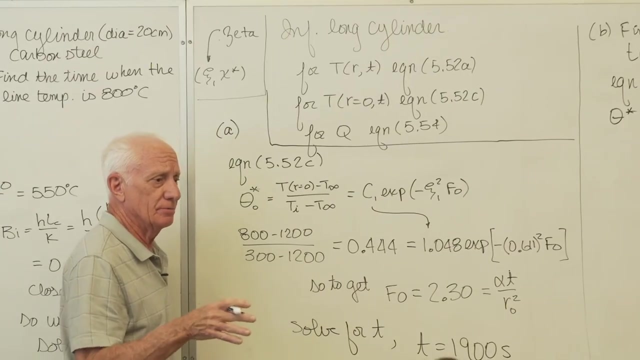 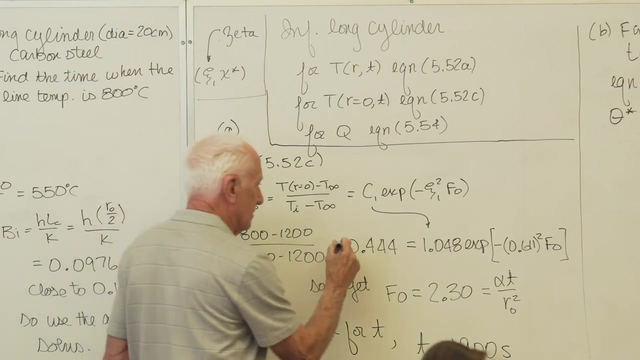 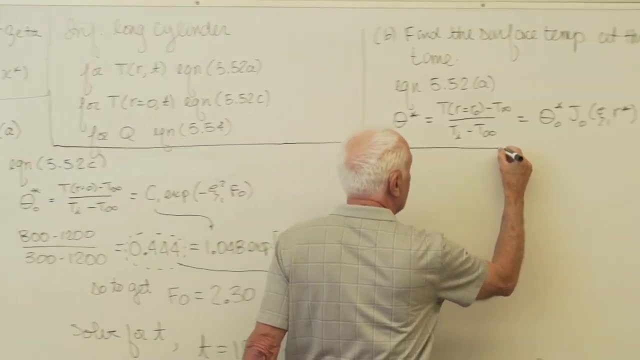 Okay, This guy, Theta naught star. Let's see, Theta naught star. That should be a star, pardon me, Star always means divided, a ratio. That's what the star means. Okay, There it is, He goes in there. I've already found it. 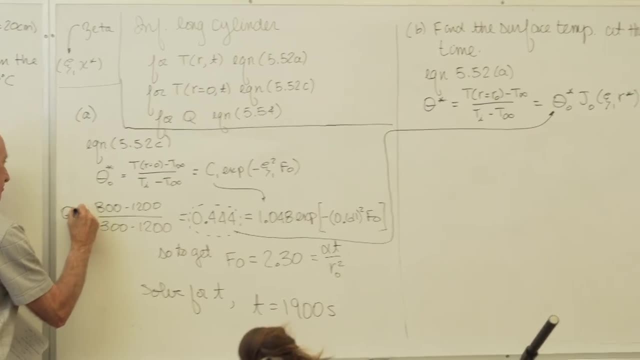 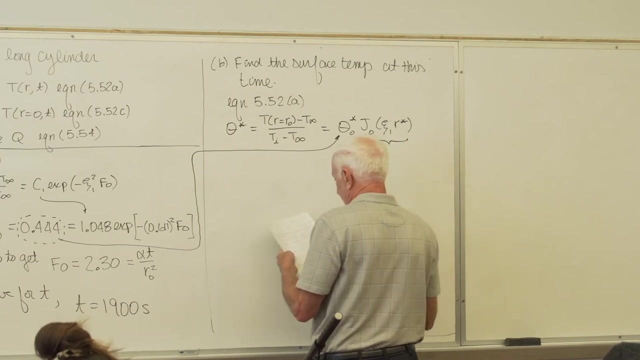 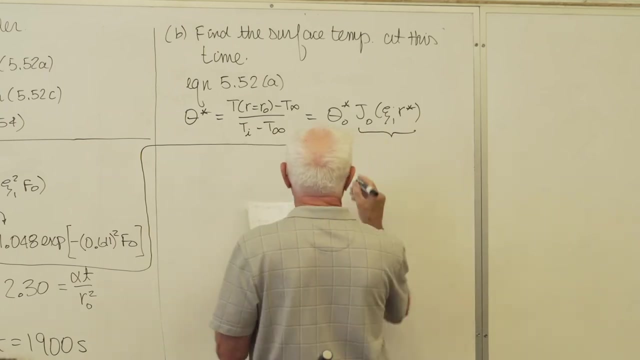 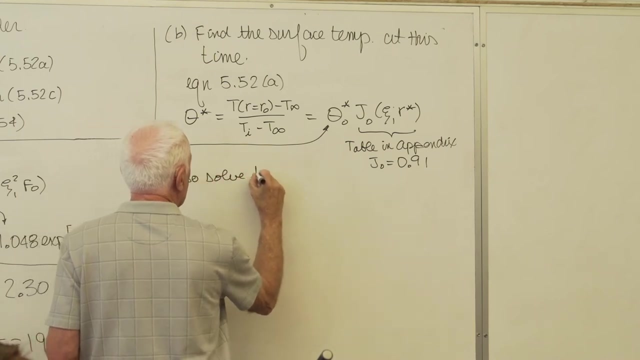 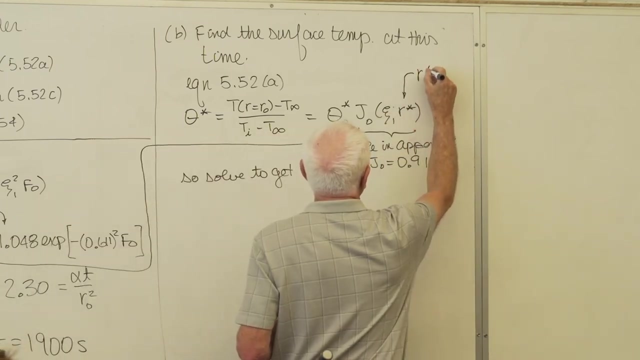 Theta naught star. Okay, Got to go here and find this guy. Okay, That is in the table from the table back of the book 0.91.. So solve to get: oh, by the way, R star equal R over R, naught equal R, naught over R, naught equal 1.. 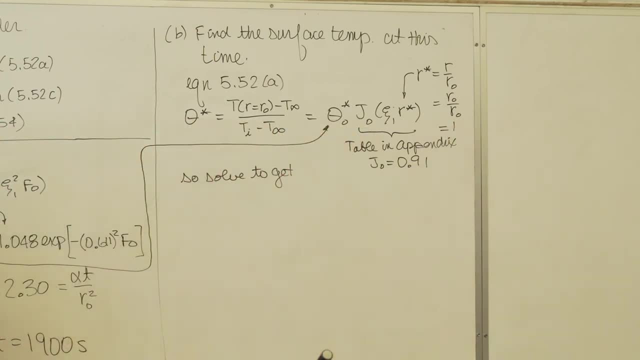 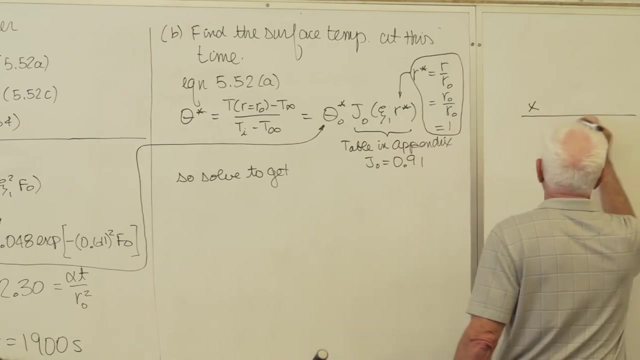 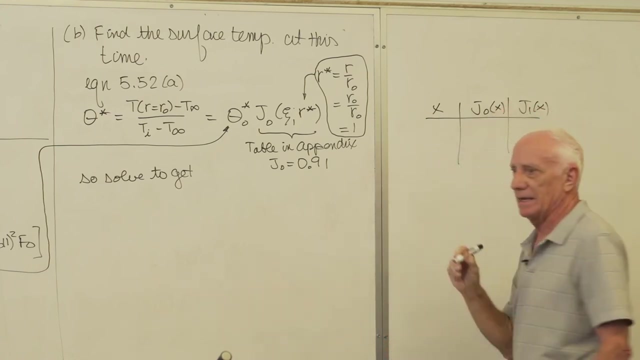 So R star is 1 at the surface of the cylinder. So I go to the table. Here's what the table gives you. That's what it says. That's exactly what the table says. X. You got to figure out what X is. 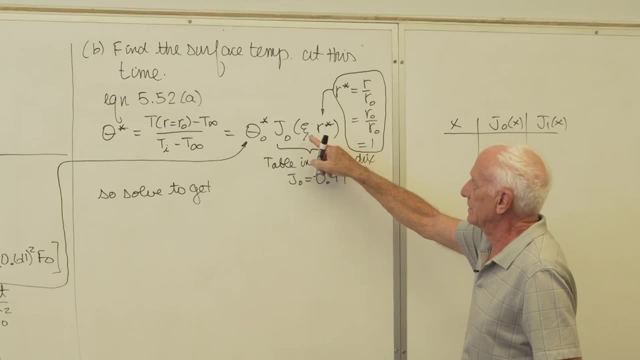 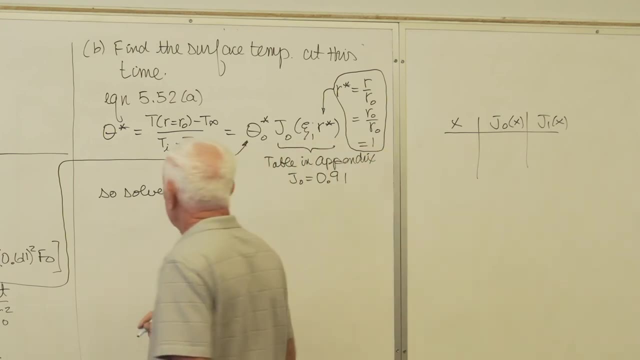 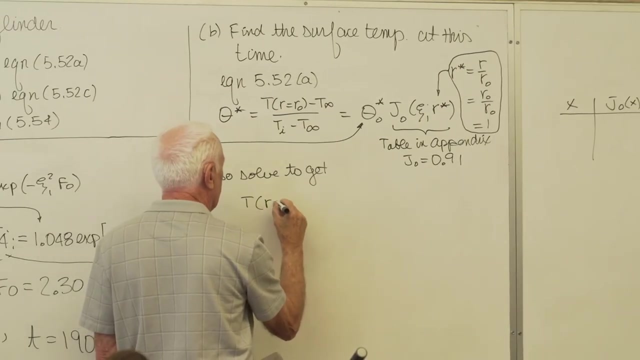 X is Zeta 1 R star. X is Zeta 1 R star. Okay, Now put that in there and solve to get what Solve for the temperature at the surface: 8.3.. 8.3. 8.3.. 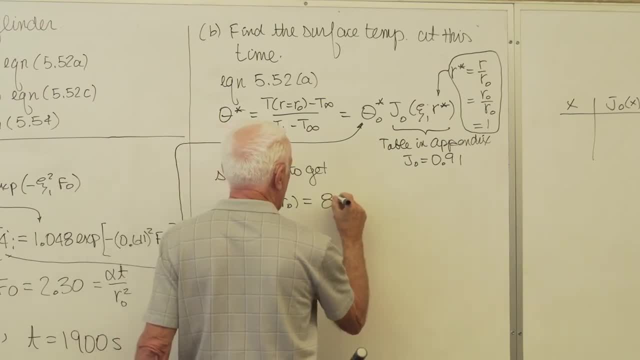 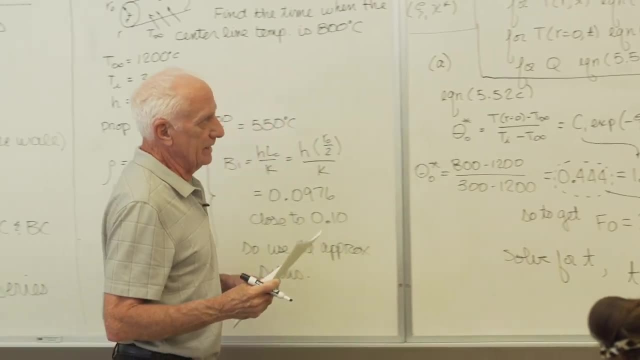 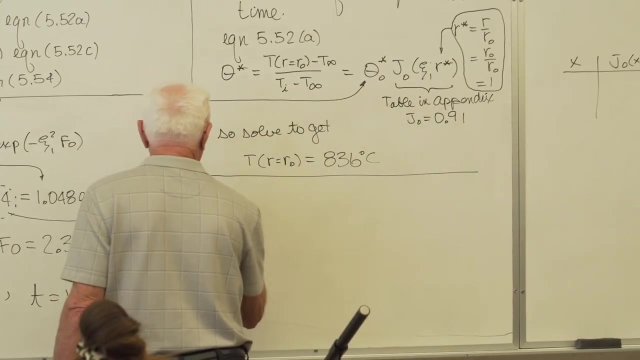 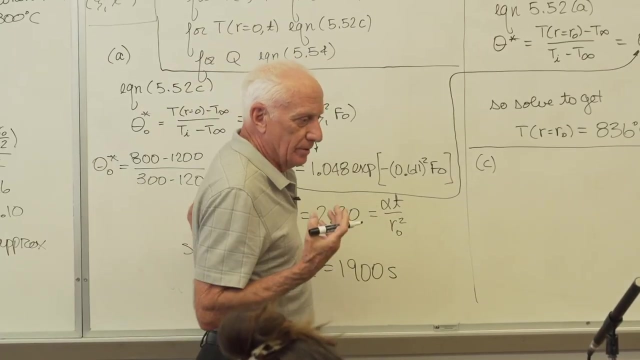 8.3.. 8.36 degrees C. So after 1,900 seconds the temperature of the surface of that is 8.36 degrees C C. How much energy has been transferred to the cylinder from the hot gases? 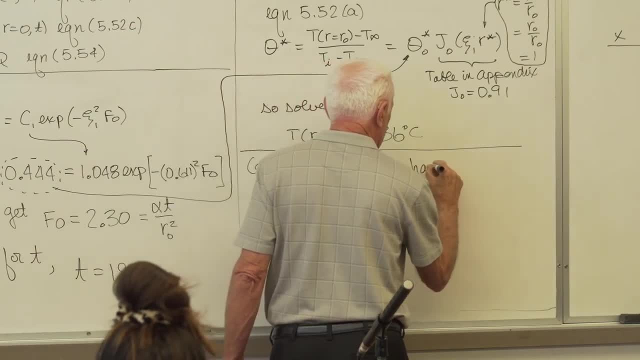 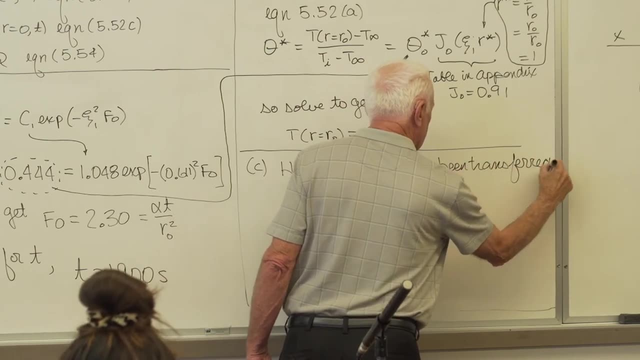 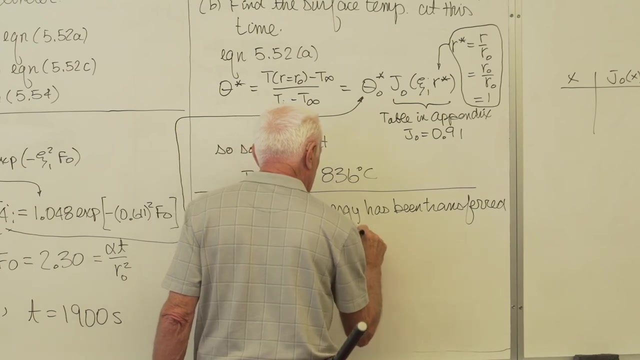 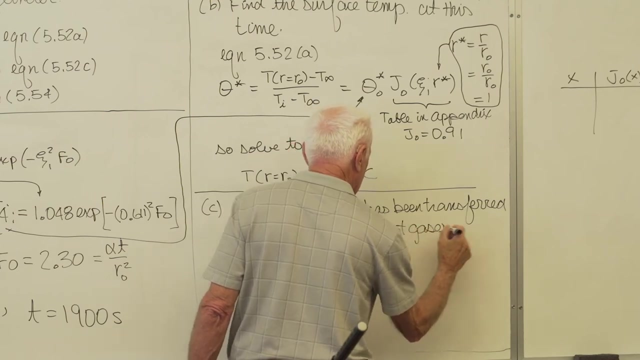 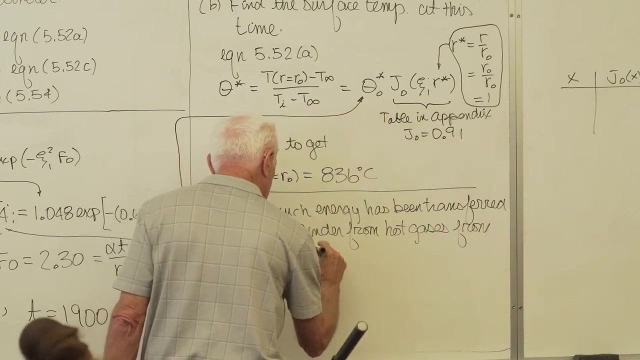 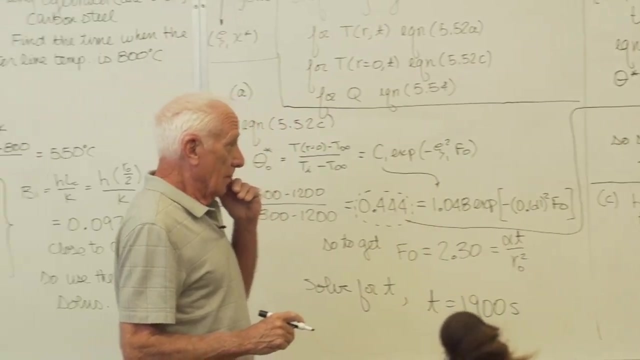 potato 5. tror Yeah, So now you know Big me, I think it's roots. Big me, Big me, Big me. Okay, that's the question. Okay, back to our three equations. Only have three equations B. your number is greater than one-tenth. 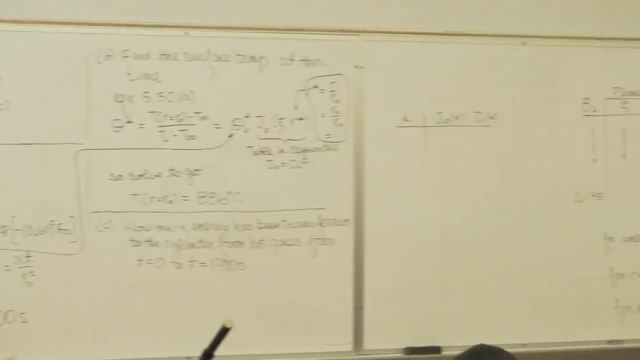 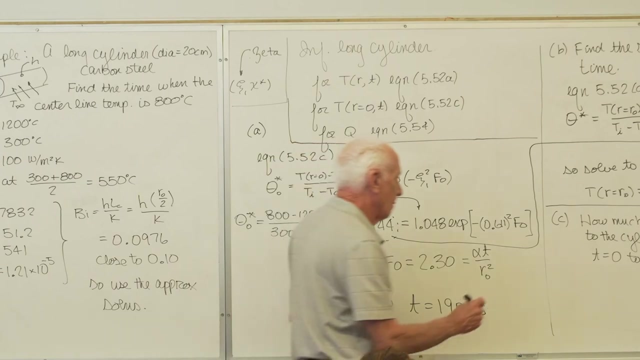 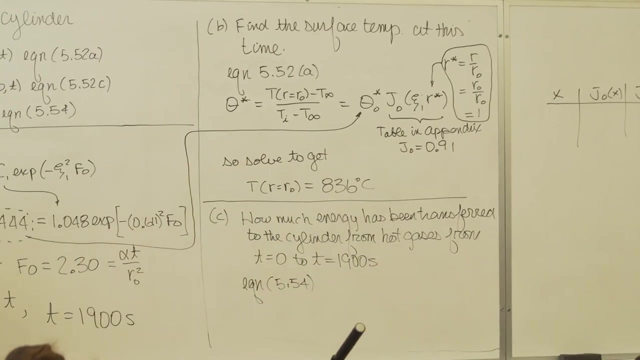 There are three equations you can use to solve for things: Center temperature, off-center temperature, Q. I'm going to solve for Q, energy. Okay, equation 554.. So 554, it's a ratio Q over Q naught. 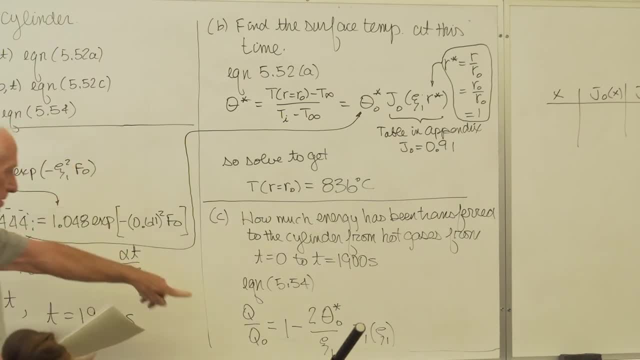 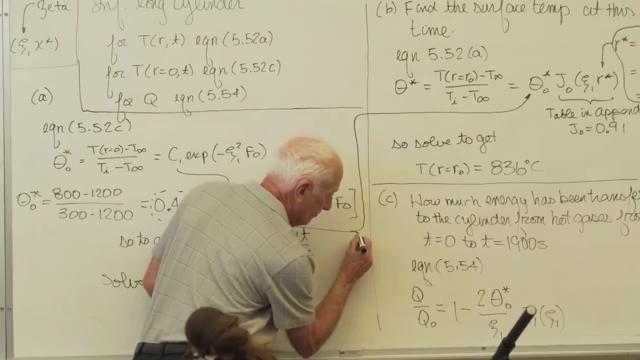 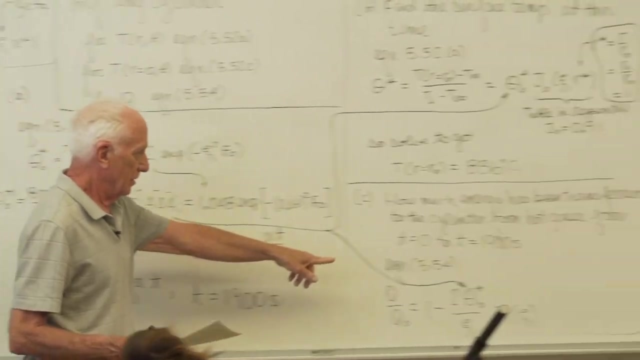 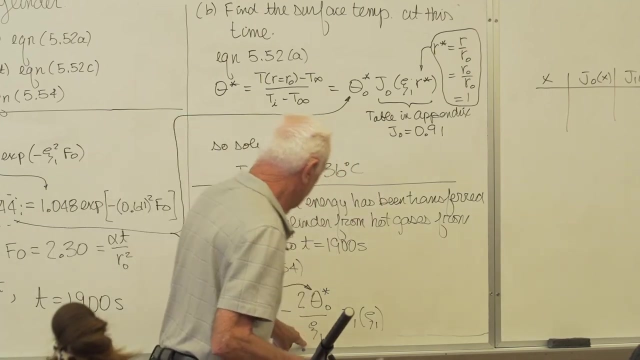 That's an equation 554.. Theta naught star. here it is. Put it in there: 0.444.. Two times 0.444 divided by Zeta 1, 0.611.. Yeah, J1 of Zeta 1,. 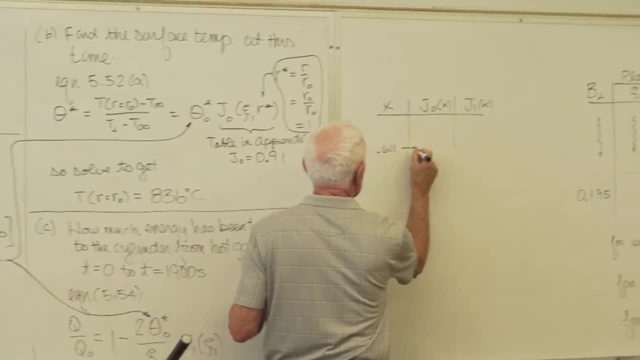 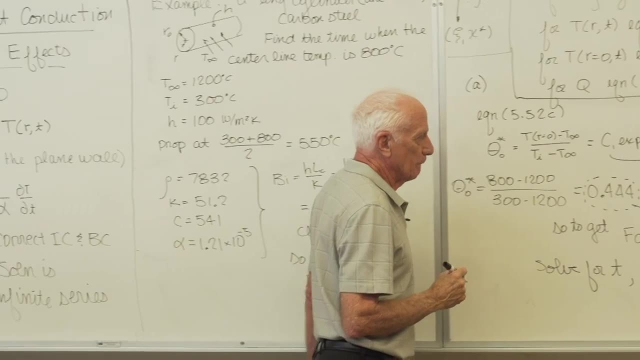 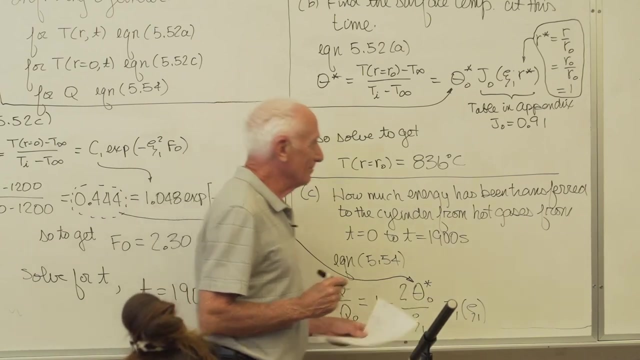 go here: 2.611.. Get J naught, get J1.. That's how you do it. Now this guy here, see, there's a Theta naught and there's a Q naught. Okay, now I'll get Q naught. 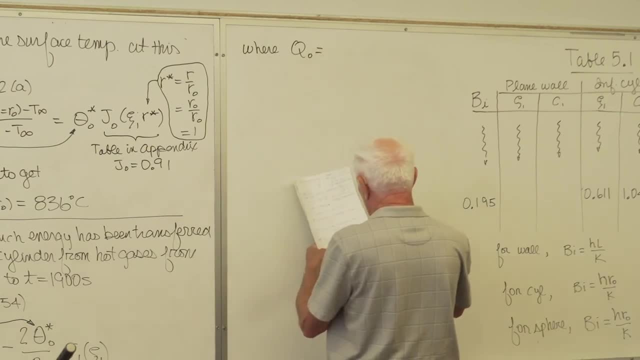 So my Q naught is rho C 0.4.. So my Q naught is rho C 0.4.. So my Q naught is rho C 0.4.. VV- t initial minus t infinity. 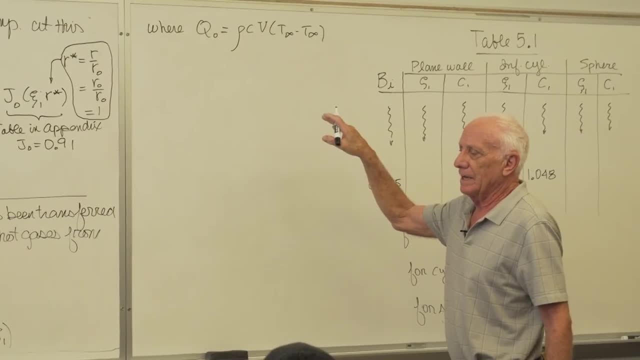 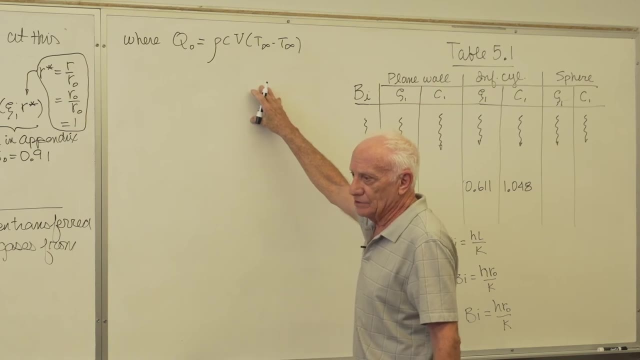 That's like mass times, C times the temperature change. That's like stored energy. So what Q naught is: it's like the amount of stored energy in the body at the start of the process relative to the t infinity outside temperature. relative to the outside temperature. 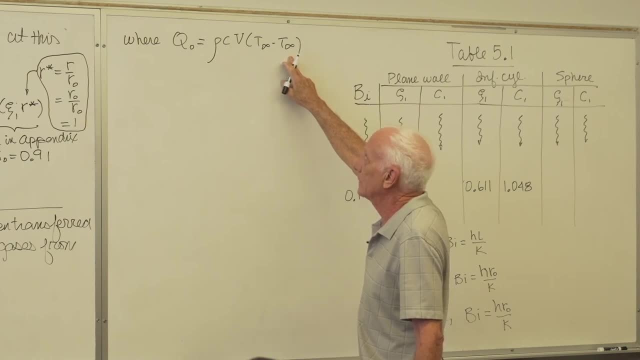 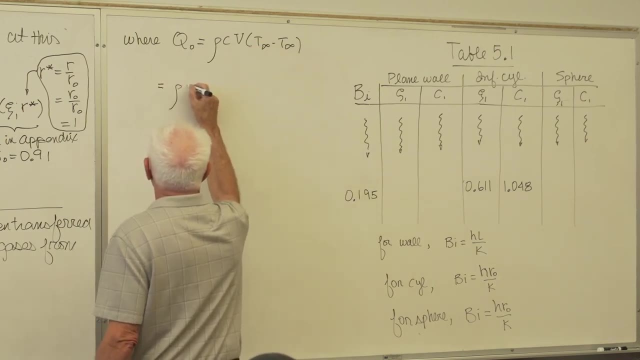 How much energy is stored relative to the outside temperature of the body. Now, what's the volume? Okay, this is a long cylinder, rho Cv. circumference, pi times d times the length, t initial minus t, infinity. Do I know the length? 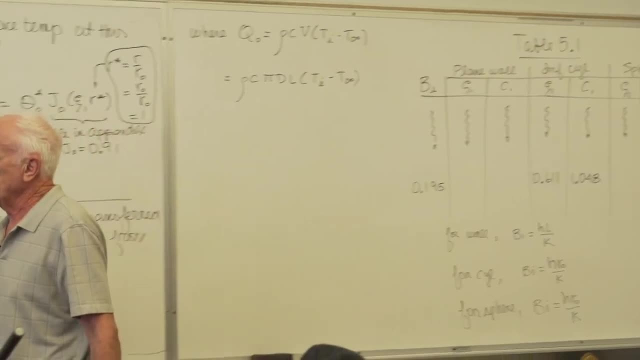 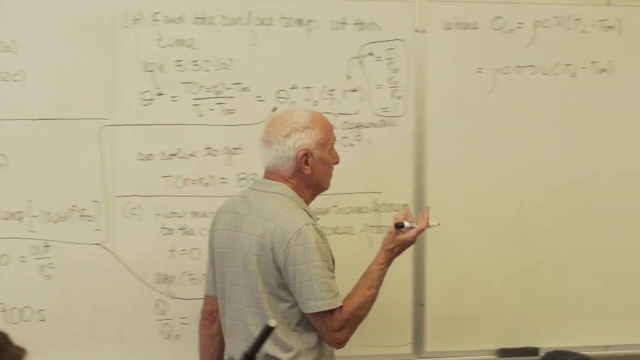 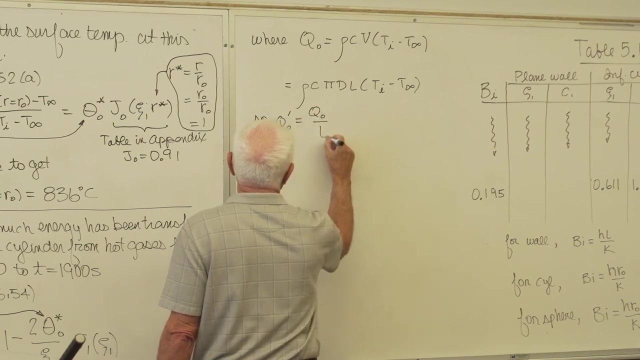 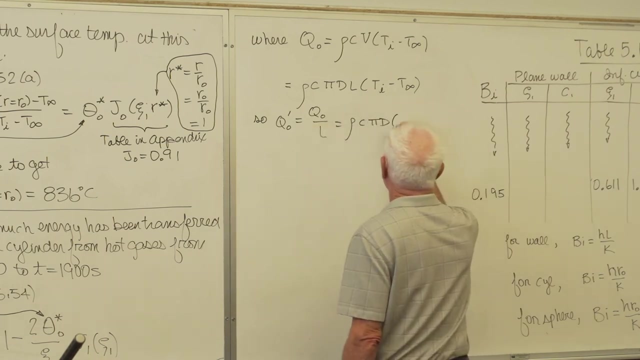 No, the problem set a very long cylinder. I don't know L. You know the game we play. If you don't know L, you divide by L, You make it prime quantity. The L cancels out. Now you've got to put primes on everything. 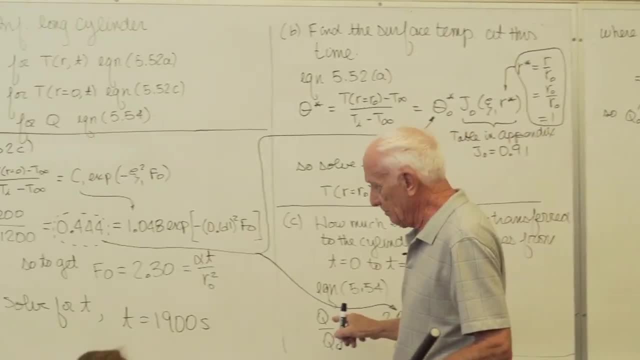 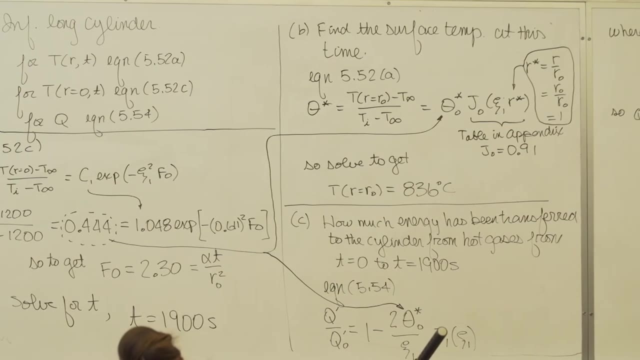 I'm not going to find Q in joules, No, I want to find Q prime which is joules per meter, and this is Q naught prime. So there's the right equation. I'm going to use Q prime divided by Q naught prime. 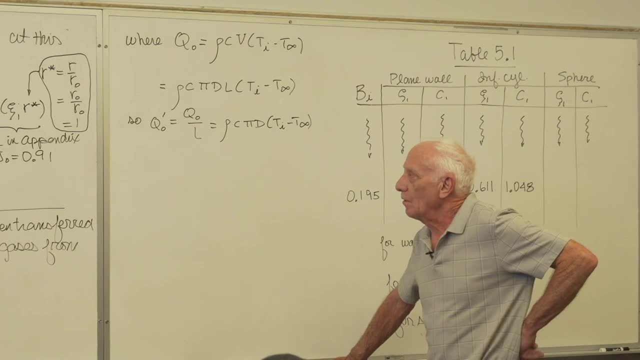 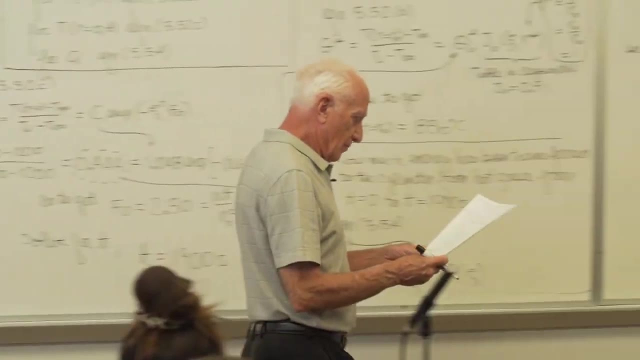 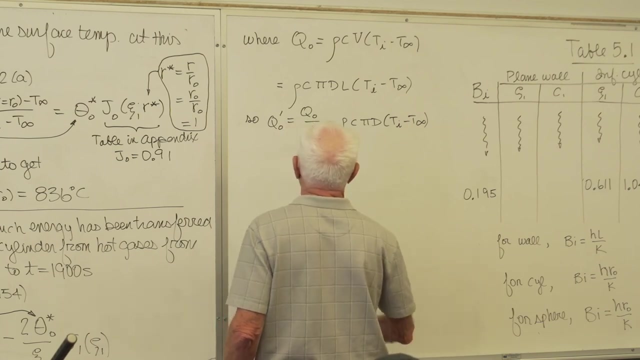 equal 1 minus dot, dot, dot. Oh, and then did I get that number? Let's see if I got that number. Yeah, I did 2.4 times 10 to the ninth joules per meter. Then I put that: 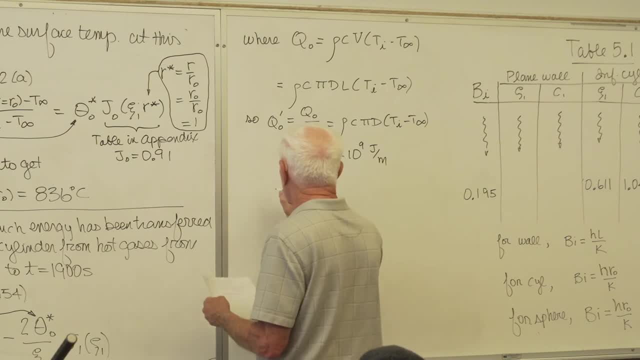 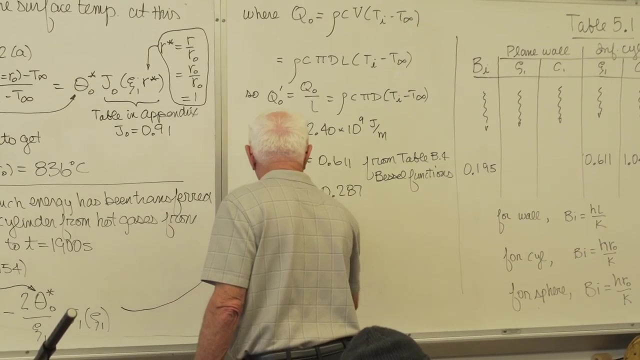 Now I need this guy. So at x equal 0.611 from table B4, Bessel functions J1,, J2,, J3,, J4,, J5,, J6, and J7.. Put that in there. 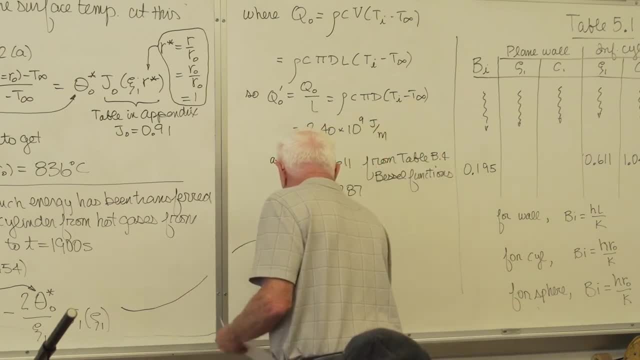 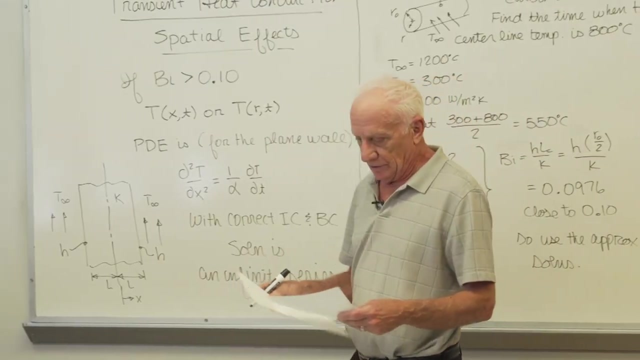 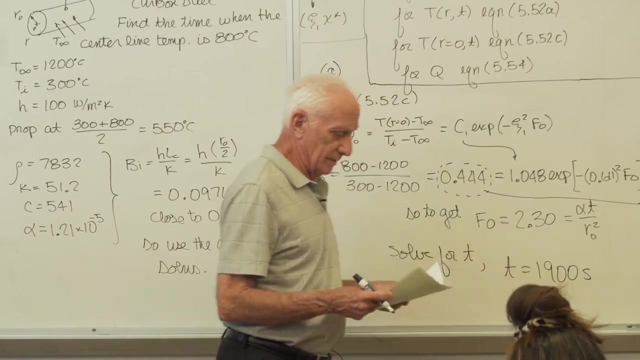 Solve for Q, and there is the amount of energy that's been transferred to the cylinder from the hot gases In the time interval from time 0 to 1,900 seconds. So what I've done there, then I've used all three of. 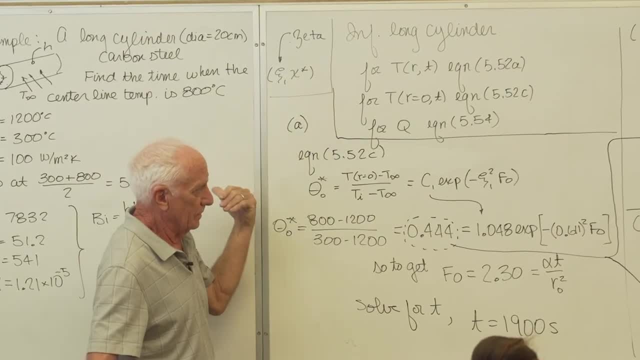 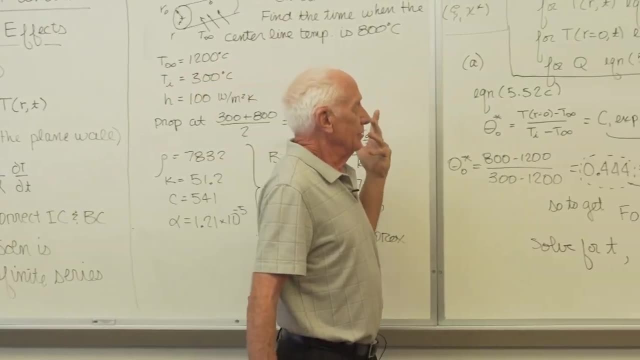 these equations in this example, for this one problem, It doesn't matter if it's a plane wall, a long cylinder, R-sphere. you do the same three things. You can find the temperature anywhere. You can find the temperature at the center line or the center. 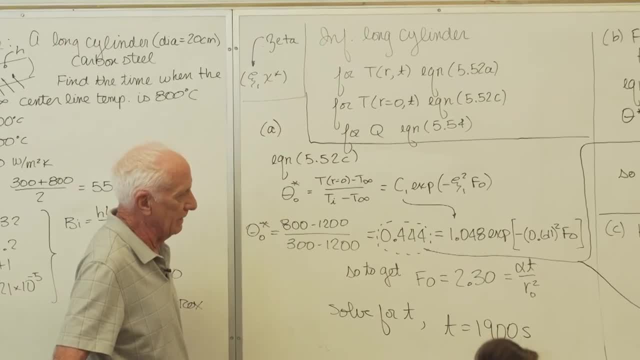 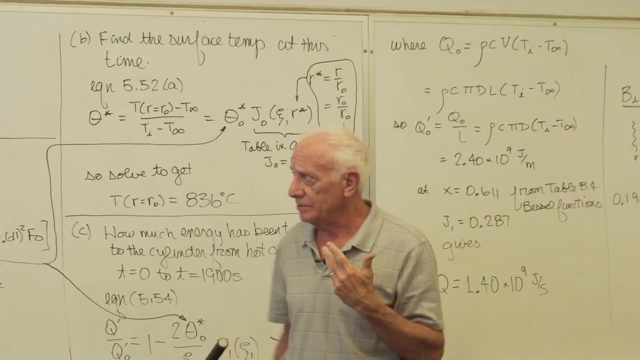 and you can find the amount of Q that's occurred between time equals 0 and time t. Why does our book only give these three geometries? Because they're very popular geometries. They occur quite often. For instance, maybe you want to heat. 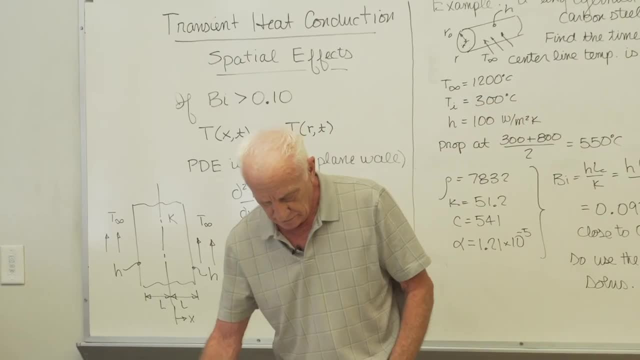 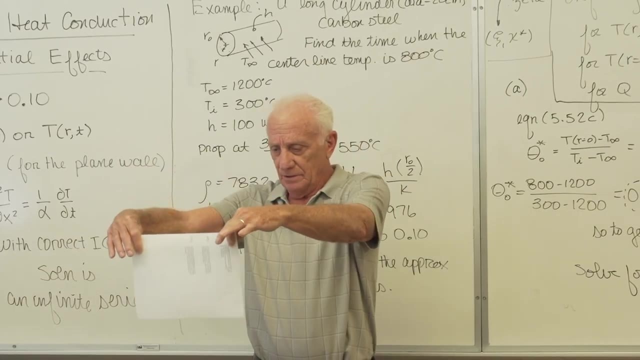 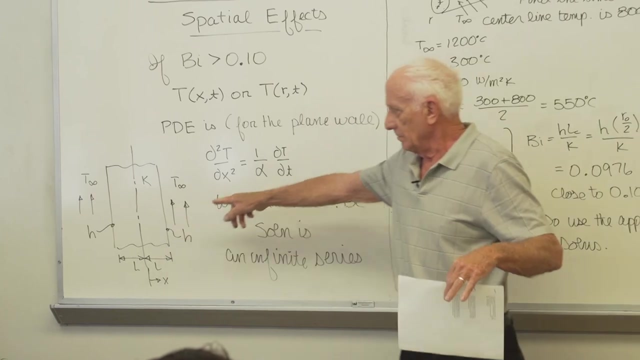 treat some kind of a metal plate, and so you've got the metal plate hanging from hangers. Here's a big metal plate. You put this guy in a furnace- hot gases on both sides. There's a picture right there. This is used for heat treatment of plates. 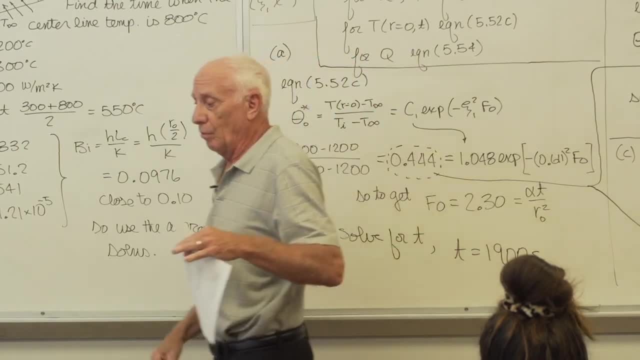 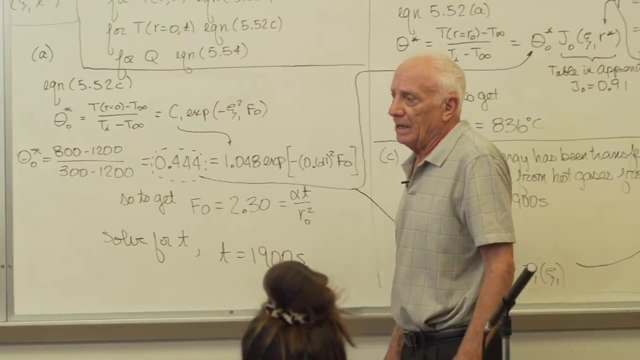 Along cylinder. a wire is a long cylinder. You can heat treat wire. A big spool of wire hundreds of feet long, By how big diameter, I don't know. one inch, half an inch, quarter inch, That's a long cylinder, believe me. 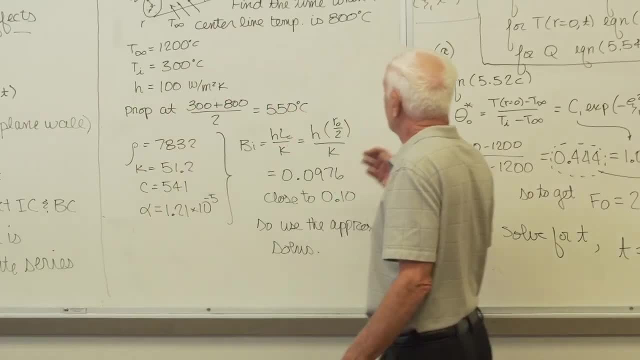 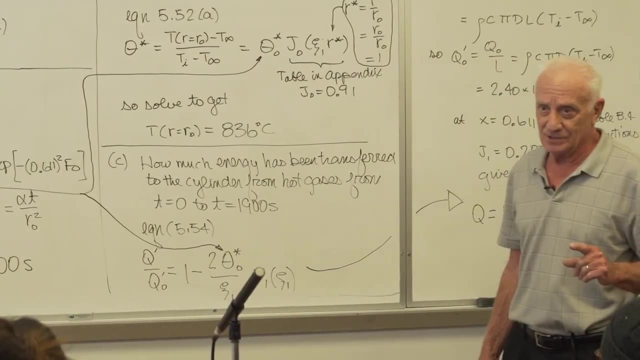 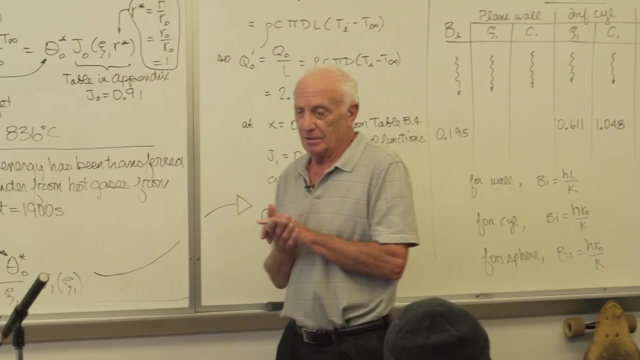 It's used for heat treating wires. How about spheres? Ball bearings have to be hardened on the outside surface, only On the outside surface hardened. How long should the ball bearing be in heat treatment, just in order to make the outside hardened? That's here it is. 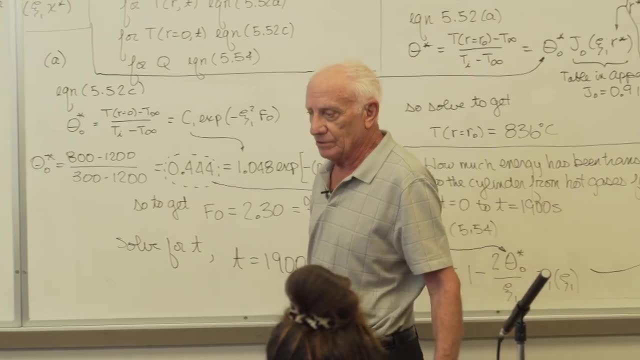 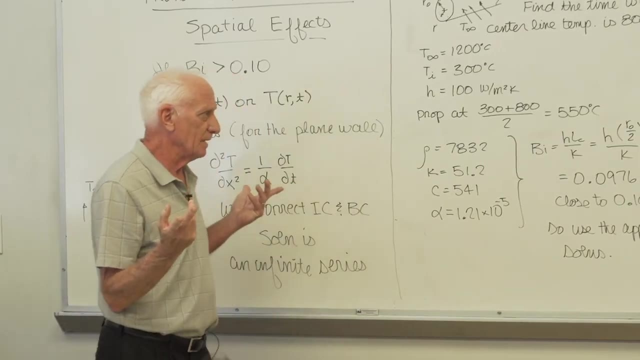 Where's the time in there? We just did a one with time. Yeah, these are common geometries used in engineering for heat treatment, for instance. besides other reasons, of course, But mainly a lot of it's on the heat treatment side.